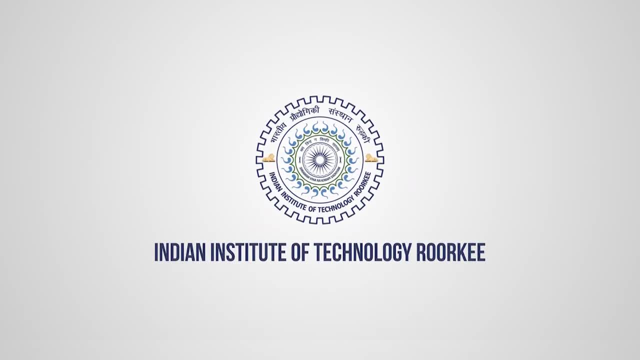 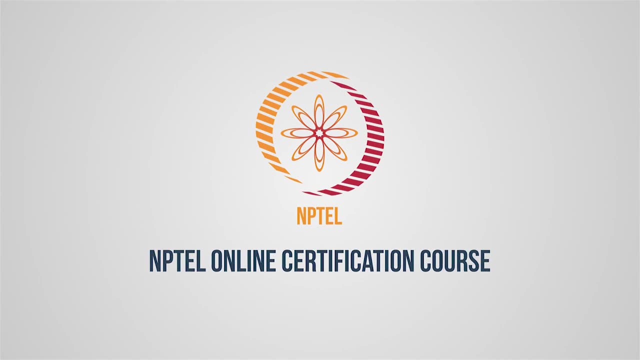 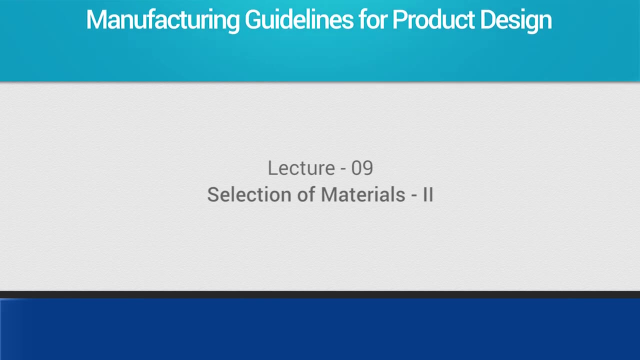 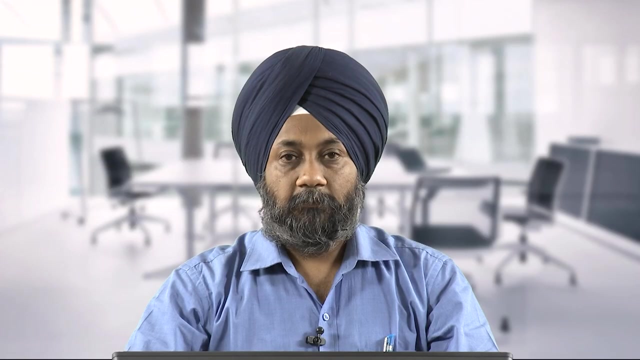 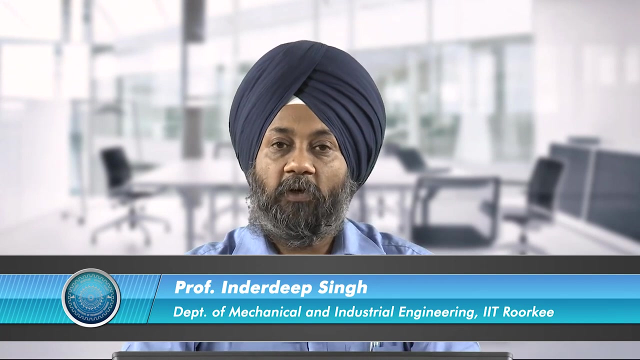 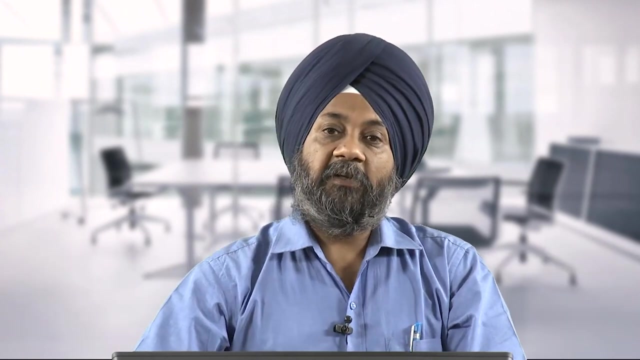 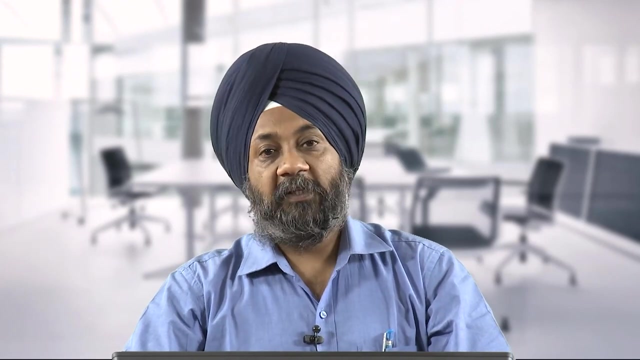 Namaskar friends, welcome to session 9 of our course on manufacturing guidelines for product design. We are currently in the second week of our discussion and our target in week 2 are the engineering materials. We want to have a basic idea or a broad picture of the various types. 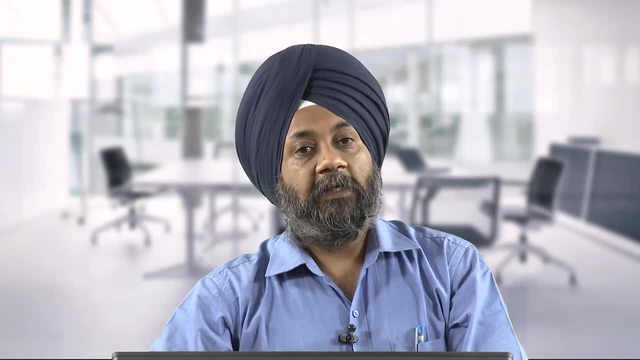 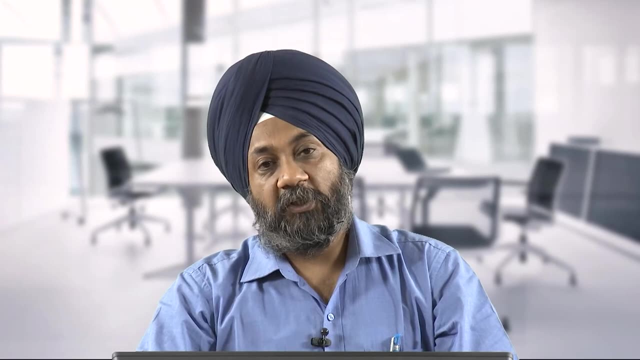 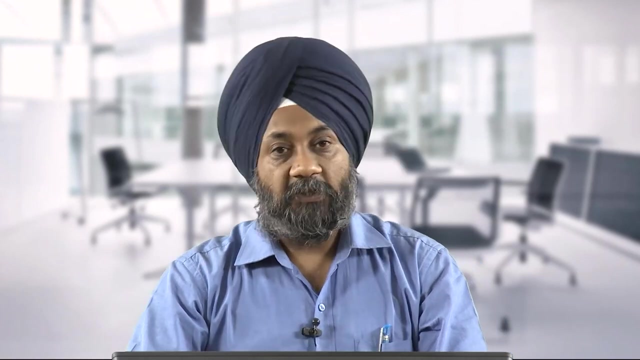 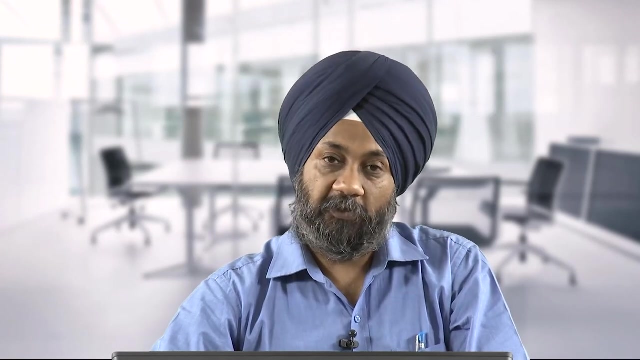 of engineering materials that can be used for making different types of products. We have already seen the categorization or the classification of the engineering materials. We have seen that there can be broadly, metals and alloys, polymers, ceramics, composites, as well as certain advanced materials such as nano materials or shape memory alloys. 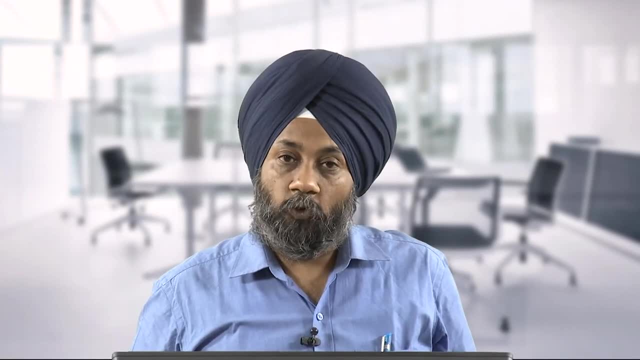 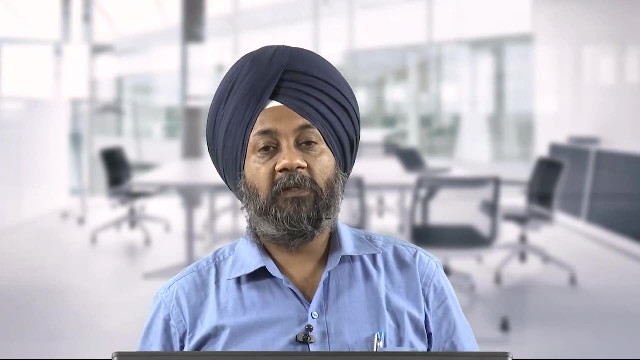 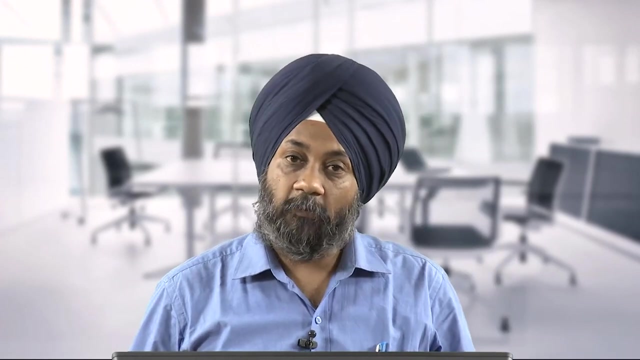 So the classification is well known to all of you by now. We are now trying to understand that, because of the wide variety of engineering materials, with having different characteristic features in terms of their physical properties, chemical properties, manufacturing properties- Depending upon these properties, we have to select the best material. So we have a problem. 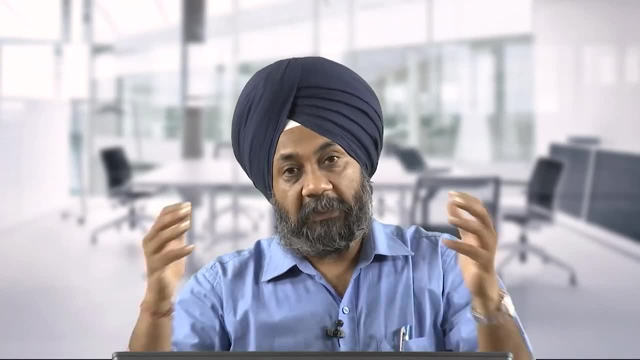 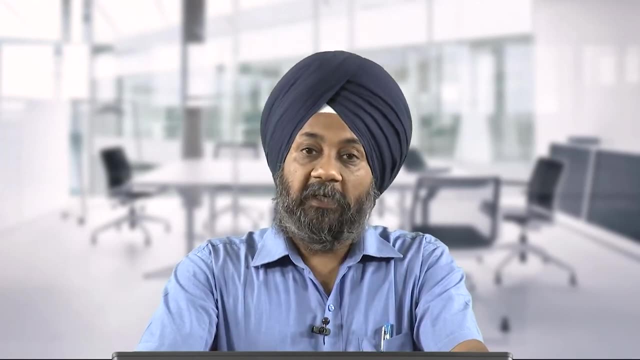 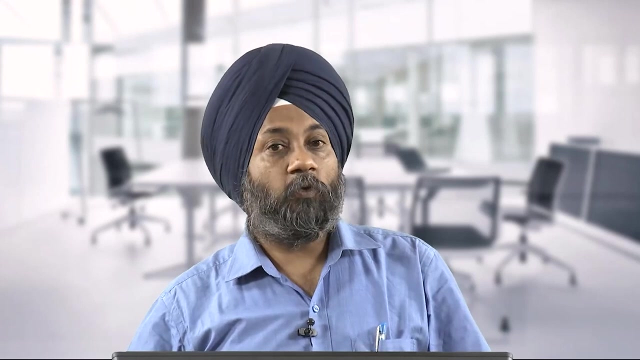 of plenty at hand. There are so many materials having so diverse properties, how to select that, which one material or which one of them is going to suit or is going to help us achieve our intended function for our product, Or is going to help us to satisfy the needs and requirements for which the product is? 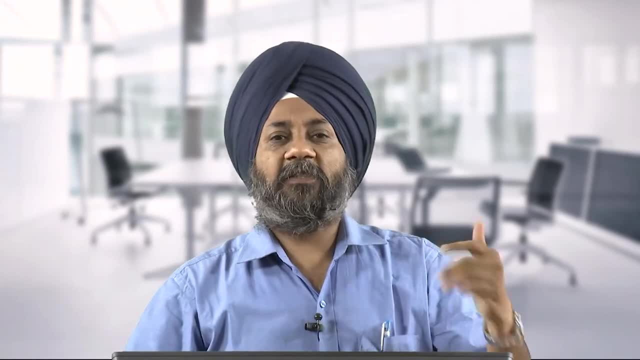 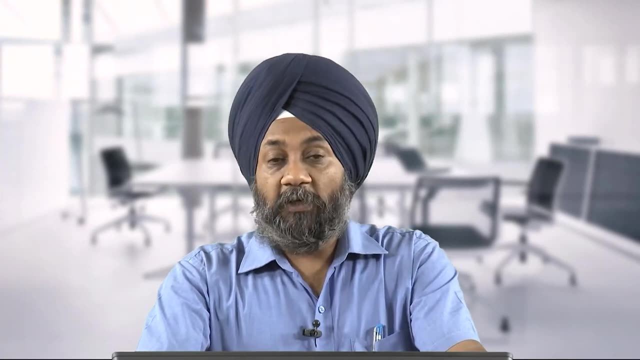 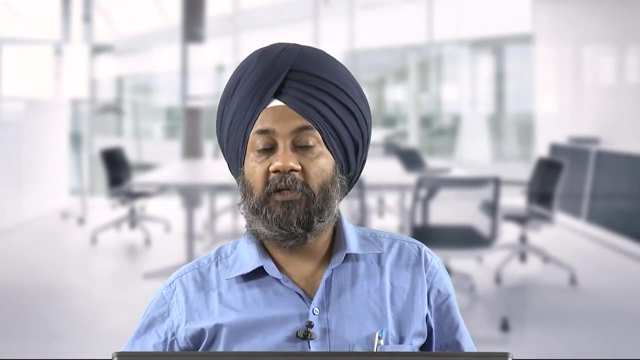 being developed. We have taken very vague examples like metallic bristles for brushing of tooth or brushing of teeth. So we cannot use metallic bristles for brushing of our teeth because the bristles have to be light on our gums, otherwise the gums will start to bleed. 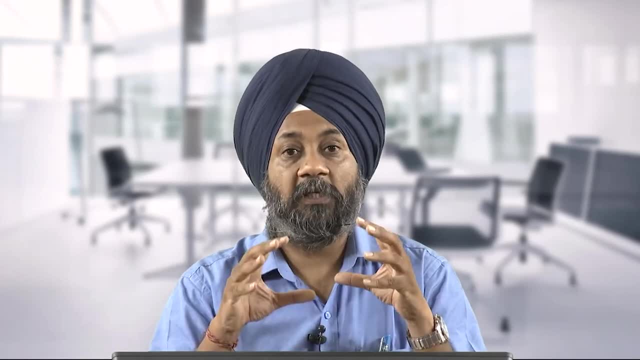 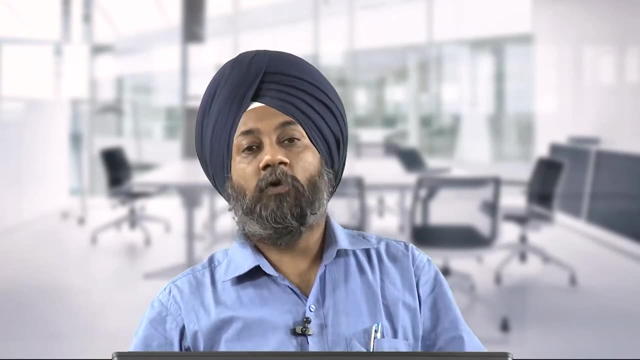 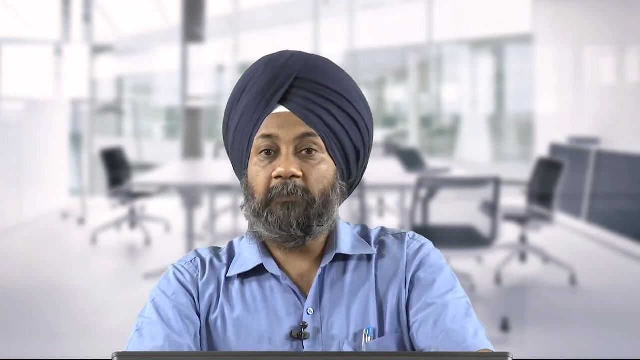 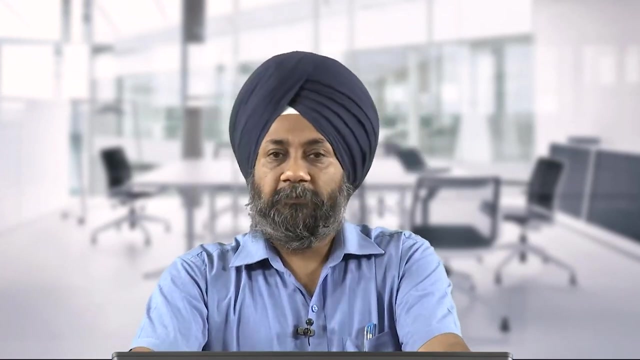 So each of a engineering material for a specific application depends upon the service or the needs and requirements that the product is going to fulfill for the customer, And for that the engineering materials play a very important role. Many times we have to see: there are material available, there are fabrics available which have very long life, But we 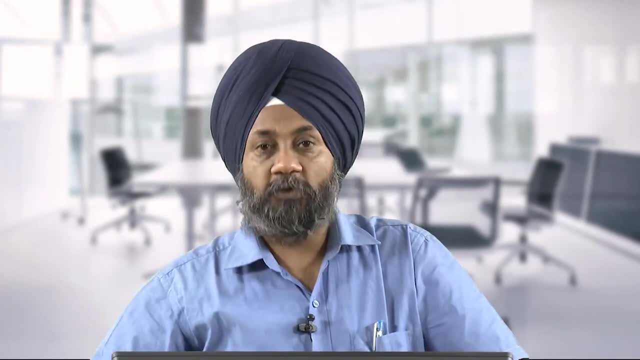 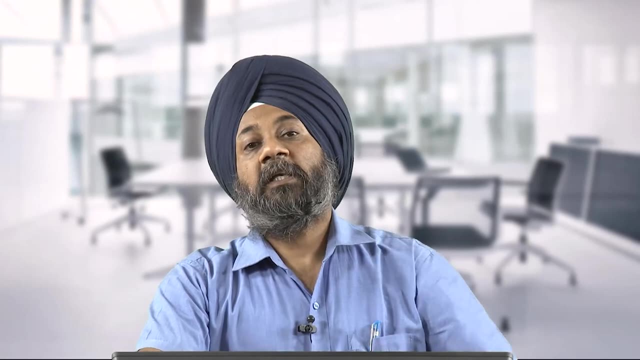 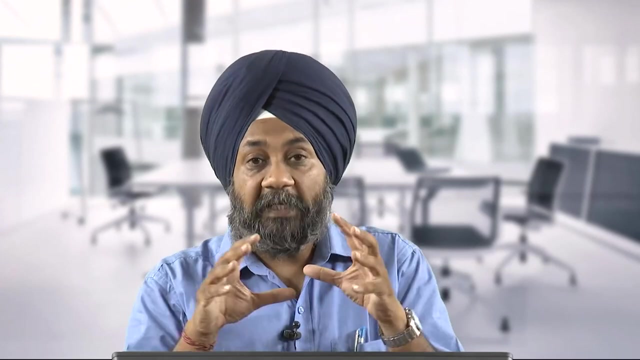 cannot select that fabric for making up of the socks. So we have to select the fabric for making up of the socks, Because we must replace our socks every 6 months or every 3 months, because they sometimes get worn out, sometimes they start smelling bad. So, depending upon the intended function, 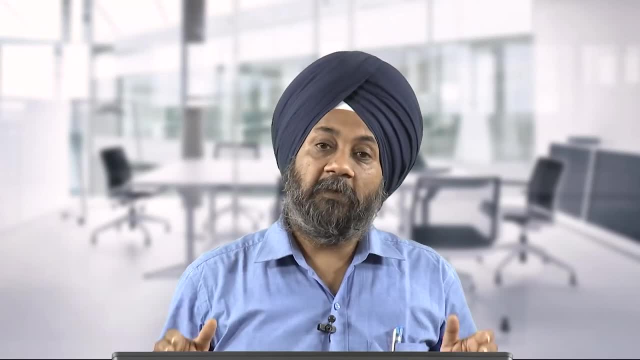 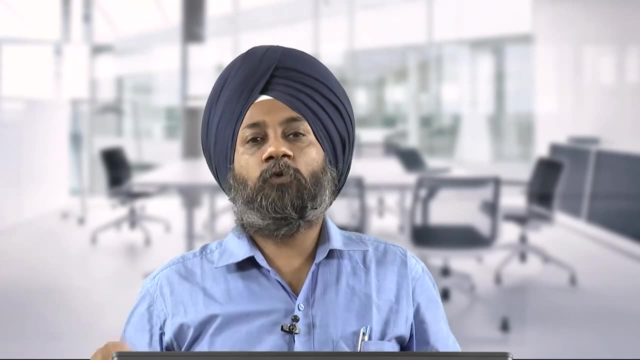 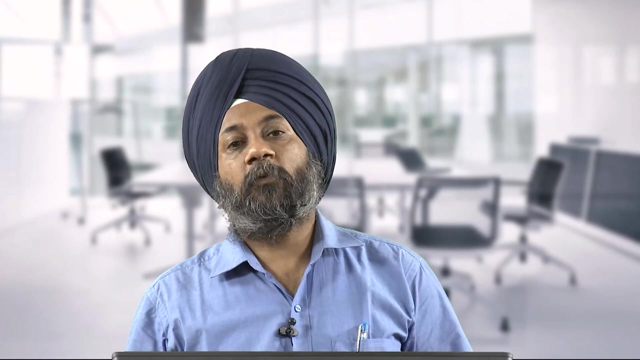 we have to select the engineering material. If suppose somebody develops a material for the bristles of the toothbrush that once as a child you buy a toothbrush and then you need not replace that throughout your life. So we have to be advisable, depending upon the hygiene and the other conditions we have. 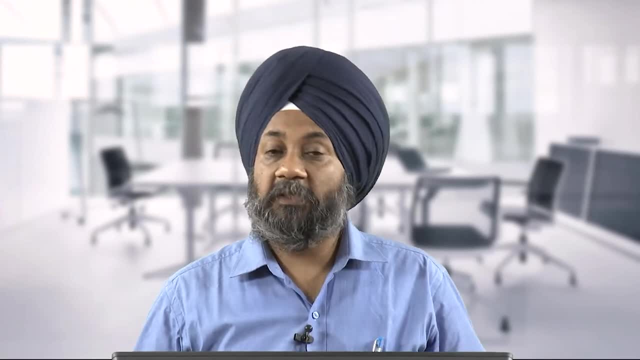 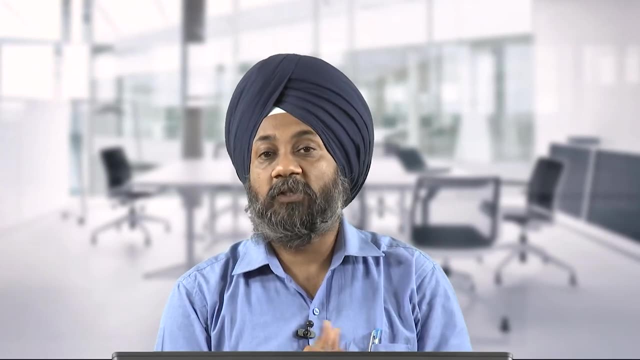 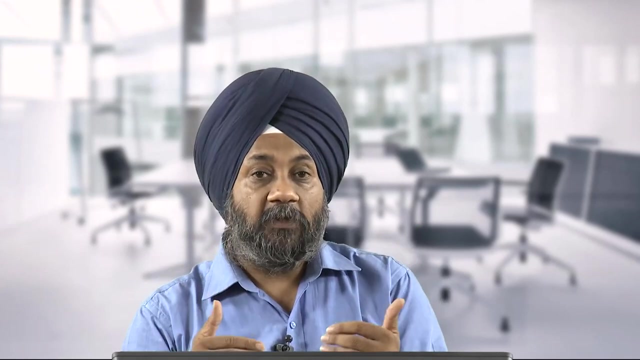 to see that. what are the material properties that we are required to satisfy the intended function? So there are number of other parameters that govern our selection of the engineering material, And today we are trying to further see that, sometimes using concepts of mathematics, we can try to come up with solutions or try to solve the problem. 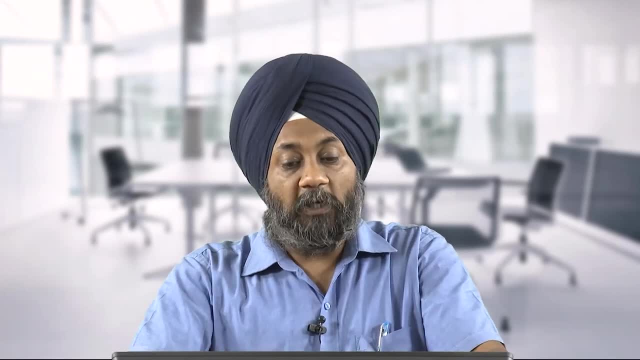 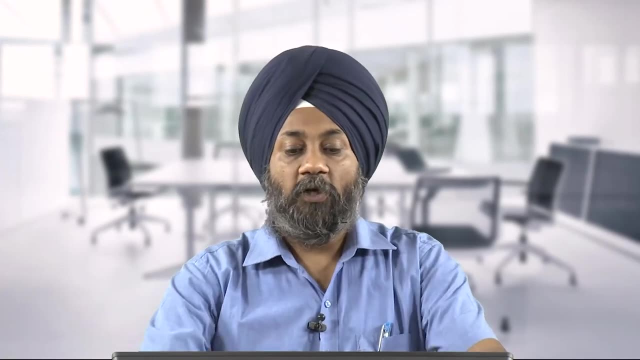 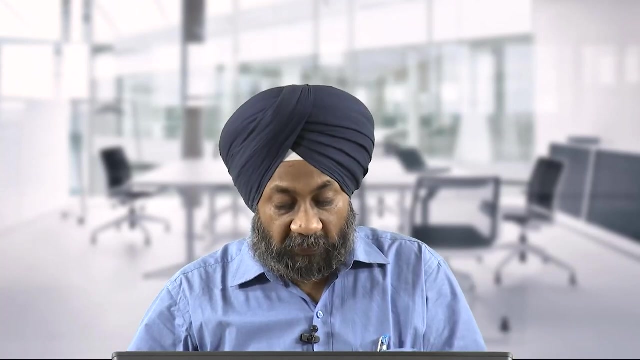 So when the manufacturing guidelines for product design we are going to see in today's session, with emphasis on selection of materials. that is the second part. In first part we have seen the basic aspects. today we are going to see the applied aspects. Now let us see. 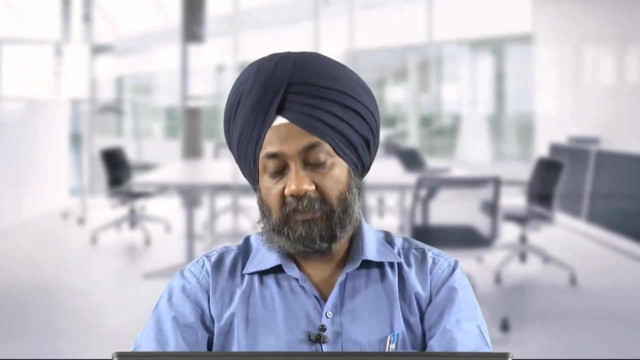 that. what are the various factors that influence the material selection? In our previous session we have already seen that. what are the material properties deceived? So we have already discussed about partial State of matter. the two술 and matter We have to aren't gotten to that. 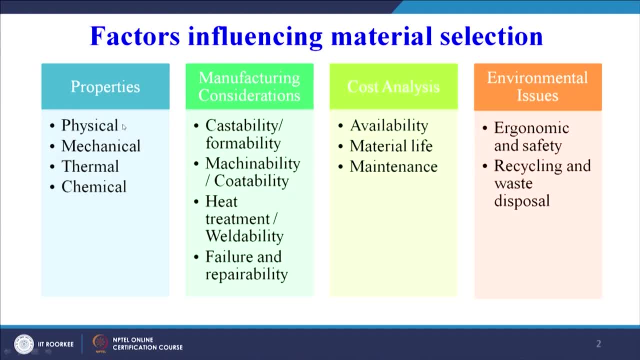 Thank you very much, Kenwish. Here we will conclude with an end of this session, our first session for today's. What are the various physical properties we have already seen for the different types of materials? mechanical properties, thermal properties, chemical properties. so the properties. 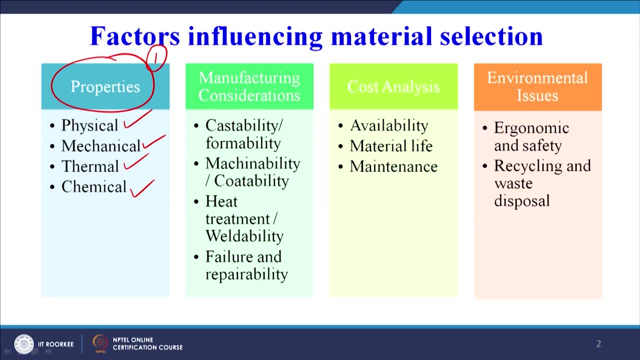 of the engineering material is the most important criteria which has to be taken into account. Then the manufacturing considerations are also very, very important. we may definitely be able to find a material here, and suppose we find that the composite material is satisfying our requirement. all the requirements that are there in the product design. 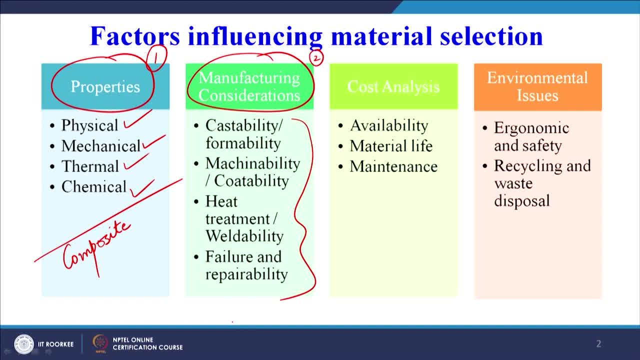 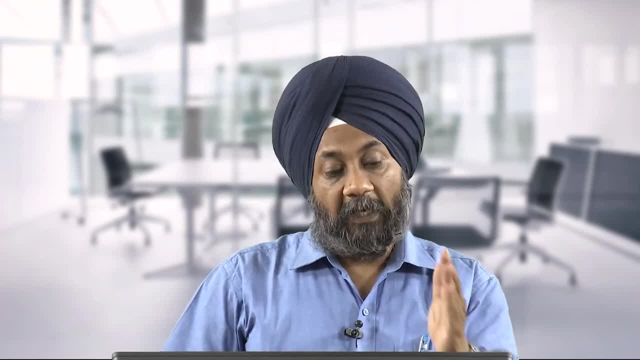 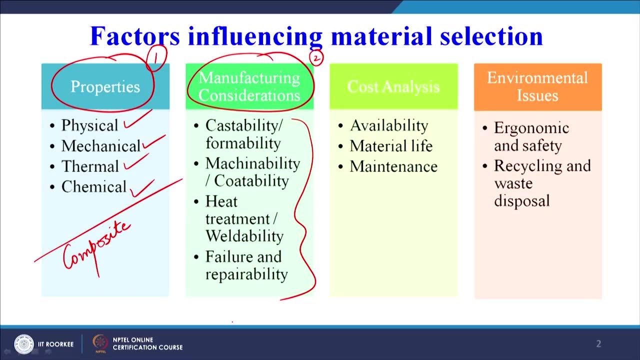 But maybe then we are not able to find any manufacturing process which can make the composite as per the required product design. Therefore, alongside the properties of the engineering material, we must also consider the manufacturing considerations. We must understand the castability, formability, machinability, coatability, then failure and 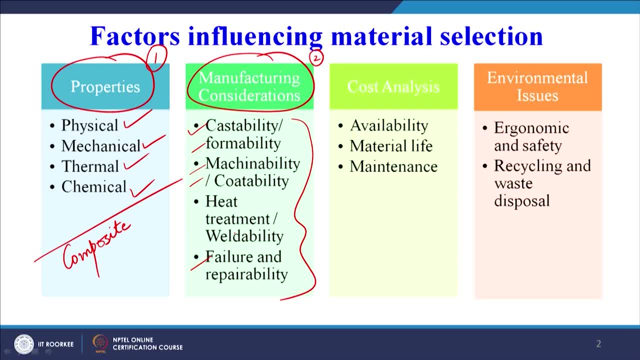 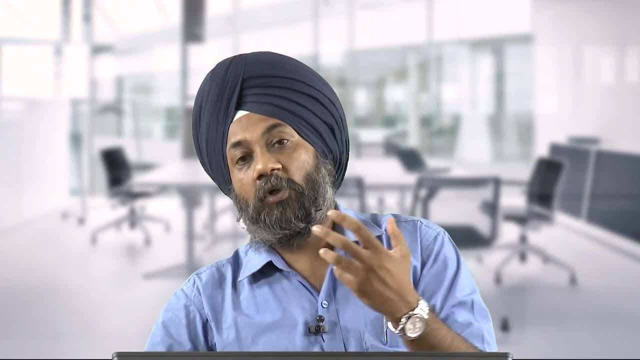 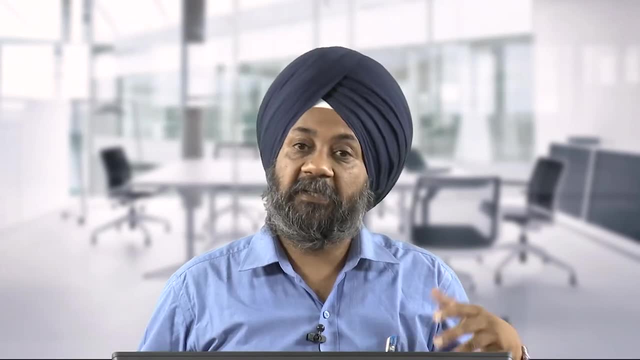 repair also sometimes play a very important role. For example, we have designed a product, we have installed the product or engineering structure and it has got damaged because of certain unwanted circumstances or certain unwanted events or certain accidental events. If we do not have a repair strategy, 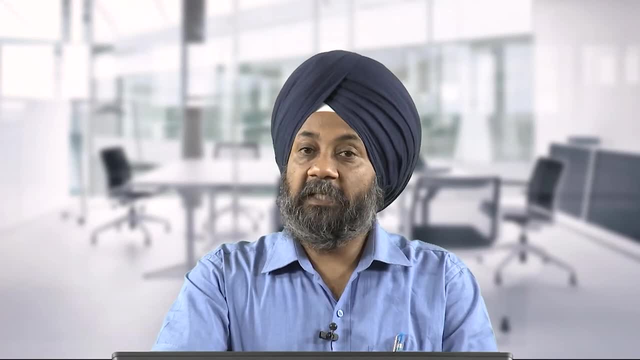 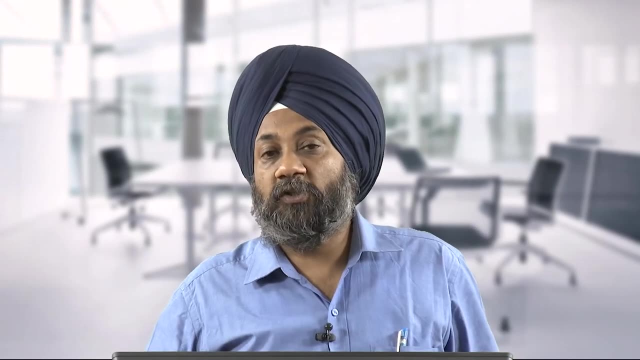 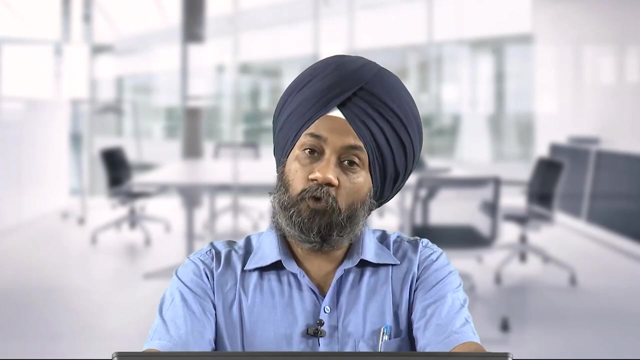 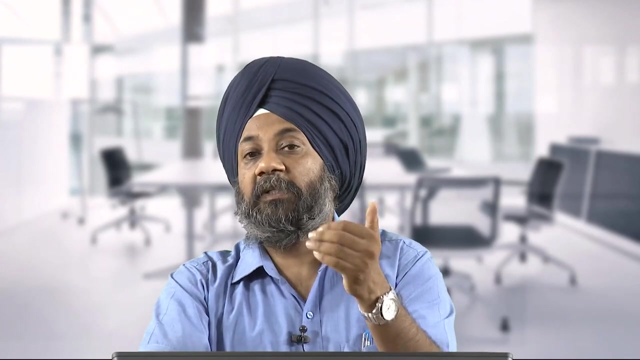 In place, definitely the product will not be. the product will not be able to provide the intended function for which it has been designed or installed. So therefore the repair maintenance also has to be identified in the very beginning only, and then, for repair and maintenance, we have to select our engineering materials in such 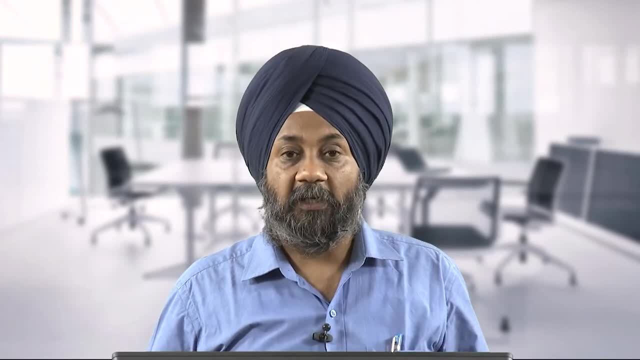 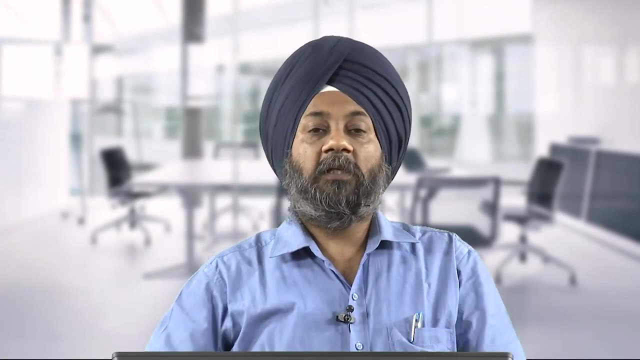 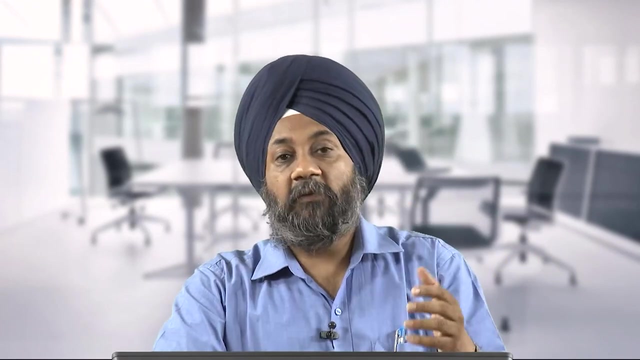 a way that the repair and maintenance is easier. So So, first thing are the properties, second is the whether we will be able to manufacture the product with the selected material economically, whether it is feasible. can we get that shape? can we get that size? 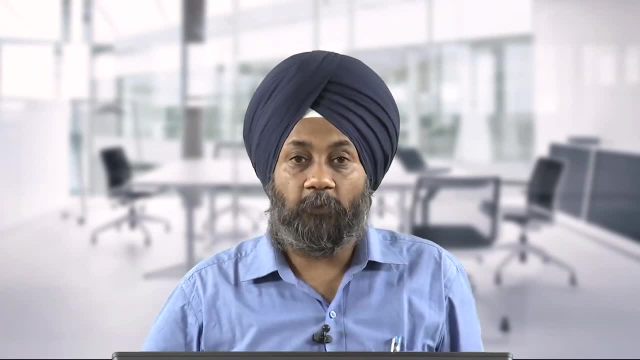 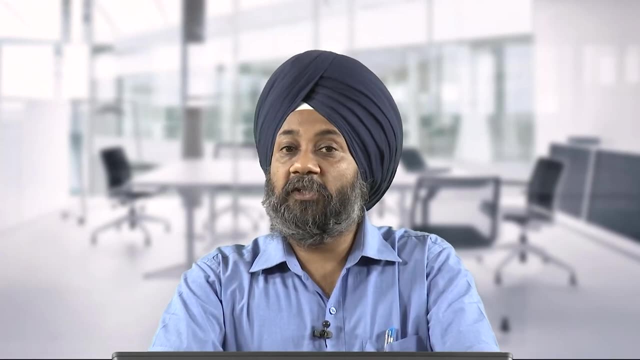 So that? can we get that complexity that is there in the product design using any one of the standard manufacturing processes, or we need to modify our manufacturing processes to suit the needs and requirements of the product design. All those things we have to consider, Okay. 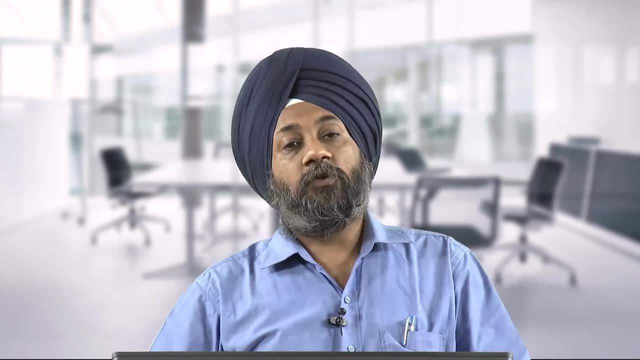 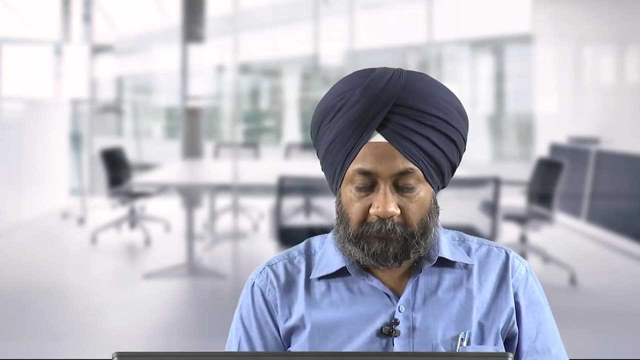 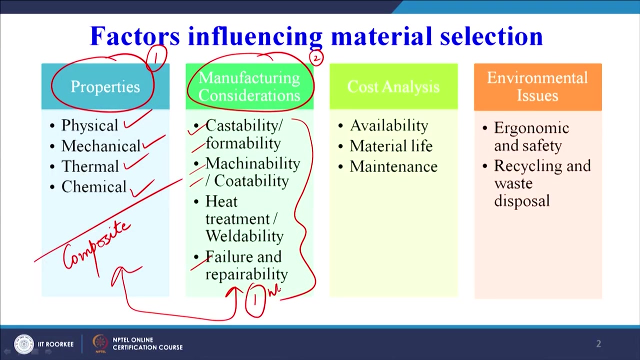 All those things have to be considered during our process of selection. Then the other parts, the allied parts, are also equally important. These 2 things we are focusing currently- the manufacturing considerations in the first week. we have focused and we have tried to see the process capabilities, engineering materials. 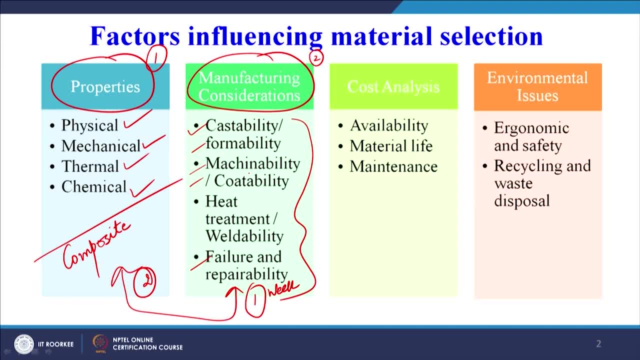 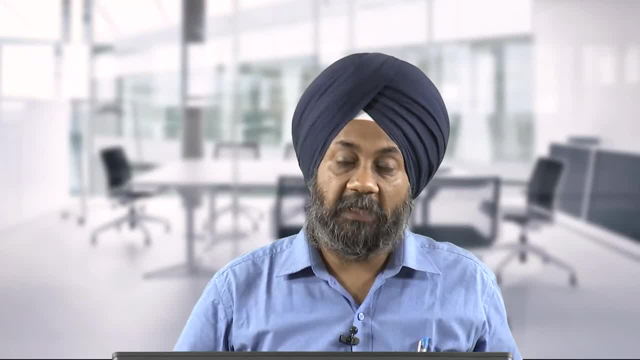 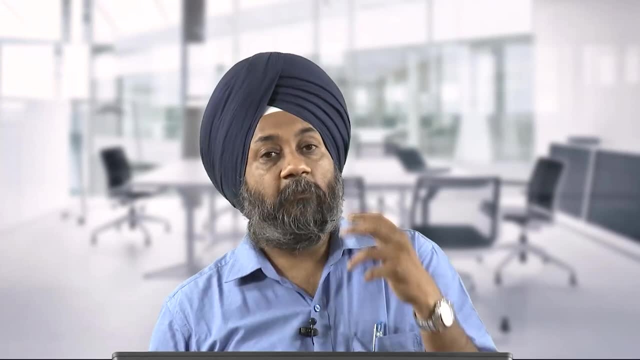 we are focusing in week 2 and further. all these processes, whatever is written- casting machining, Sometimes injection molding, compression molding, specially for plastic parts- we are going to cover in our subsequent sessions. So our primary focus is on these 2 aspects, the manufacturing aspects as well as the material. 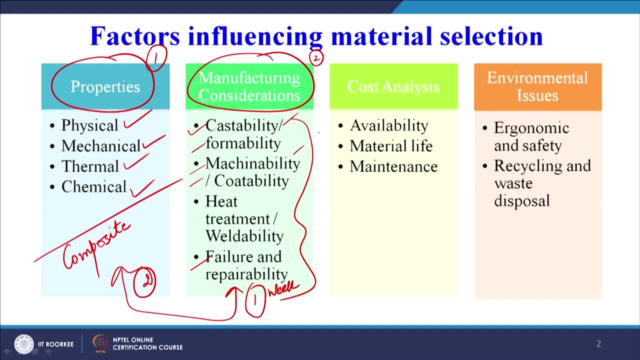 aspects. Then, finally, we also have to consider the cost, because ultimately we have to make a product in the most economical manner. in cost analysis, we have to see the availability of the materials. We have to see the life of the material. just now I have given an example that if just now 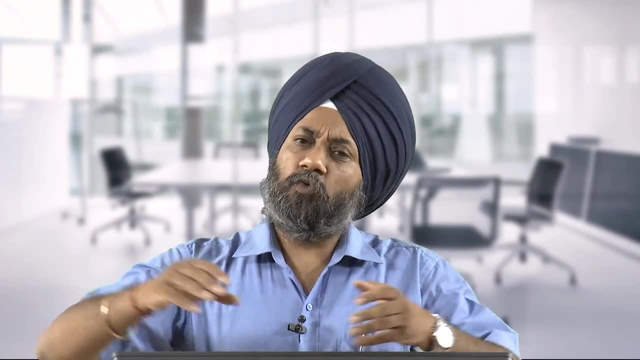 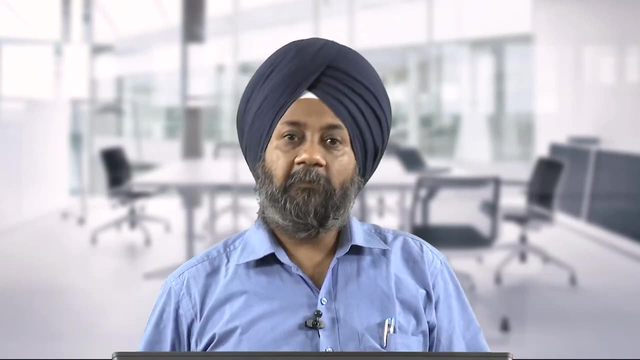 I have told you that if the material life is too long and we are using it for making a shirt, I may not like to wear the same shirt throughout my life. I may like to change the shirt every year, or maybe 1 and a half years, or 2 years, 2 and. 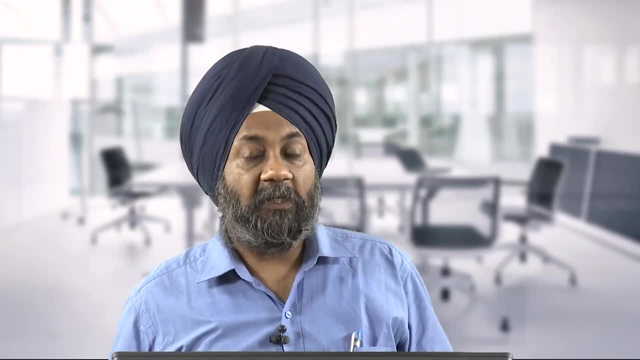 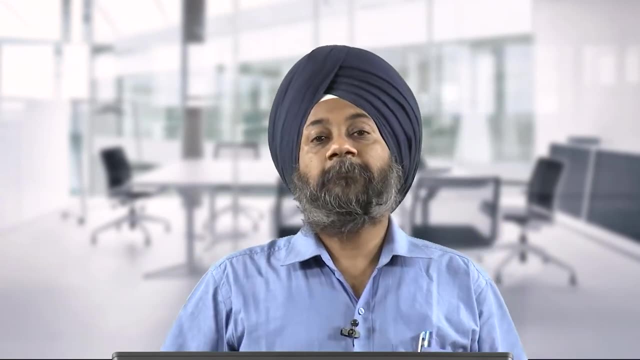 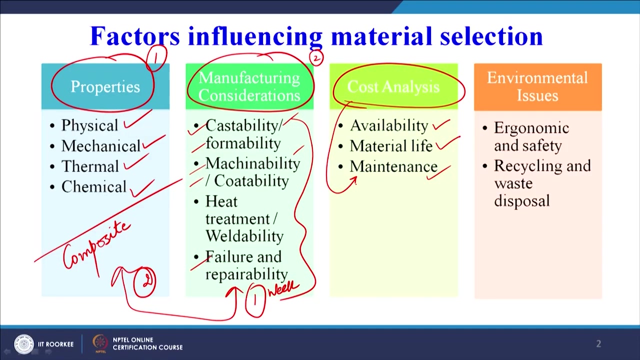 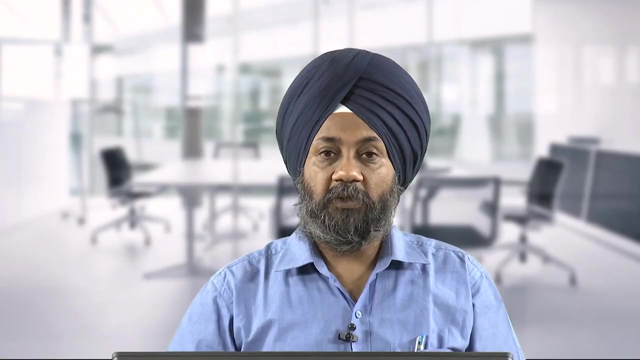 a half years. So the material life is also very, very important. then the maintenance of the material that we have already seen That the maintenance must be easy. So the cost analysis point of view is important because the maintenance will also if we require frequent maintenance, for example we have again- I am taking an example of underwater application- 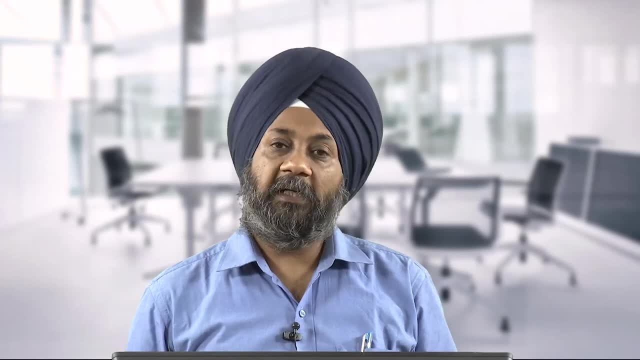 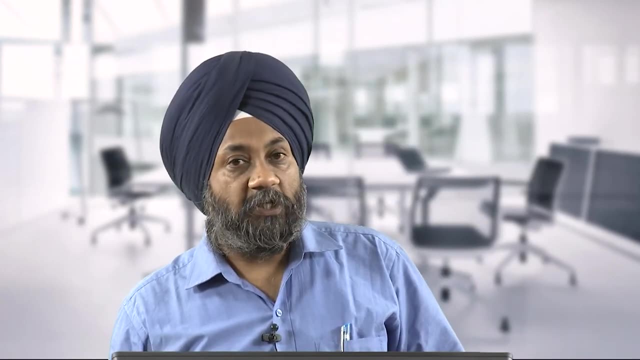 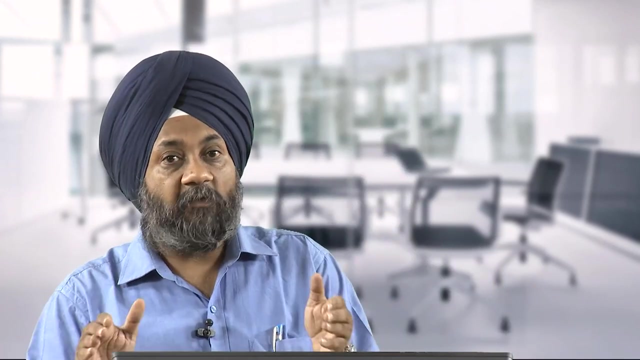 So we have underwater application, some material we have selected for that structure. Suppose, every 6 months we have to do the painting, so the maintenance becomes a costly affair, Whereas If we select a material or engineering material which requires no maintenance, however, it must be costly in the beginning. 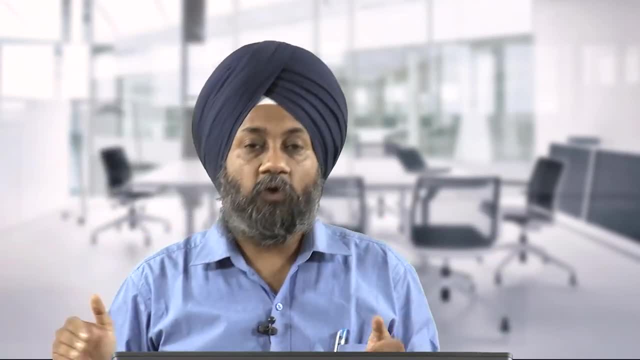 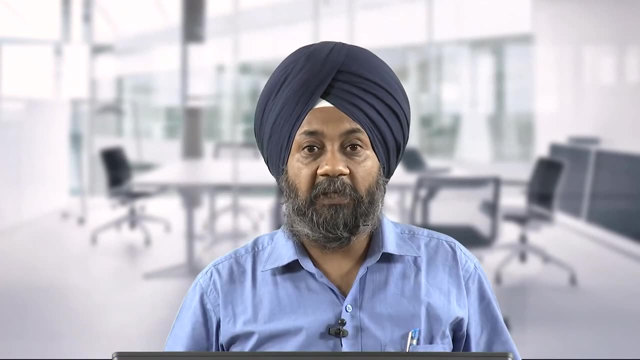 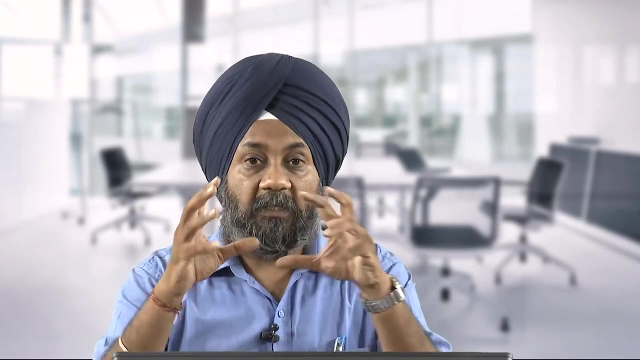 But over the life cycle the cost becomes less because after every 6 months we need not stop the operations and do the painting of the structure. So why not to select that material which requires no maintenance but initially maybe it may be slightly costly. So that kind of trade off has to be done when we are selecting a engineering material for. 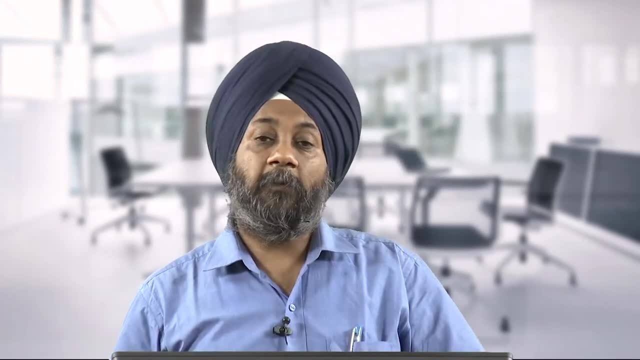 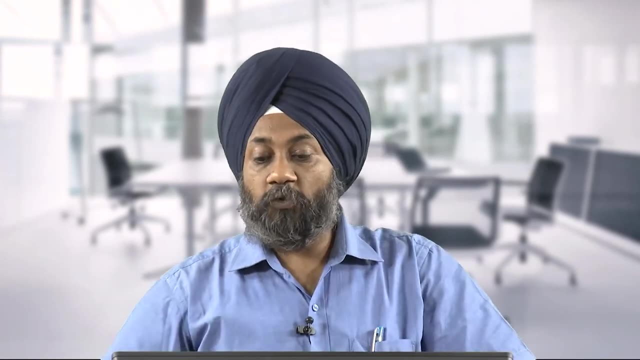 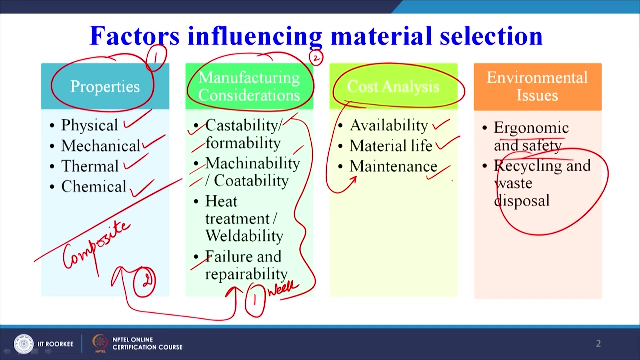 a particular product and that will help the company to save lot of money. Then, finally, we come to the environmental issues. So we have to see the ergonomics and the safety aspects. recycling and waste disposal very, very important. As we record these sessions, maybe in the 2nd week or 3rd week of June, lot of emphasis is 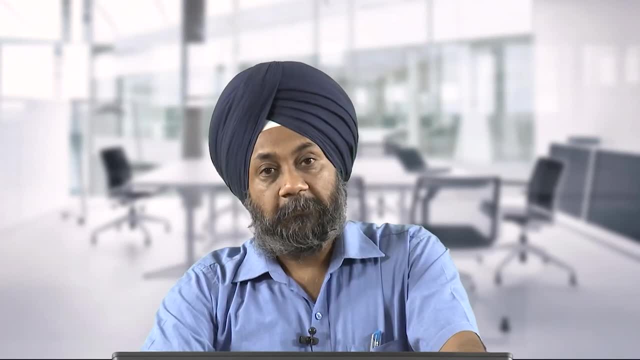 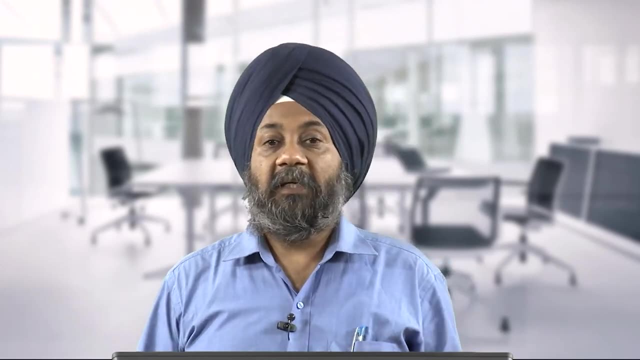 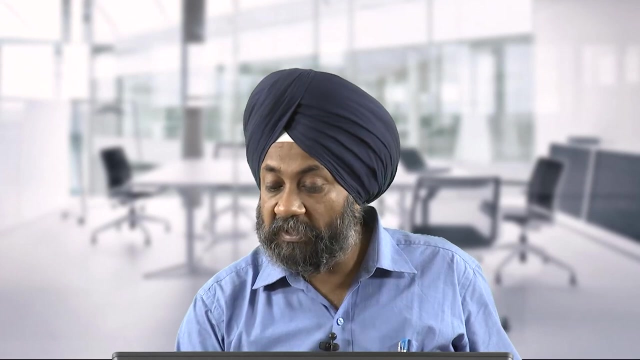 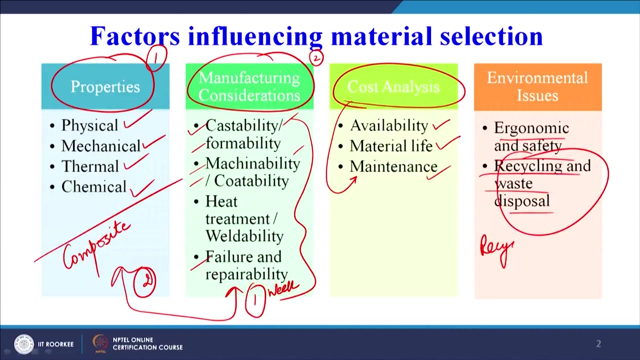 there on minimizing the plastic waste, Different organizations, different rules are being passed. every day in the newspaper we see that the use of plastic has been banned or use of plastic carry bags has been banned. Therefore, there is a need to select a material for our product which can be recycled, which 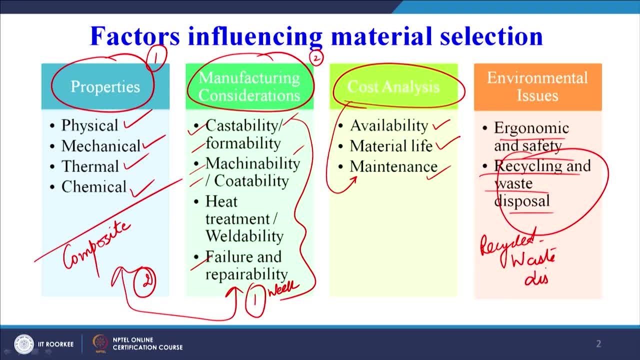 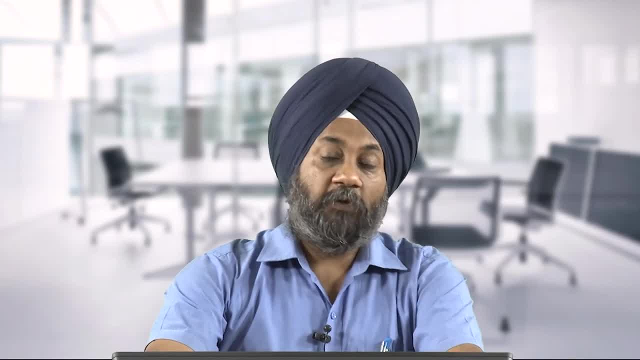 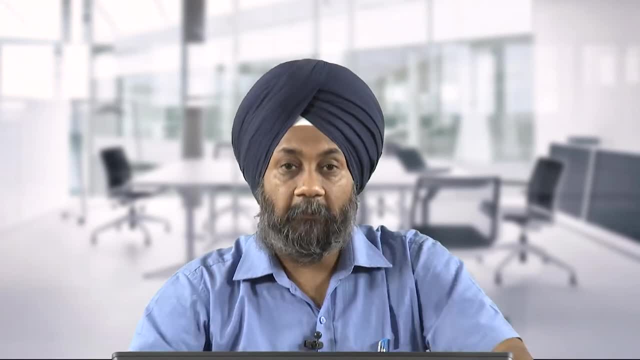 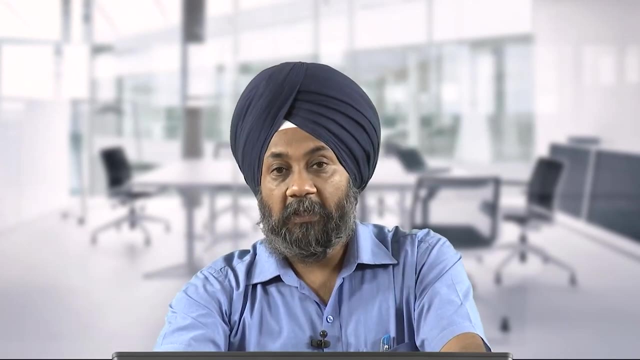 can be easily disposed into the environment without causing any harmful emissions. Okay, So the selection of engineering material for a particular product design will basically depend on these 4 important parameters, that is, the properties of the engineering material, the manufacturability of the engineering material, the cost of the engineering material, as well. 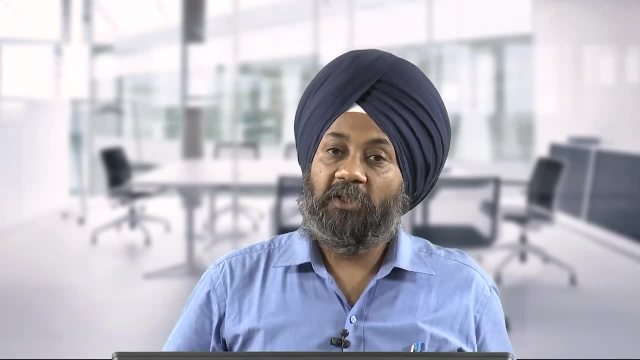 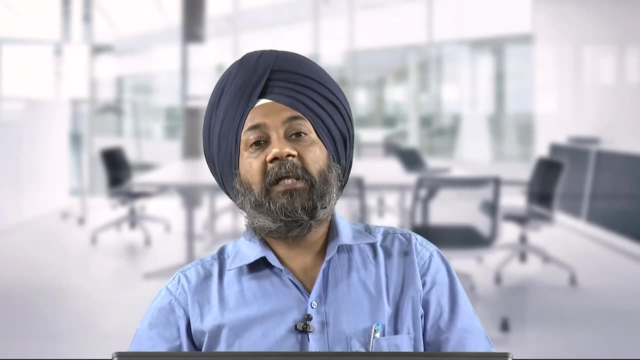 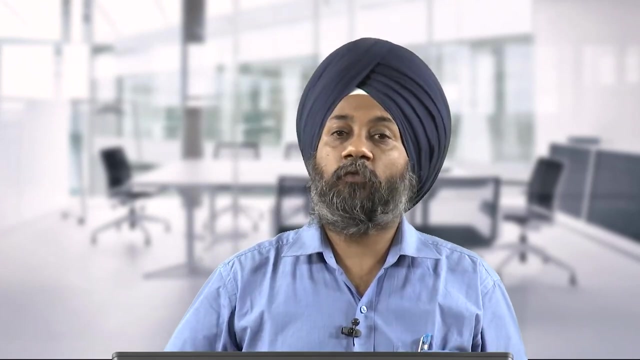 as the end of life of the engineering material or end of life issues of the engineering material, That whether it can be recycled, Whether it can be easily disposed of into the environment without causing any harm to the environment. So these 4 factors are the broad factors that have to be taken into account. 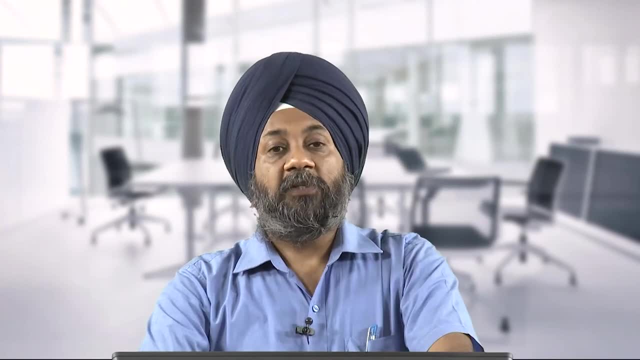 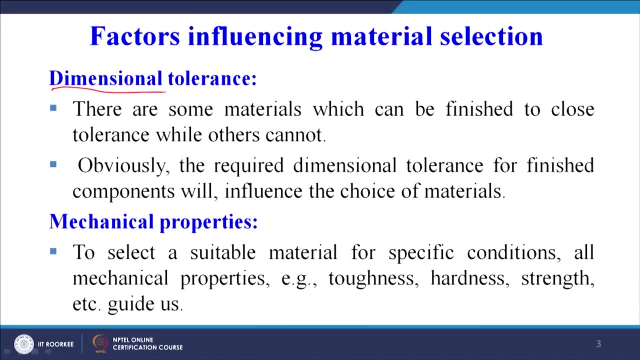 I think I have explained in detail. now, quickly we will see each one of them So factors influencing the material selection. so from properties we have not touched down the dimensional tolerance. So there are some materials which can be finished to close tolerance while others cannot. 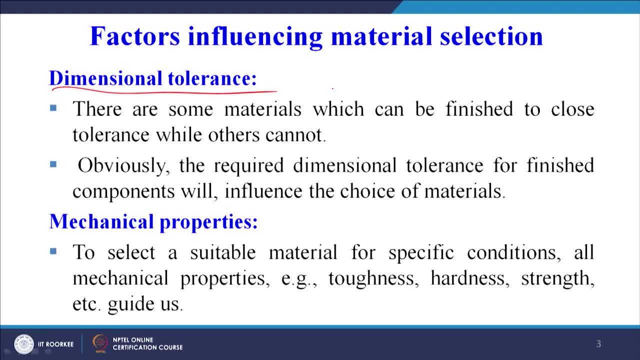 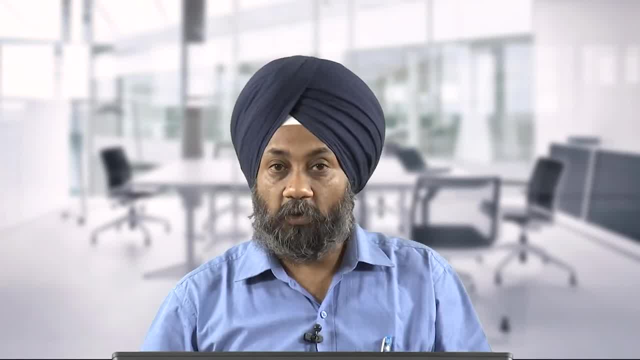 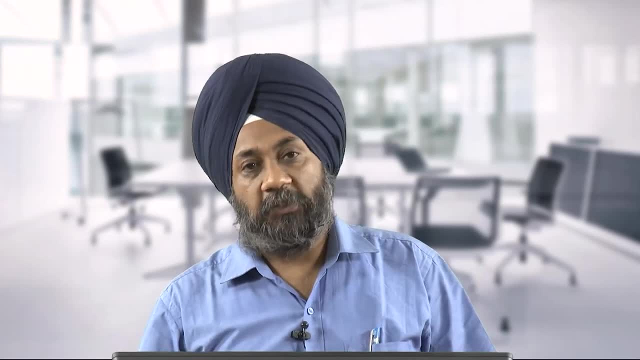 So we have to select a material depending upon the dimensional tolerance requirement in our product design. We have to select a material which can provide us that kind of dimensional tolerance. If we are not able to get the dimensional tolerance, the quality of our product will suffer. 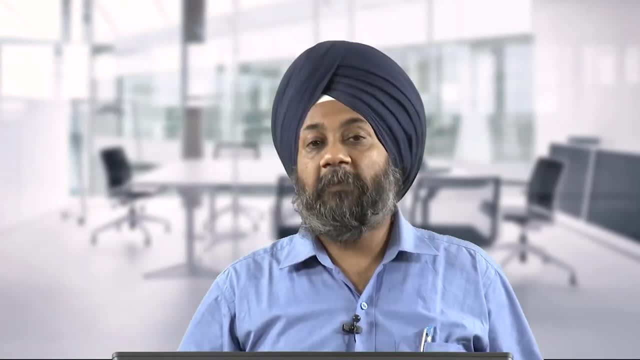 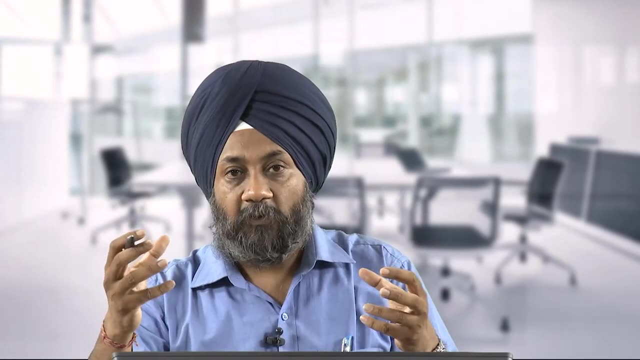 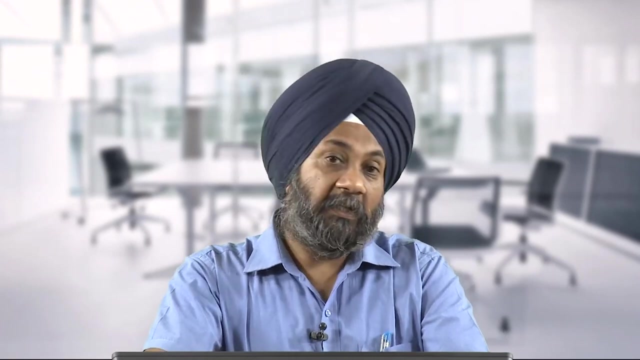 So therefore we have to select a material as per the dimensional tolerance achievable with that material. For example, if we talk of metal and a polymer, So with both We can achieve a certain degree of dimensional tolerance. So, depending upon the application, we will see that here better dimensional tolerance. 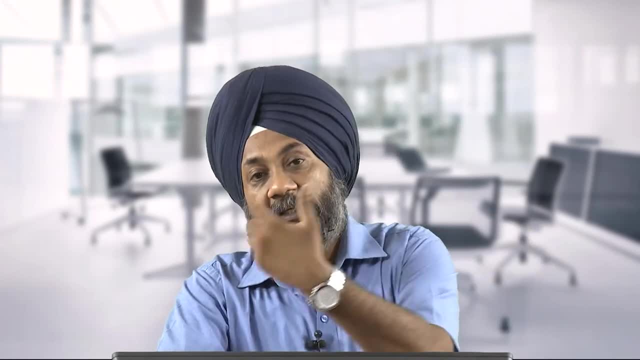 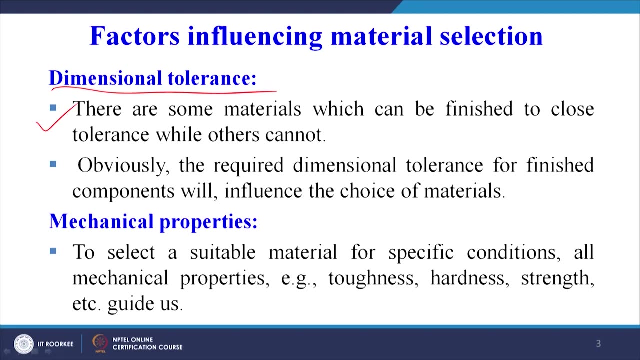 is required. So let us select X material and we can discard or screen out the Y material. Obviously, the required dimensional tolerance for finished components will influence the choice of materials. So then the mechanical properties, to select a suitable material for specific conditions. in place of conditions, we can write specific. 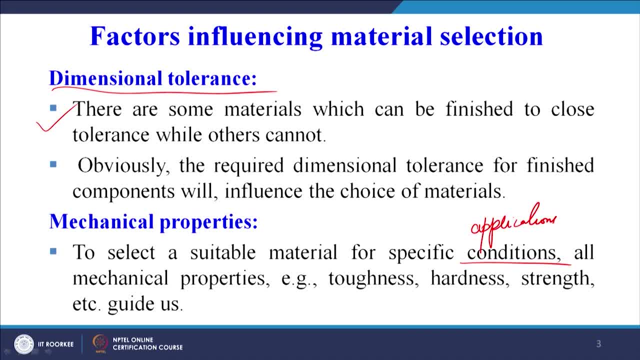 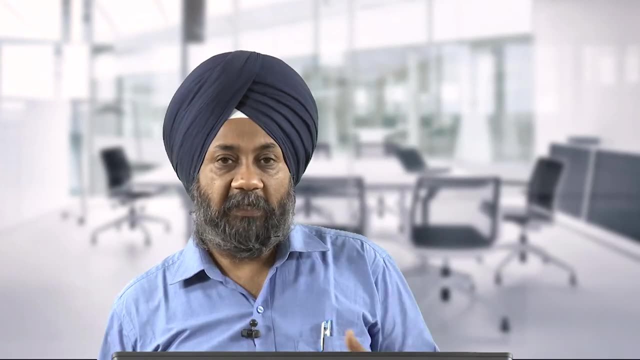 Applications also, which is subjected to different types of conditions, All mechanical properties. these are just the examples given, like toughness, hardness, strength, etc. They will guide us, they will act as a guiding factor. So whenever we select a engineering material, for example, we have to design a new design. 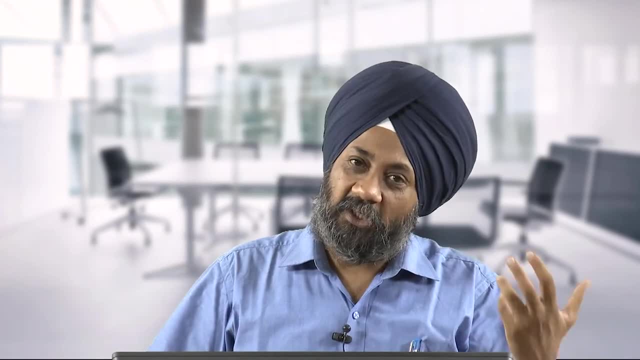 of a tie rod or of any engineering component. We have to design the design of a tie rod or of any engineering component. So whenever we select a engineering material, for example, we have to design a new design of a tie rod or of any engineering component. 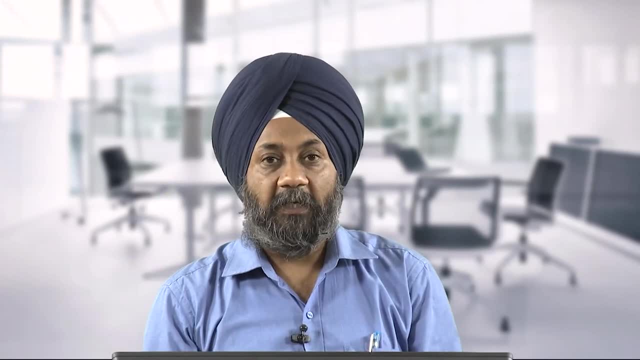 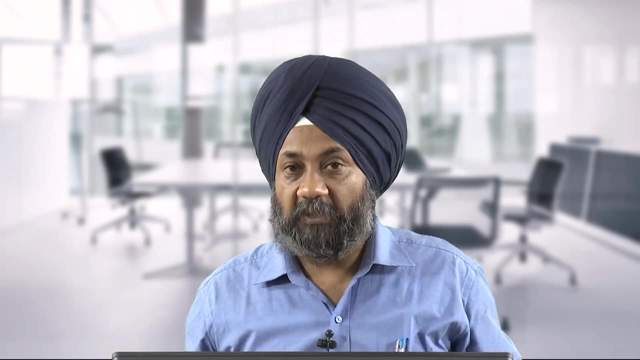 We will see the material property table and then see what is the tensile strength of this material, what is the compressive strength of this material, what is the shear strength, what is the impact strength, what is the modulus. we will try to see all the properties. 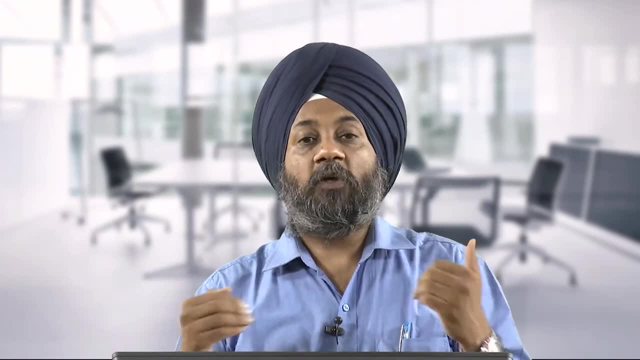 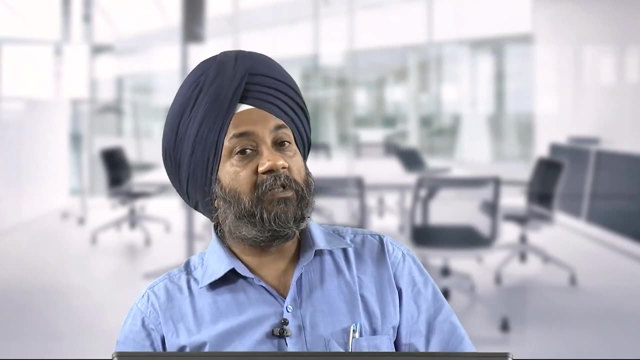 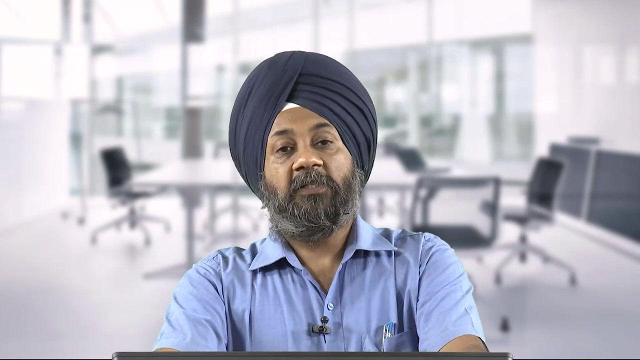 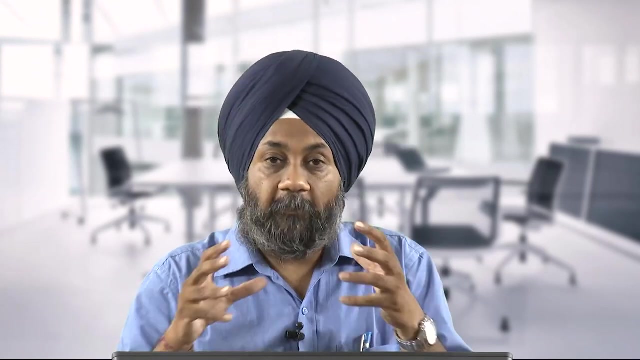 And finally, if the properties satisfy our requirements, then only we will select that engineering material or we will out of a library of engineering materials. we will select the material which is satisfying all the requirements that are that have to be satisfied for selecting a particular material. So we, for example, we design a particular product. we, as per the in service requirements, we list: 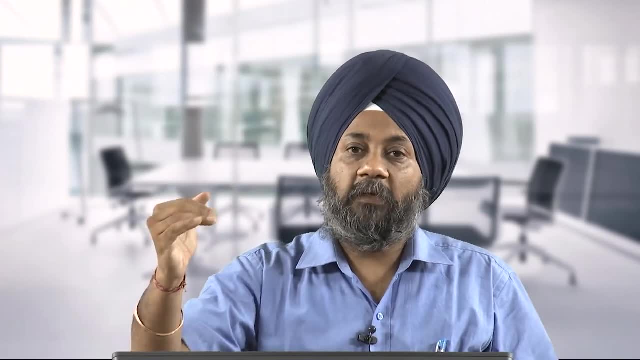 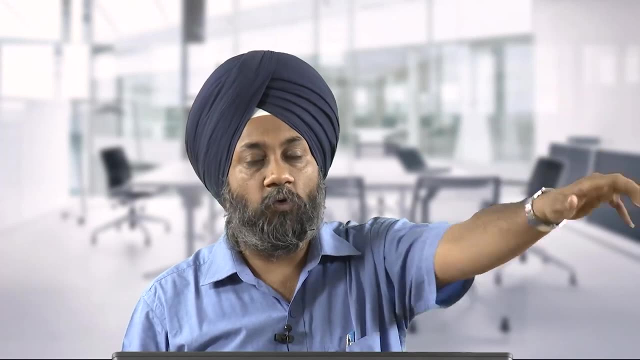 down that the tensile strength for this material must be more than this. compressive strength of this material must be more than this. So when we look at the data table or in the handbook of materials, We will see which material is satisfying this requirement. 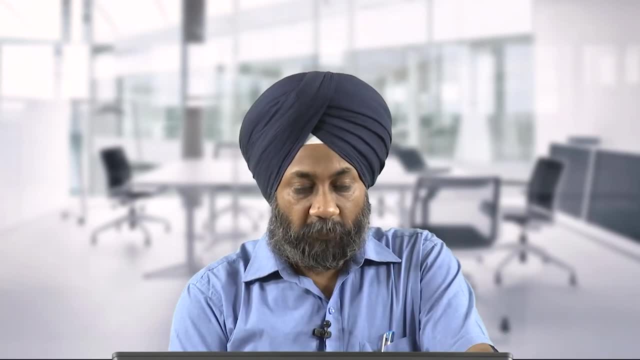 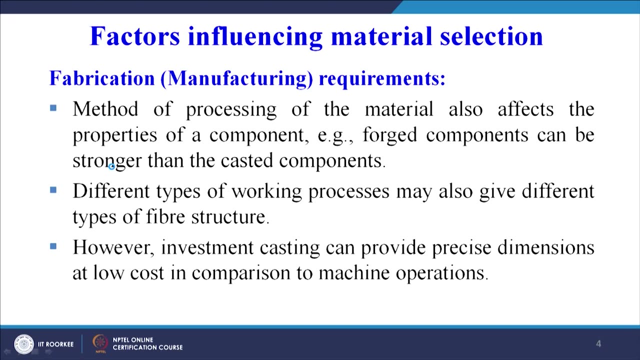 So with accordingly, we will select the engineering material. So the mechanical properties play a very important role in the selection of the material, Then the fabrication of the manufacturing. the second column that we have seen in the diagram today, Method of processing of the material, also affects the properties of a component. 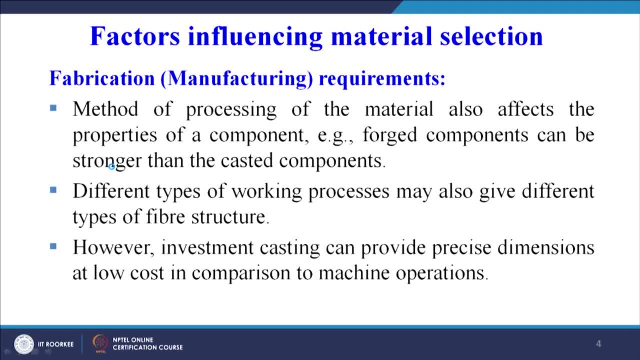 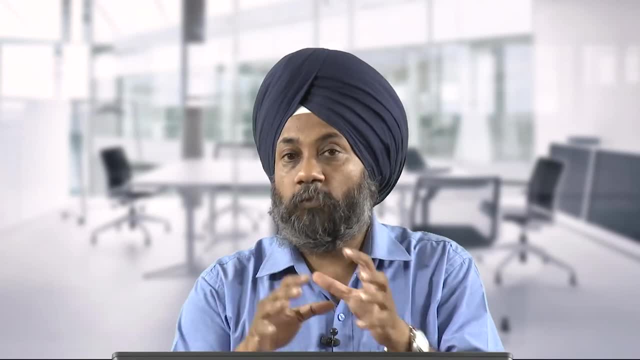 For example, forced components can be stronger than the casted components And therefore The manufacturing process will also play a very important role in the choice of material. Now we want higher strength for our engineering component And we are going to use forging process to get that higher strength. 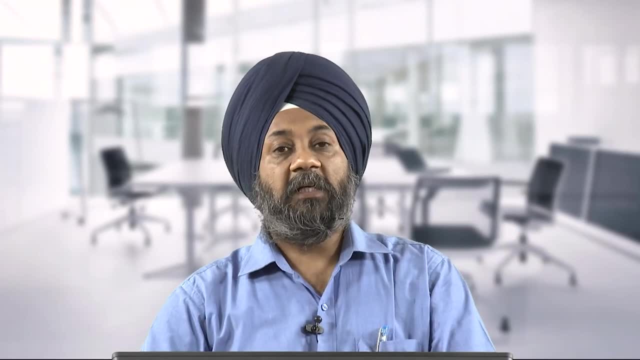 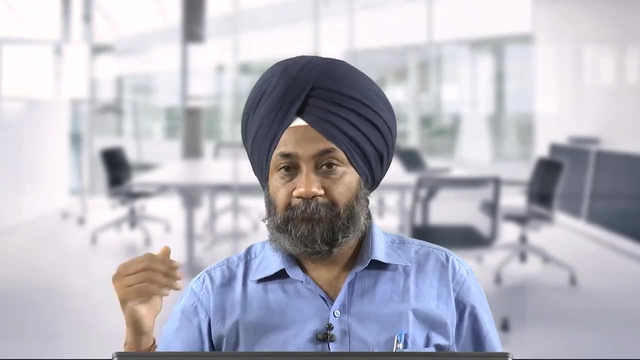 Then the material also has to be selected in such a way that it can be forced properly. It must not happen that we have selected a material which is not, we can say, friendly to the forging process. So that is the selection of the process. Okay. 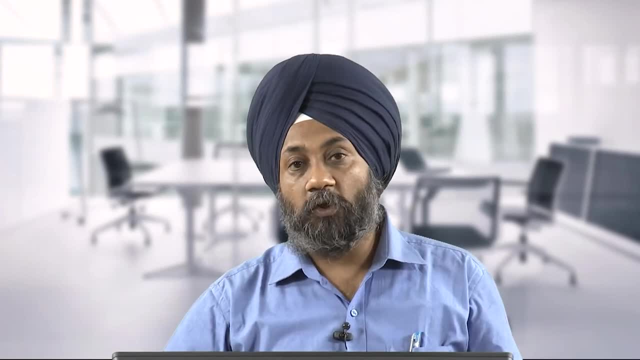 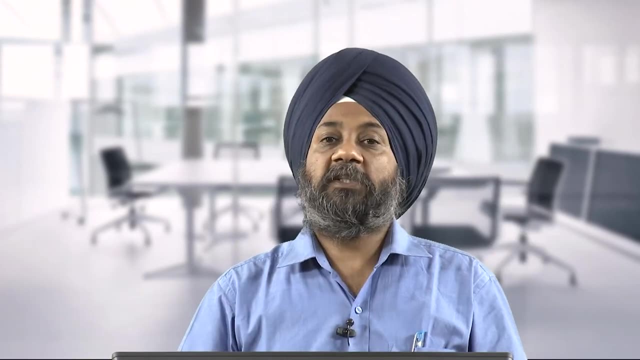 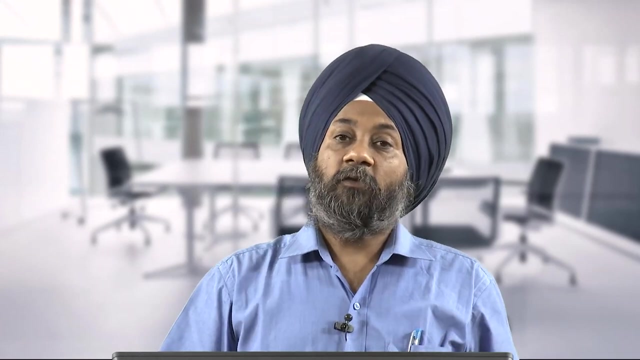 So the selection of the process will also have a influence on the selection of the material, And vice versa also, selection of a material will also have a influence on the selection of the manufacturing process. So different types of working processes may also give different types of fiber structures. 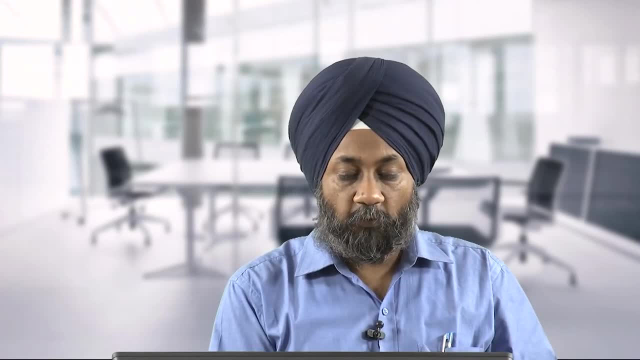 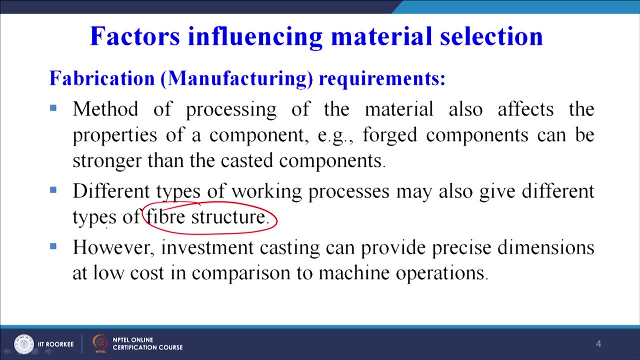 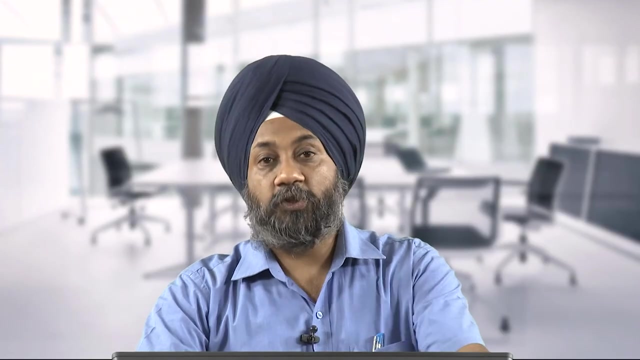 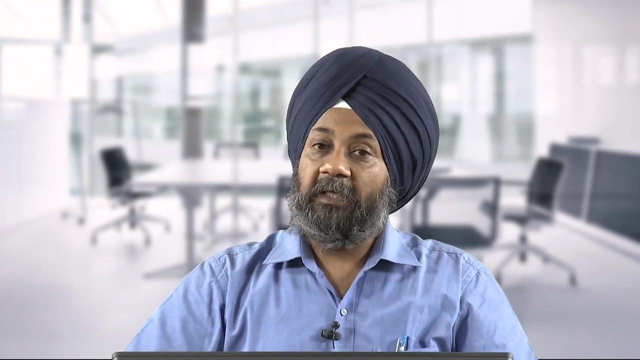 or the microstructure. Fiber structure is specifically, if we talk about the composite materials, more specific about the polymer matrix composite materials. But if we talk about the metals, when we process them using different types of processes, their microstructure also gets affected. So if the microstructure gets affected, the properties will also get affected. 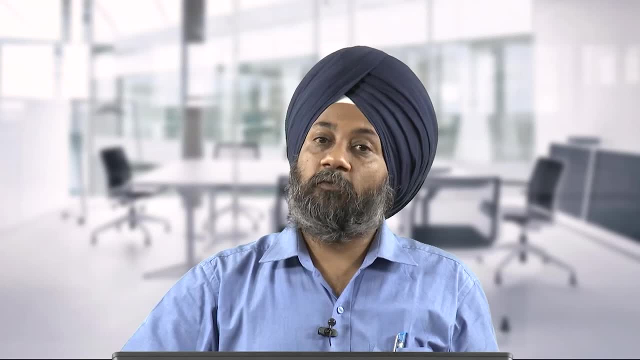 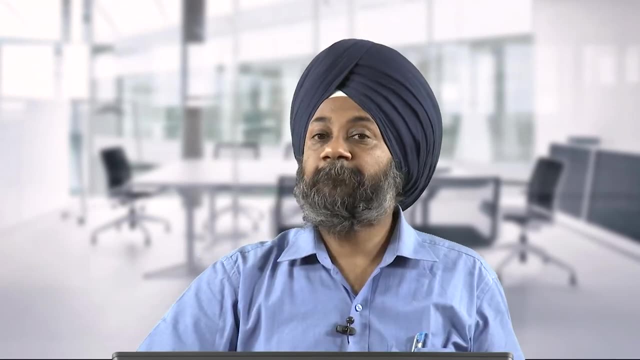 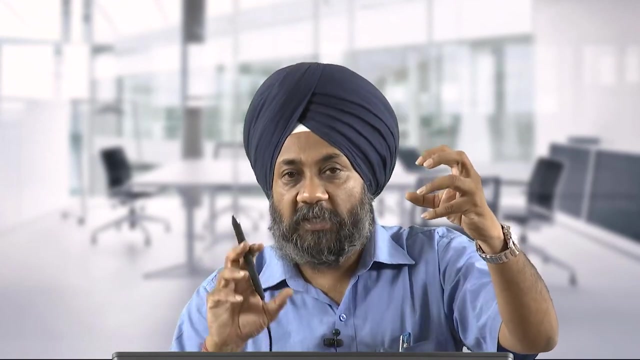 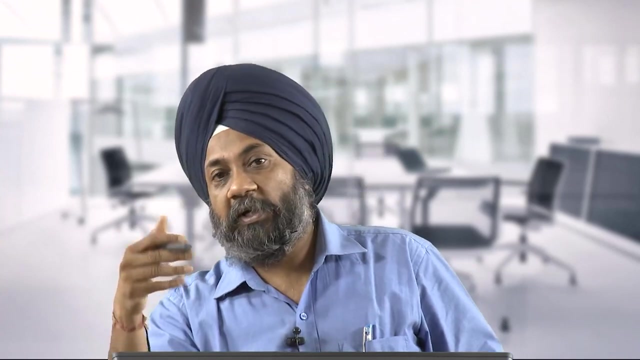 And these properties will definitely influence their performance during the. in service or in service performance of the components will be affected by the manufacturing process. So we need to understand that we have selected material X, we are processing it with process Y. so material X processed by process Y. how it is going to? 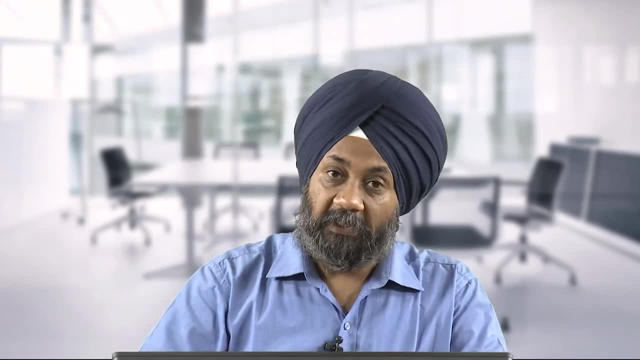 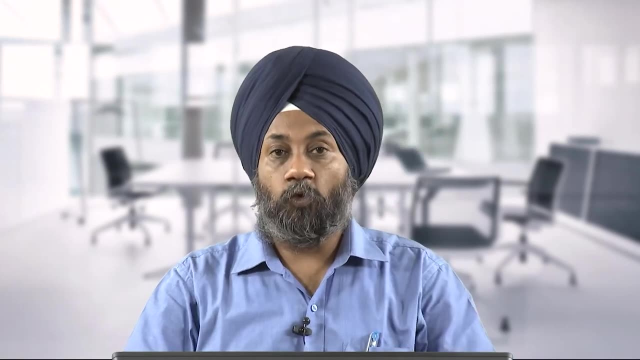 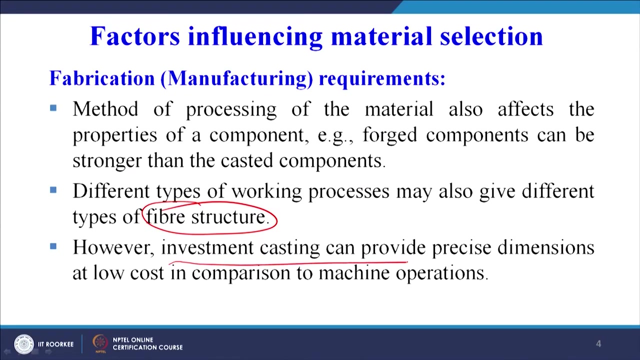 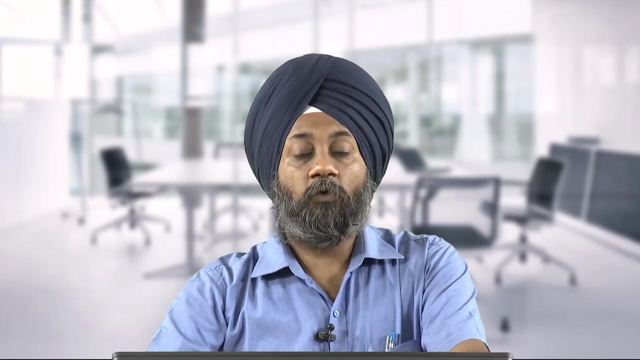 influence the microstructure of the material And how that microstructure is going to affect the performance of the material when it is going to be exposed to the service requirements. So one example is taken here: investment casting can provide precise dimensions at low cost In comparison to the machining operation. so when very good example is taken here that 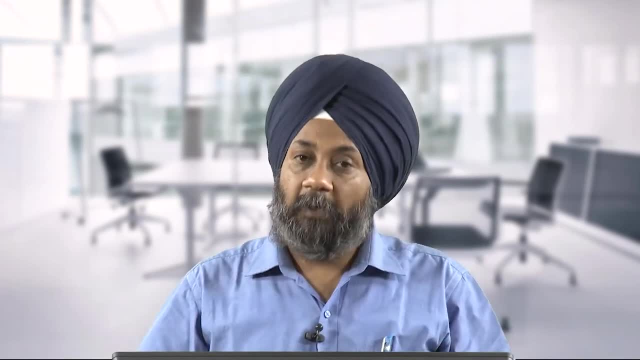 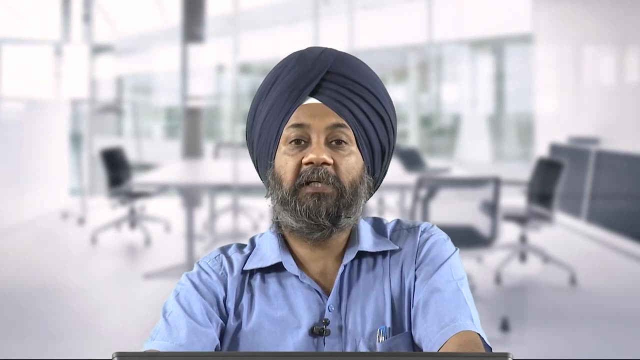 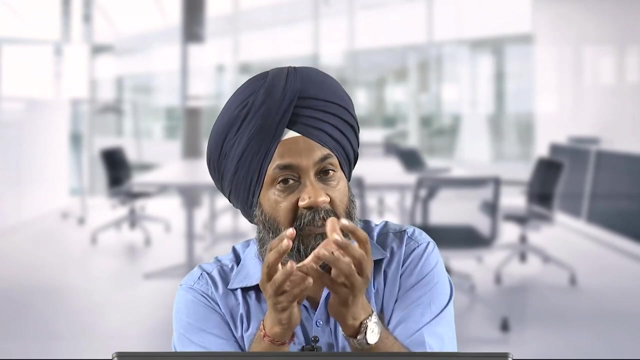 if we have to make a very intricate metallic part We must go for investment casting, because machining of those intricate features will definitely add a lot of cost of processing into the product. So investment casting is better when the very, very intricate details are required in our 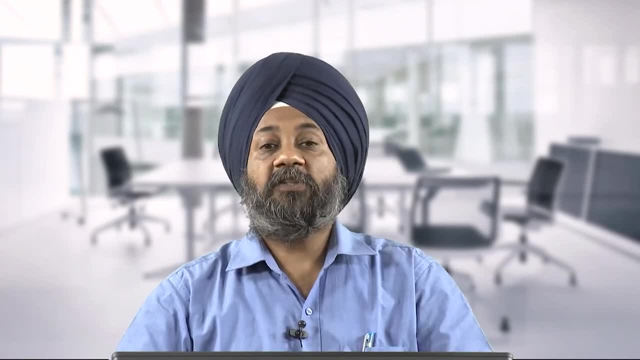 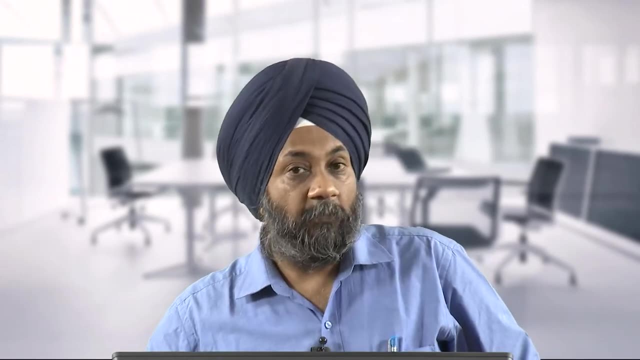 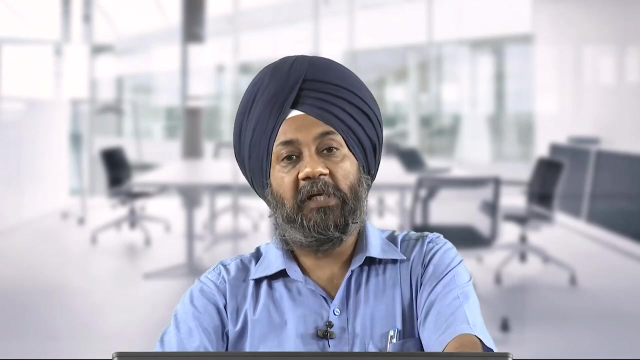 product. So the product can be a jewelry item. We see that a jewelry items are very, very intricate details. So if we start machining those intricate details, it will be a very, very expensive proposition. So it is always better to use investment casting for intricate metallic parts. 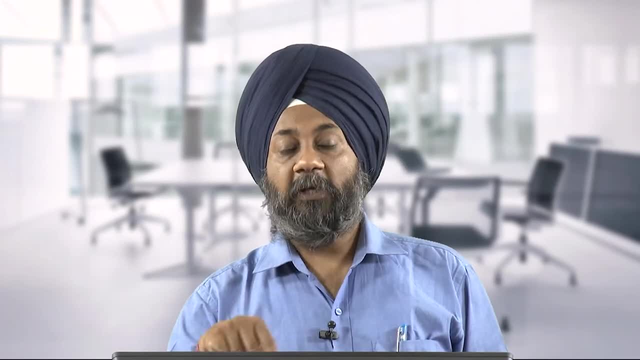 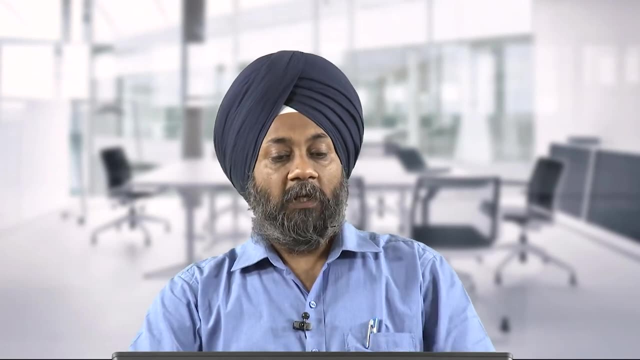 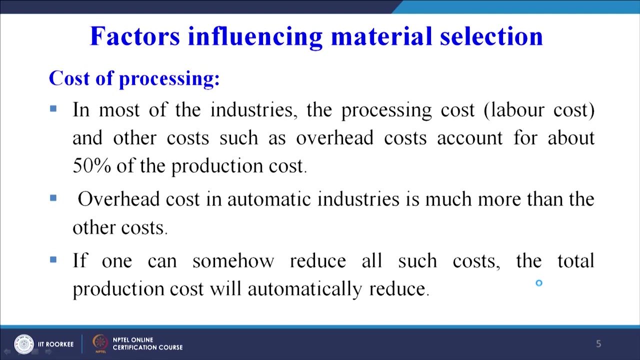 This is one example related to how manufacturing processes can also influence the selection of the engineering material. Now, the cost of processing also is very, very important. In most of the industries, the processing cost and other cost, such as overhead cost, account for 50% of the production cost. 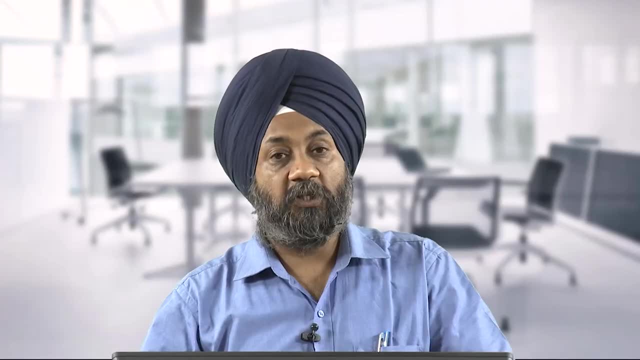 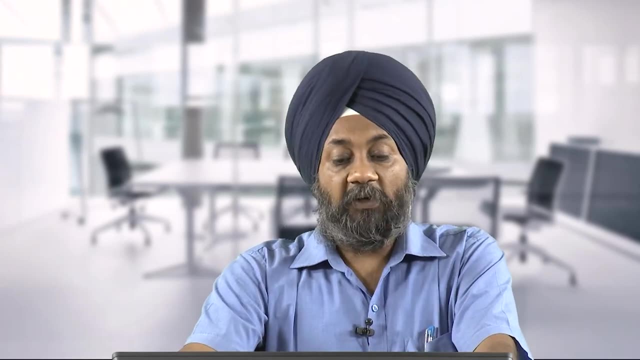 So once we select the process and the materials, we must keep in mind this 50% commitment for the production or for the cost of production. Overhead cost is automatic. in automatic industry is much more than the other cost. So if one can somehow reduce all such cost, the total production cost will automatically. 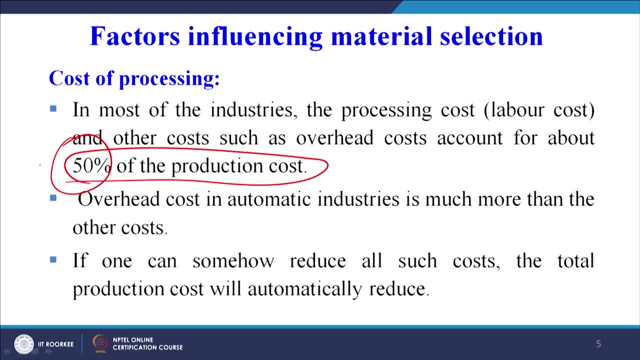 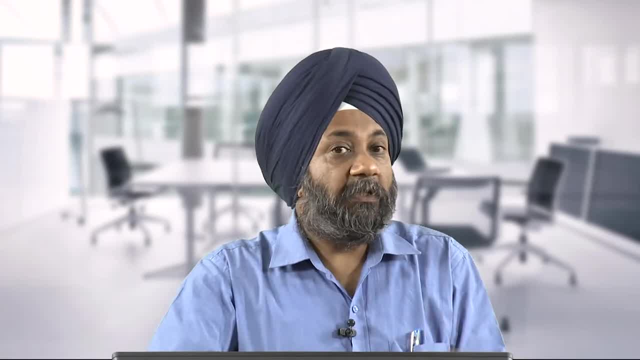 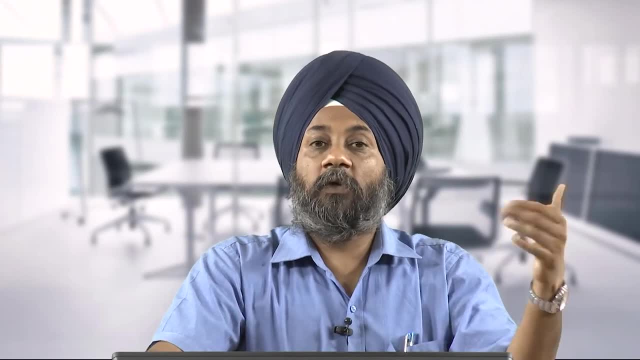 So if one can somehow reduce all such cost, the total production cost will automatically reduce. So this is not particularly relevant with the selection of engineering materials but is definitely relevant from the selection of a manufacturing process point of view And indirectly is going to affect the selection of materials also. 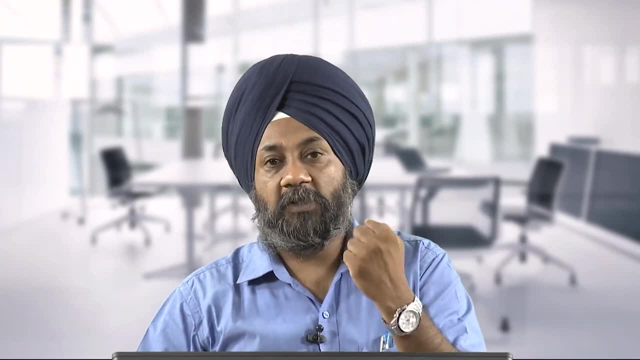 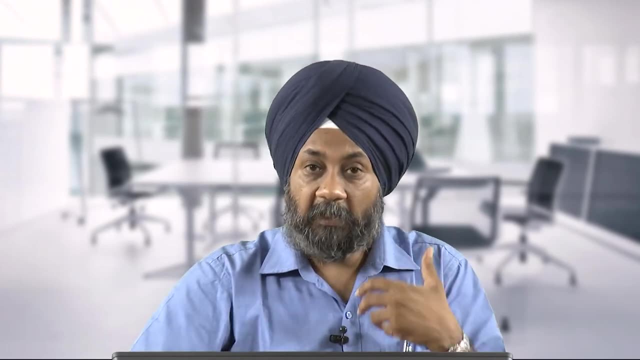 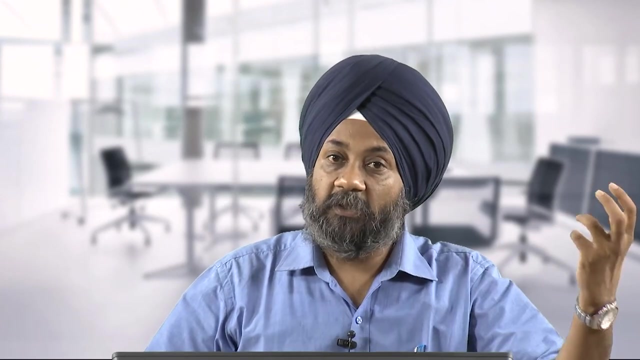 Because some materials can be processed with automatic machines and therefore the overhead cost will be influenced. Some materials may not May be, But they will expose themselves as a good candidates for automation. So accordingly, we will see that we have, we have to select a material which will influence. 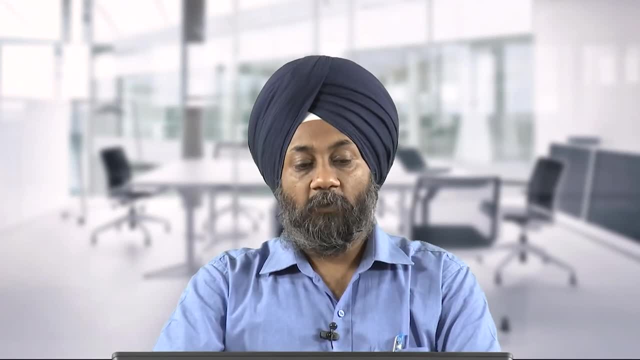 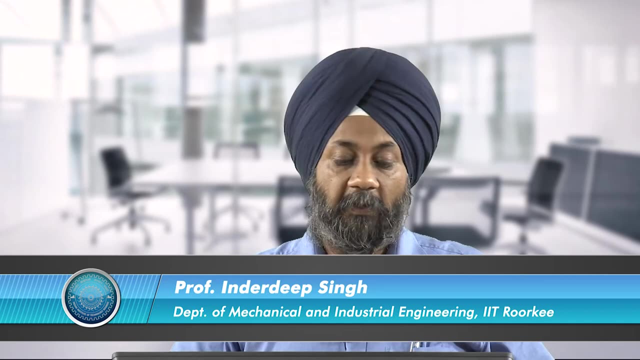 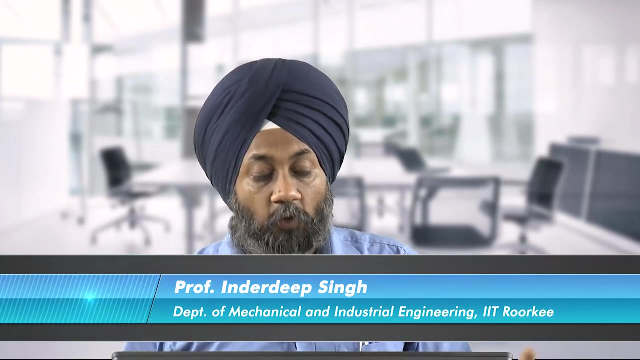 the overall production cost of the product. Availability of the material is very, very challenging task. We may find that sometimes the availability of material becomes a governing factor. The material is not available. what to do in those cases when the desired material supply is limited? 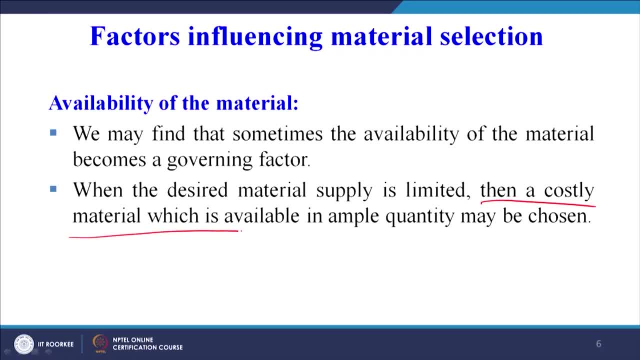 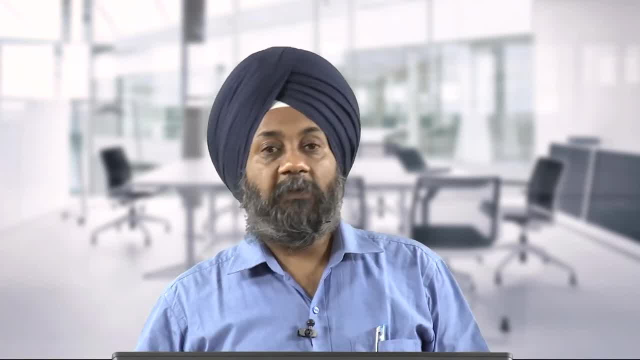 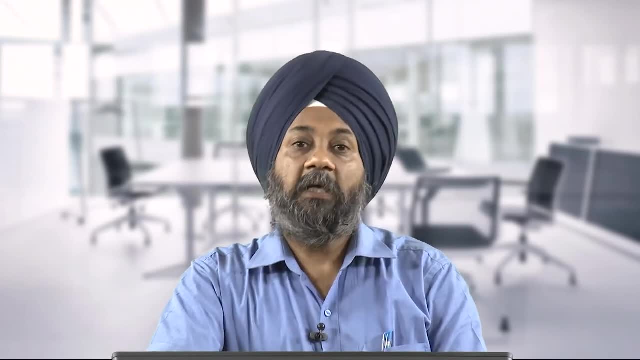 Then a costly material which is available in ample quantity may be chosen. So we have to see the availability. sometimes the material that we wish is not available, So we have to go for a material which is easily available. Maybe we may have to pay certain additional money or premium to get that material. 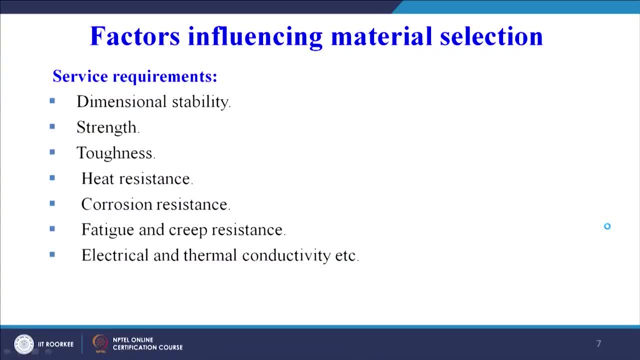 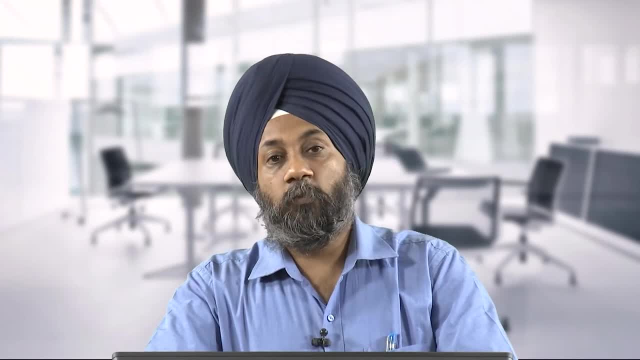 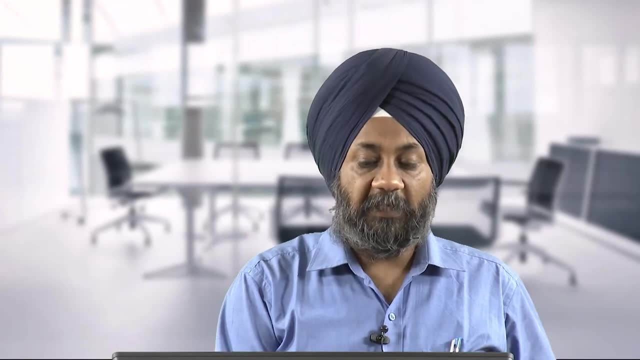 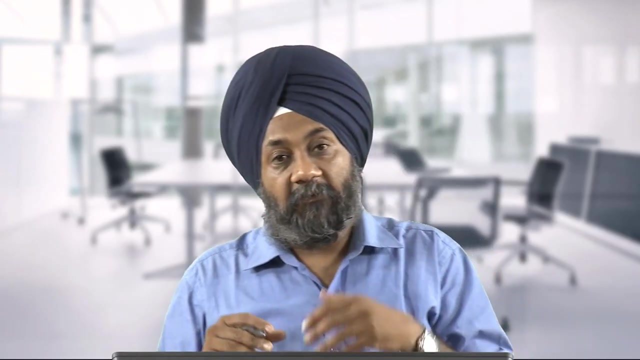 So the factors influencing material selection, service requirements, The kind of conditions The Product is going to be exposed to is definitely going to influence the material selection And therefore the dimensional stability may be the dimensional stability on exposure to the heating condition. So, if you remember, we have already seen that polymers are not that good under hot temperatures. 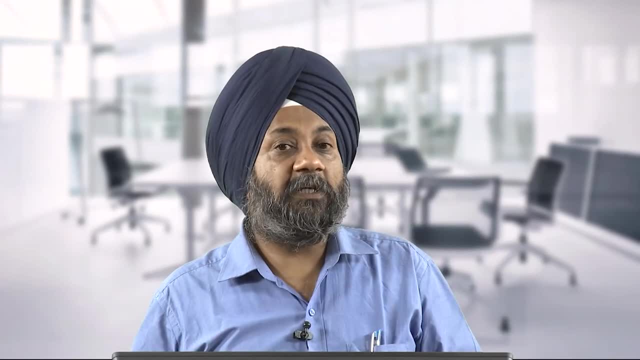 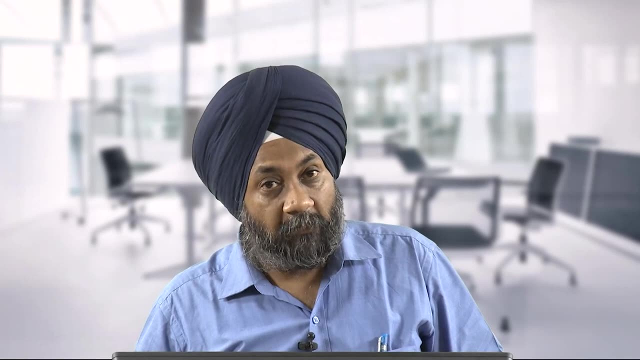 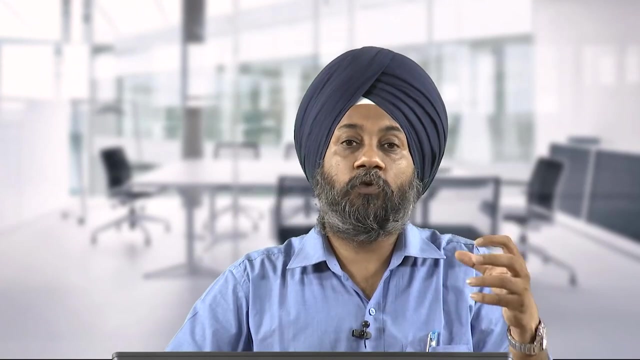 or at high temperatures. So in those cases the dimensional stability may become an issue. So, similarly, the strength must not get affected By The environment. for example, the component or the part has to be used in the freezing conditions, or a metallic part exposed to the freezing conditions over a long period of. 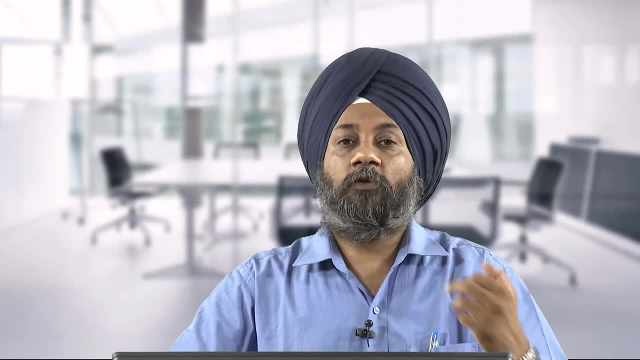 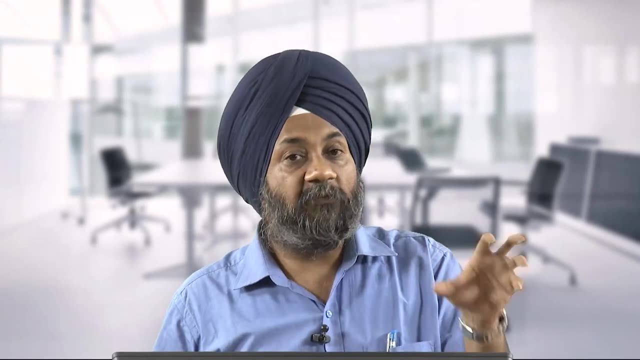 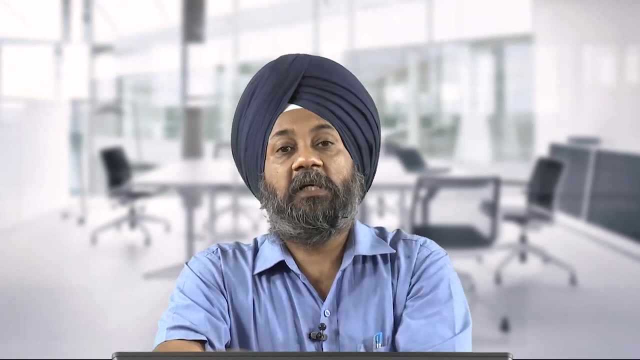 time. So the freezing conditions may affect the strength of the material. So therefore the in service conditions also play a very important role while deciding that which material must be chosen. So the material must not be susceptible to the environmental conditions or the service requirements. 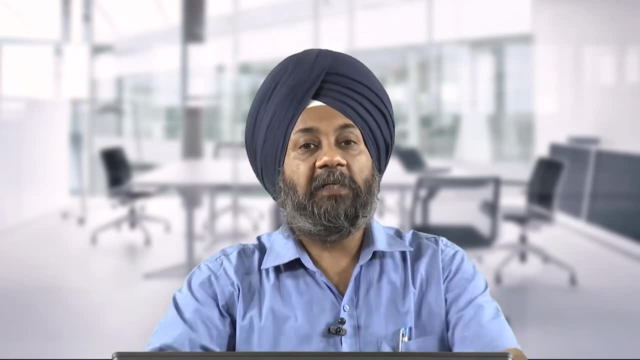 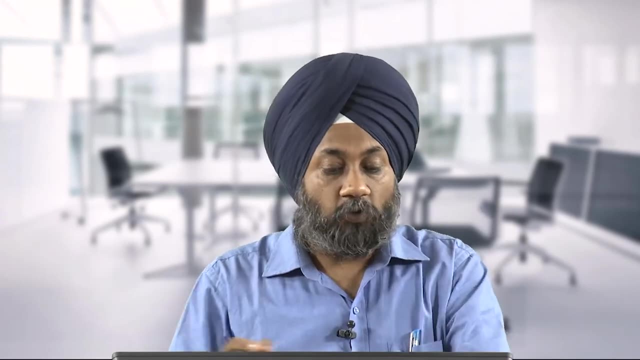 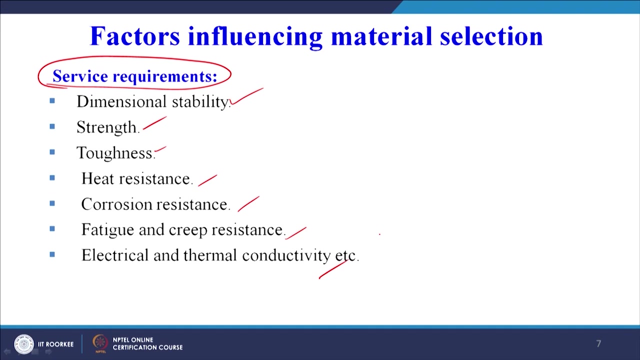 Many times the wear and tear may be a important design criteria. So we have to select a material which has hard surface so that the wear and tear does not take place. So the toughness, heat resistance, corrosion resistance, fatigue and creep resistance, electrical and thermal conductivity. 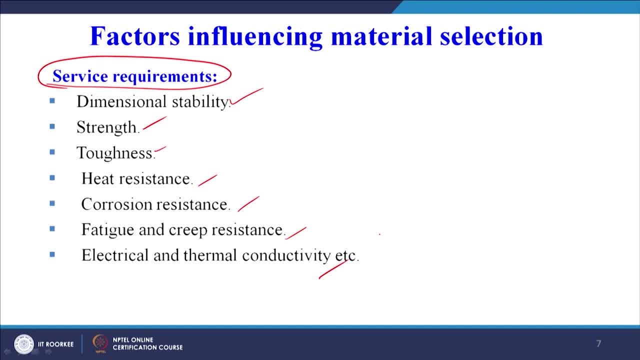 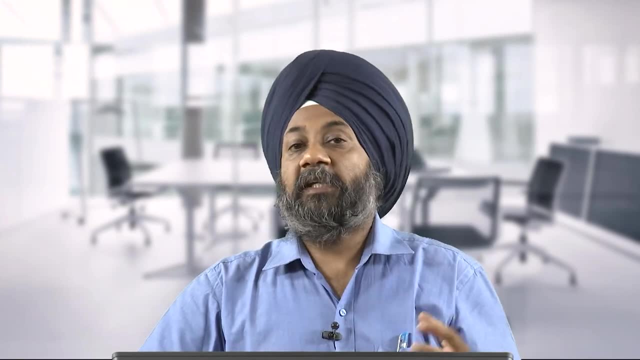 So, depending upon the situation in which the product is going to be used, it is also going to affect the choice of the material. So we have to decide that what is the material with which we are going to make that product. So example already I have taken that if the material is not that resistant to heat, we must 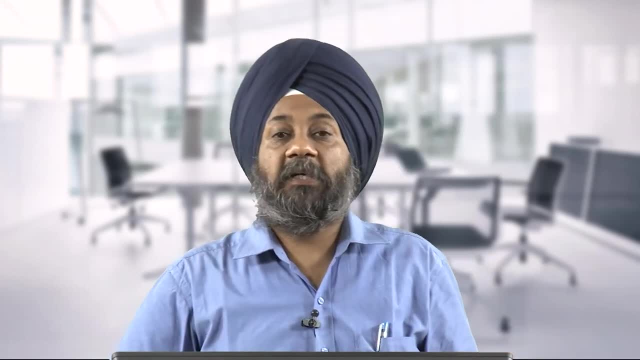 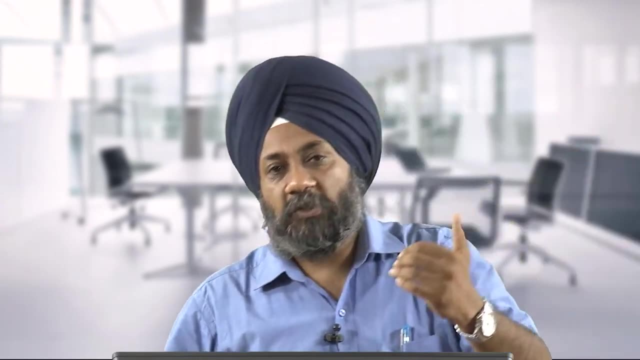 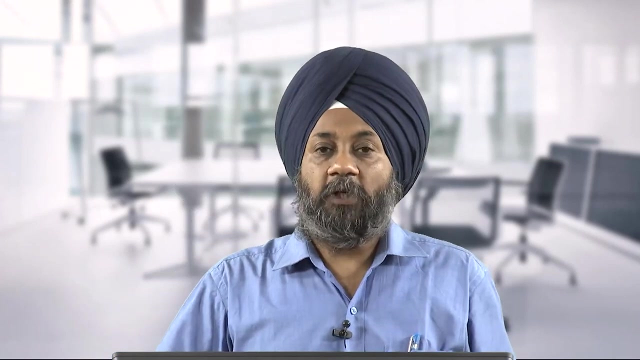 select a material which is better heat resistant, For example the ceramic material. So wherever the temperature they are going to be too high, we must avoid the use of polymers there. We must purpose the use of ceramics in those circumstances. So, depending upon the kind of material that is available, 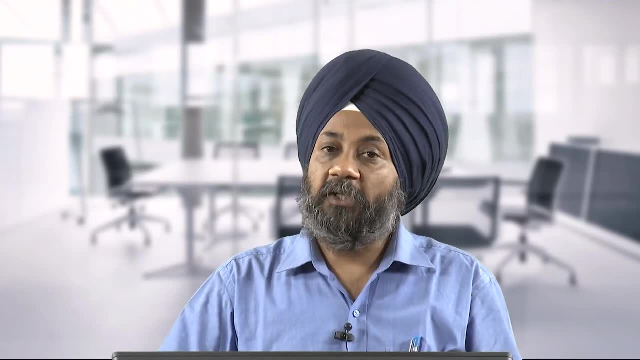 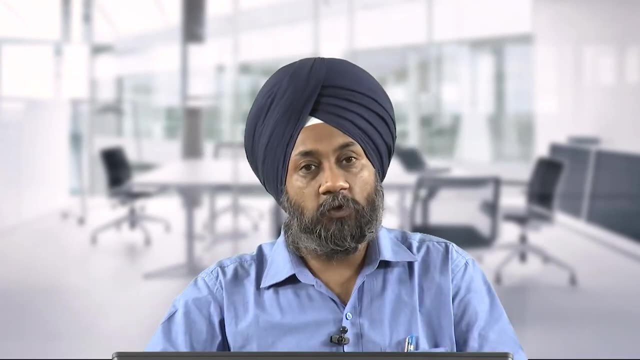 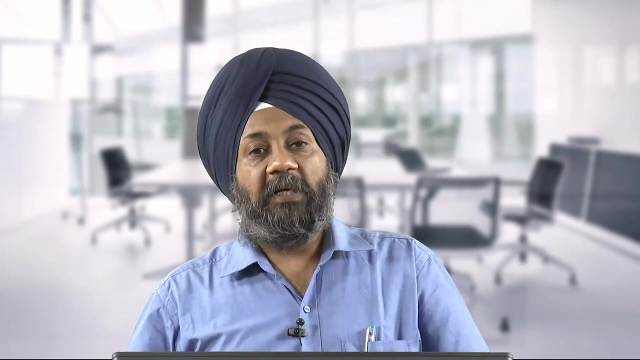 Depending upon the kind of conditions we must select. our engineering material, as well as the in service requirements of the product will definitely dictate the choice of the material for a specific application. Now the selection of materials. let us try to take an example that how we will go about. 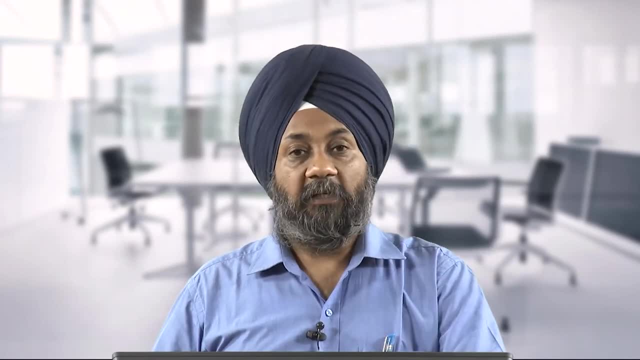 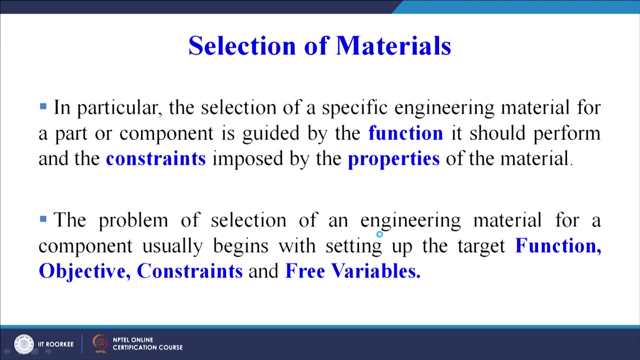 selecting a particular material, or what is the procedure that we must follow? So, in particular, the selection of a specific engineering material for a part or component is guided by the function. Already in the previous slide this discussion has come into picture. The function is very, very important. 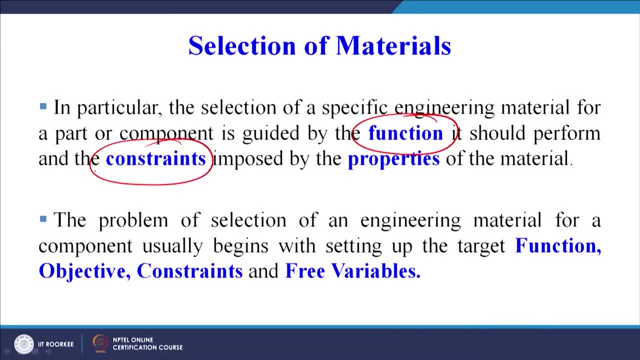 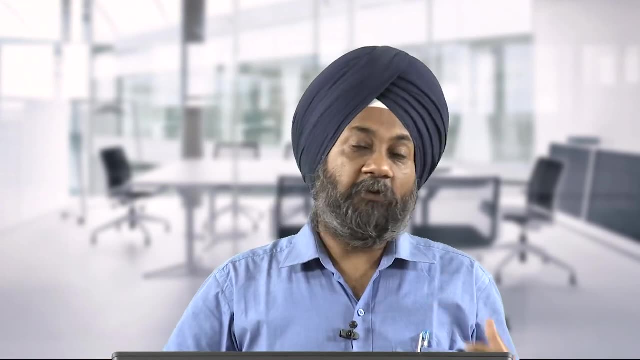 It should perform and the constraints imposed by the properties of the material. Now, properties of the material: already we have seen properties can be the physical properties, then there can be Can be chemical properties, then there can be mechanical properties. So the properties of the material will definitely pose certain constraints and we have to see 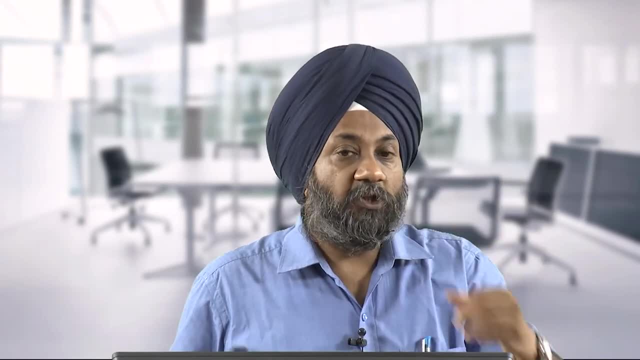 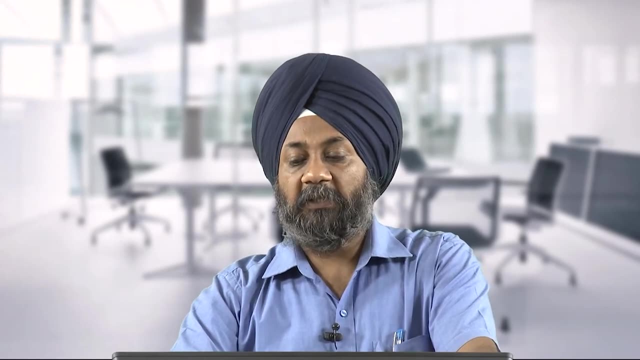 that what is the intended function of the product which is being designed. The problem of selection of an engineering material for a component usually begins with setting up the target function. So first we need to see what is going to be the function. and regarding the function and 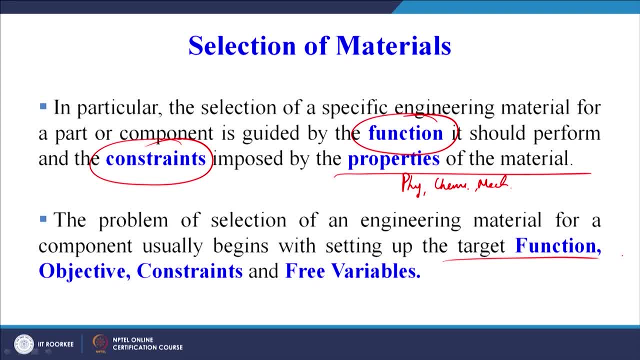 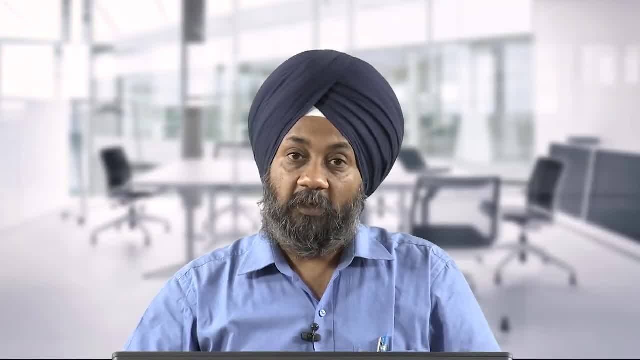 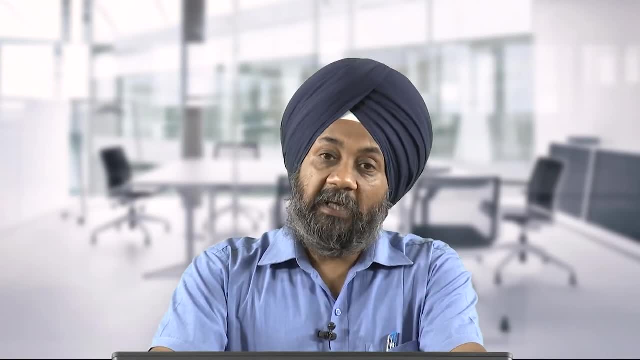 the functional analysis We have taken Already recorded a course on product design and development in which we had discussion on value engineering, which is an important technique that we use for functional analysis of a product. So we try to understand the function of a product. 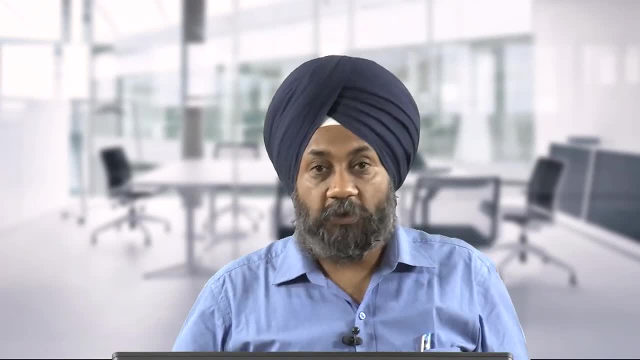 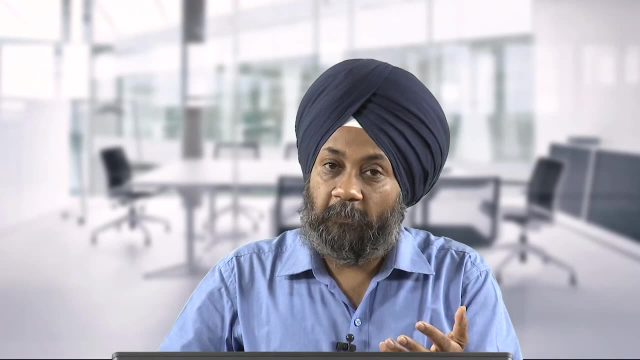 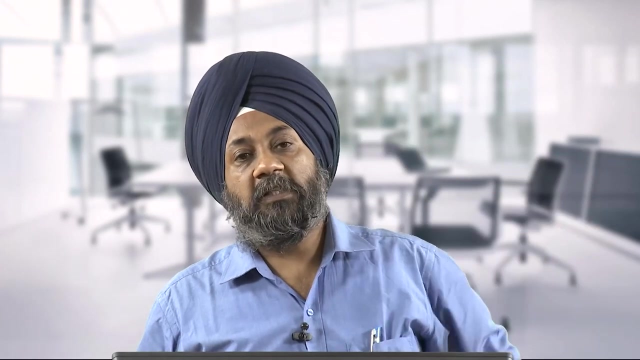 For example, if we say the spectacles that we use. So what is the function of spectacles? the function is improve vision. if we use newspapers, the function, The purpose of newspaper is provide information. if we talk about watch or a wall clock, we will say display time. 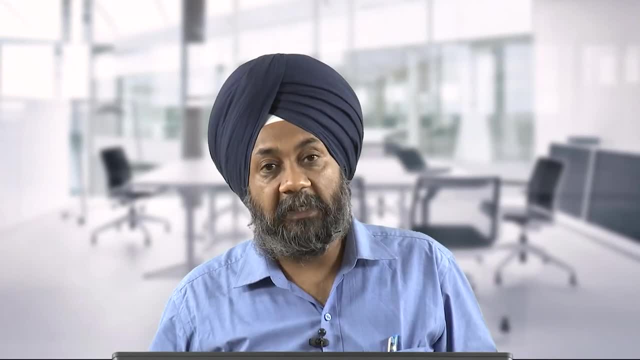 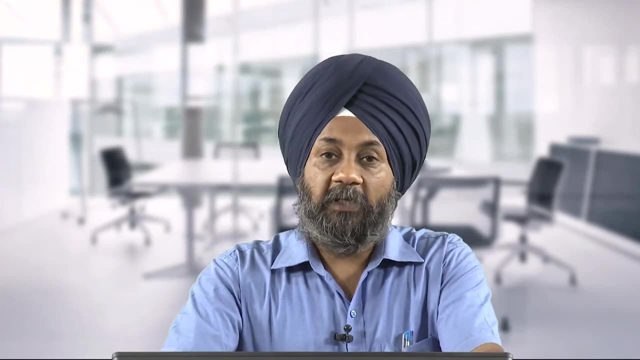 So 2 word functional definition for each product we can take. So for any product that we are designing, we must first list down what is the function which is the product is going to be designed for, or what is the intended function of the product being designed. 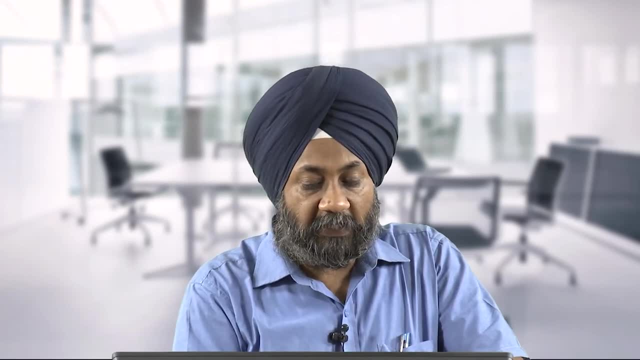 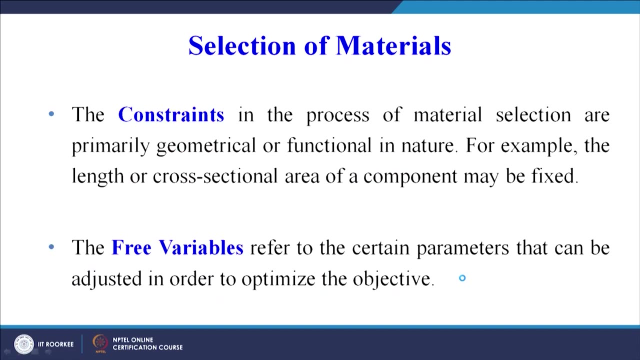 Then we have to look at the objective. what are the constraints in terms of the material properties and finally the free variables. So let us quickly see these. the constraints in the process of material selection are primarily the geometric or the functional in nature. For example, the length or the cross sectional area of the component may be fixed. 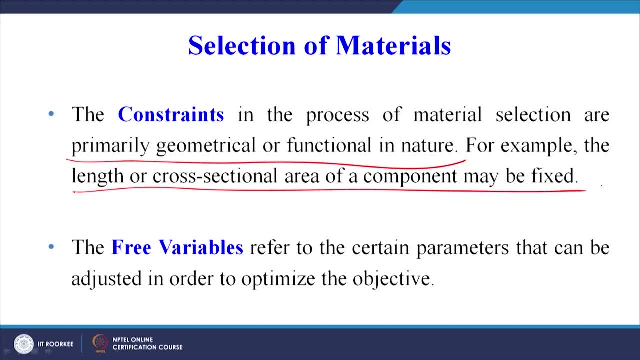 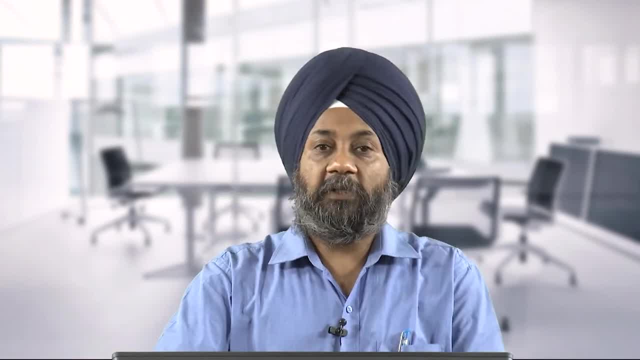 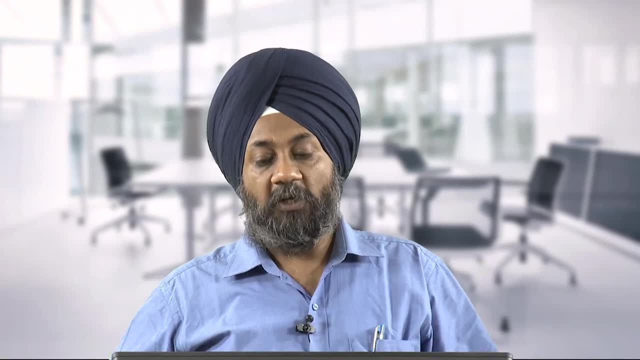 So that is a constraint. now, for example, this dais has to be designed, So what is fixed here? the height of the dais is already fixed, So that is a constraint. So The height, weight, sturdy, strong. it must not be having any kind of vibration. 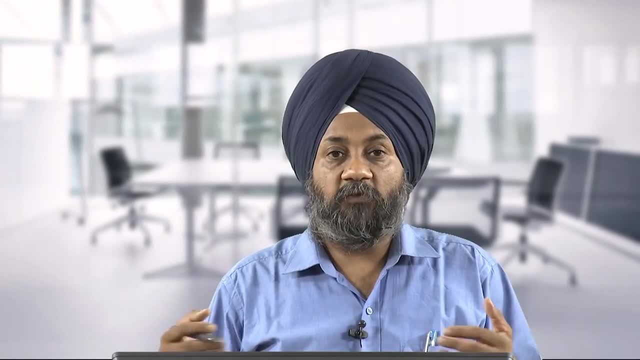 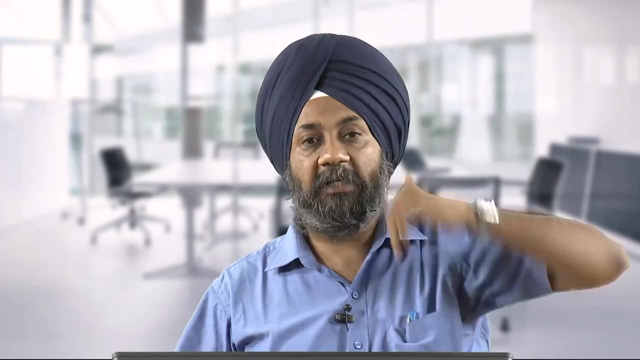 So these are some of the important design features which have to be included in the design of this dais. But one of the things is a constraint: the height. we cannot have a dais up to this much height. the speaker is not visible behind the dais. 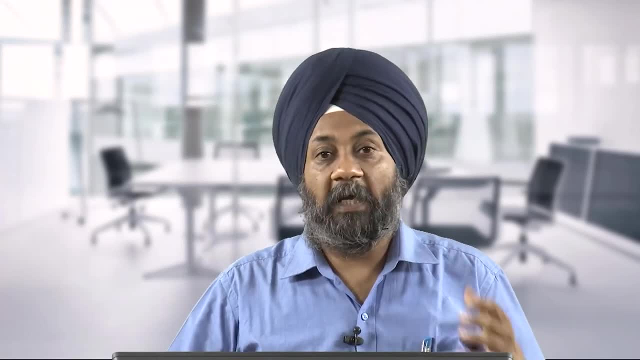 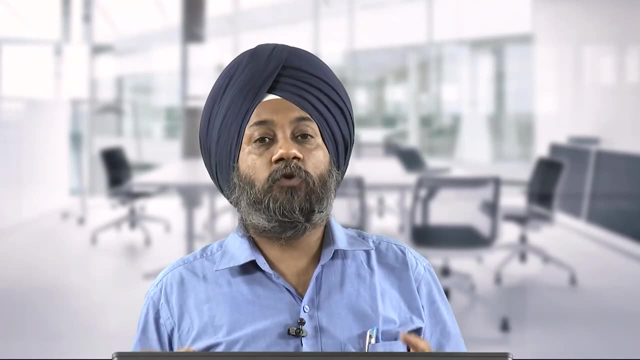 So that is not may be advisable, that is not going to help it achieve its desired function. a desired function is to provide a platform for a speaker to stand, keep the console and deliver a lecture. So that is what one thing is fixed, that is, the height is a constraint in case of design. 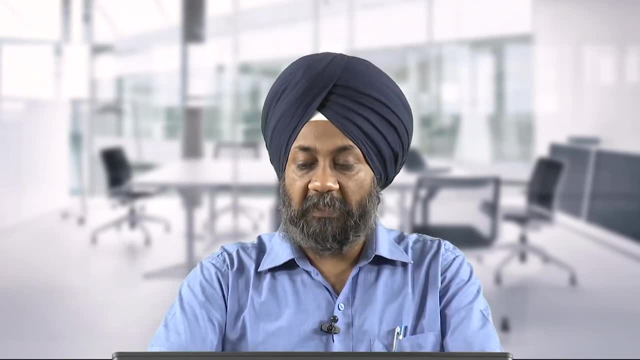 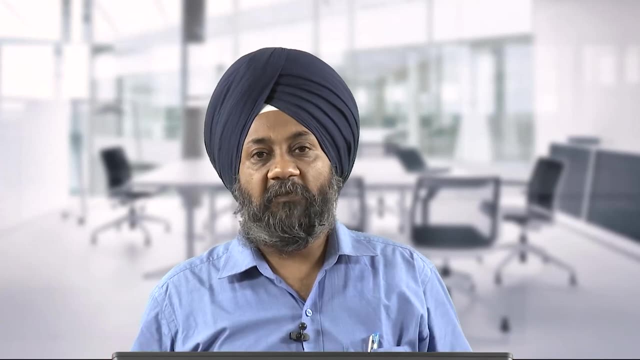 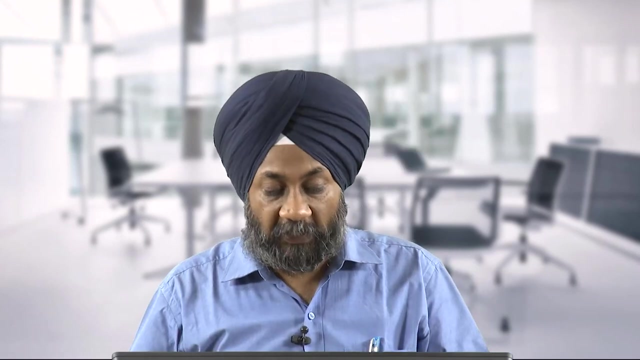 of the dais. the free variables refer to the certain parameters that can be adjusted in order to optimize the objective. Now there can be certain free variables here which will help us to adjust our objective or which we need to adjust in order to optimize our objective. 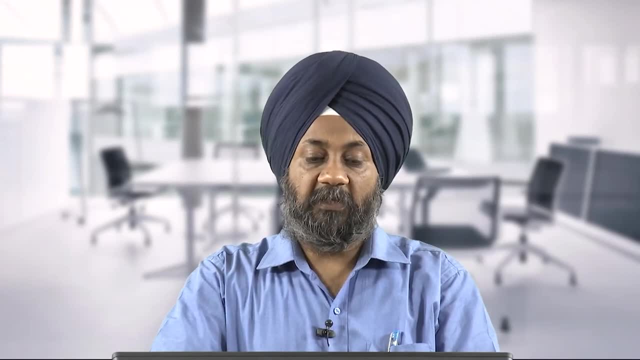 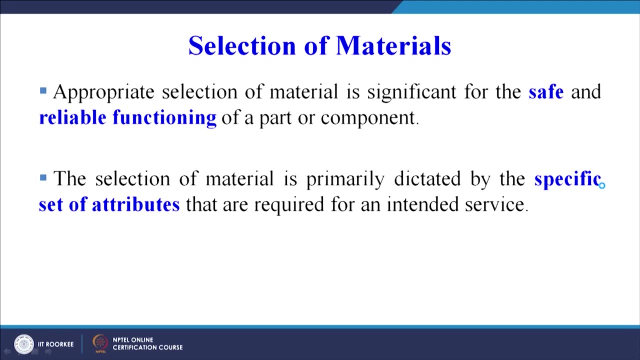 So the free variables. we will take an example in the subsequent slides. So that is what one thing is fixed slides. Then appropriate selection of material is significant for the safe and reliable functioning of a part or component. The selection of material is primarily dictated by the specific set of attributes that are: 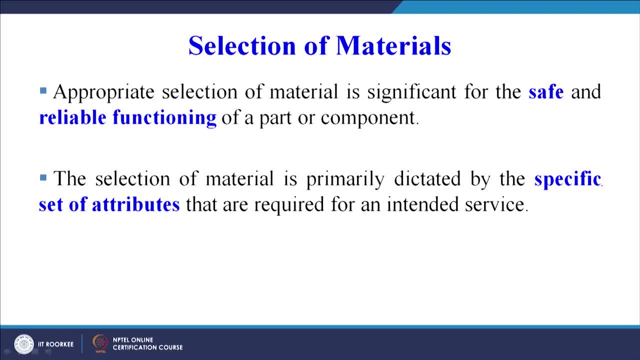 required for an intended service. So both these points already I have discussed just now, maybe 5 minutes back, when we talked about that. we have to focus on the intended function of the product and accordingly we have to select our engineering material. So the selection of material is primarily dictated by the specific set of attributes. 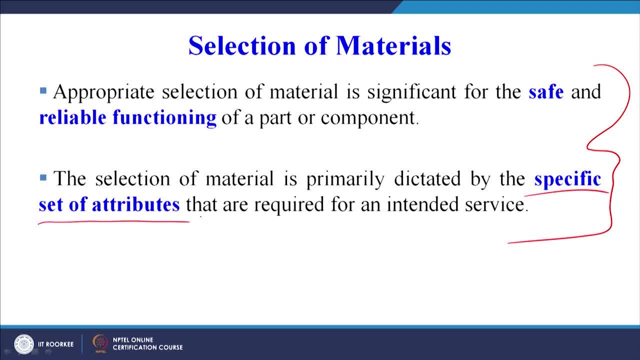 So the important point is already highlighted: Specific set of attributes that are required for an intended service. So what is required in the product so that it is able to perform its intended function? So that will define that which material has to be selected for this product, based on the 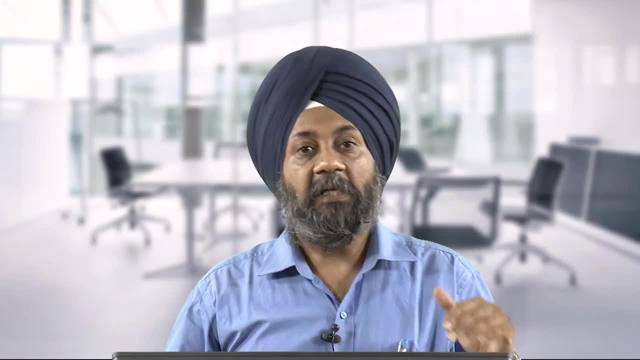 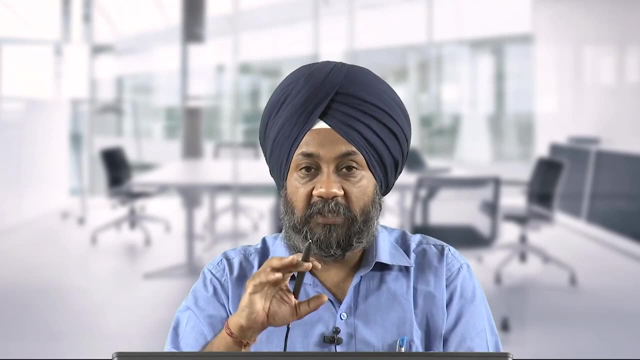 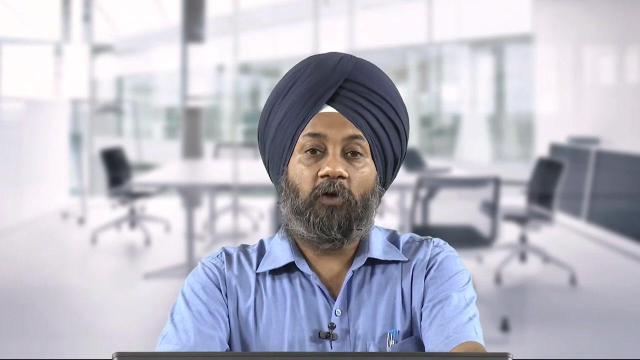 constraints and the free variables That we have already discussed. there are certain constraints which have to be taken into account and free variables that we need to adjust in order to satisfy our overall objective. Now we come to a term which we call as the material index. 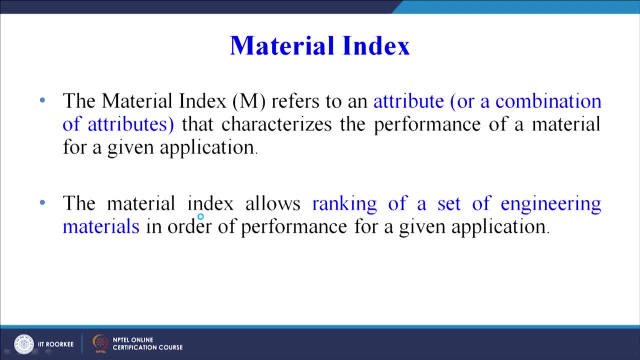 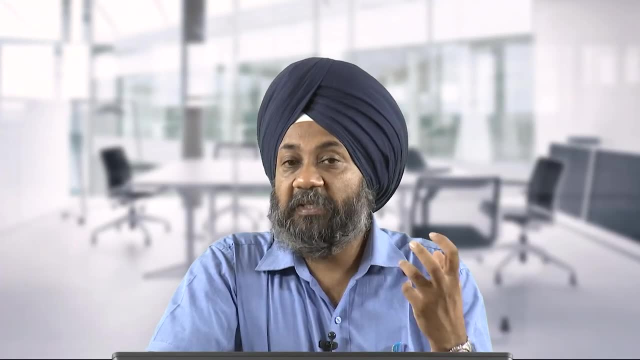 So the material index refers to an attribute, or it can be a combination of attributes that characterizes the performance of a material for a given application. So material index, Material index, will guide us in the selection of a particular material or a specific material for a specific application. 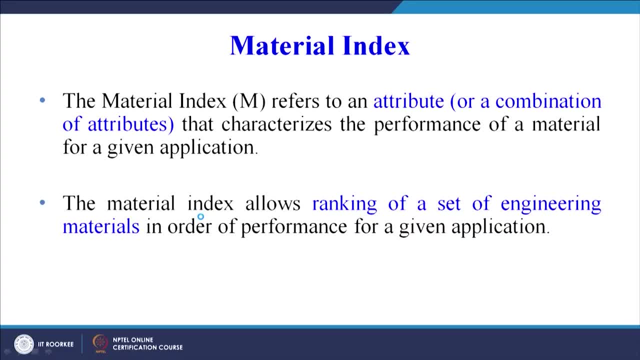 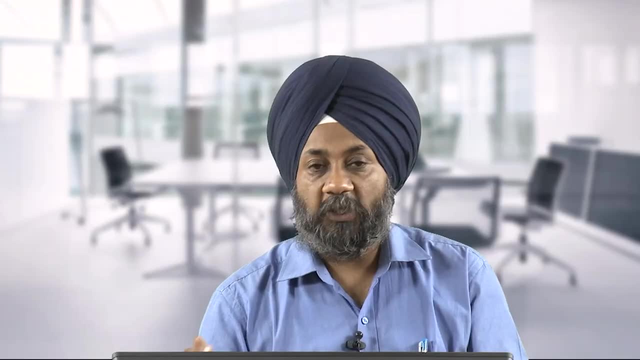 So the material index allows ranking of a set of engineering materials in order of performance for a given application. Now suppose we have a given application which we can characterize as capital A, and there can be number of materials which can satisfy this application or can be used for this application. 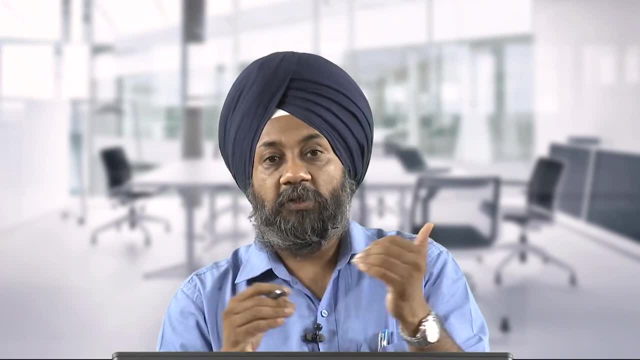 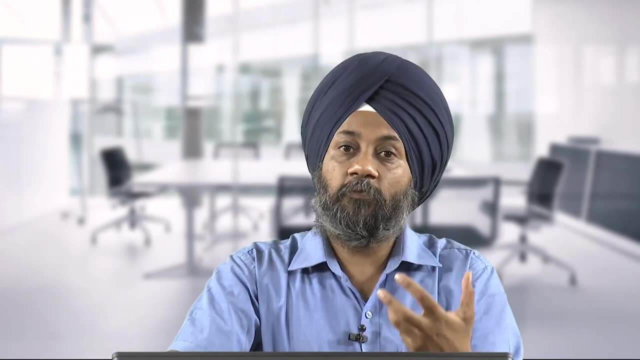 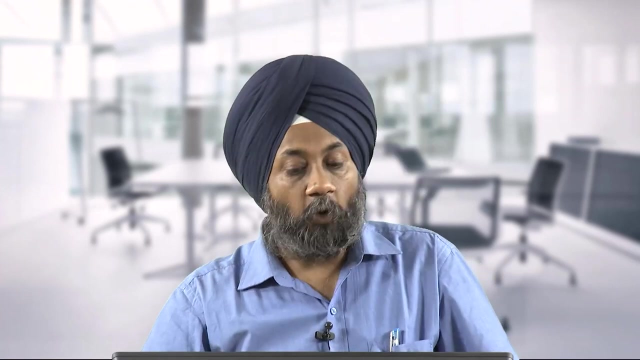 So MI or the material index will help us to select a particular material. So it is a kind of a ranking tool or the value which will help us decide that which material satisfies the needs and requirements, the functions of the application A or the product A. So 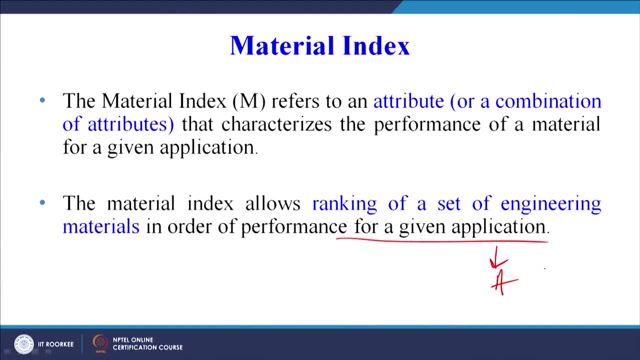 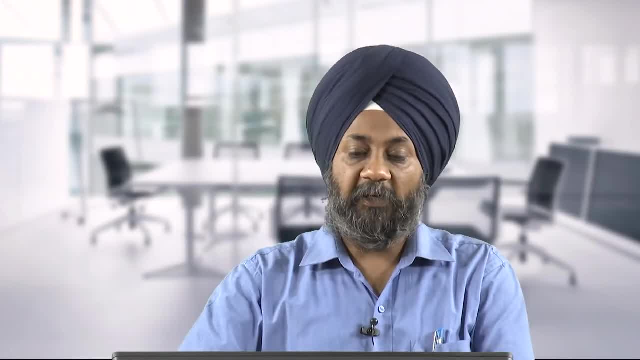 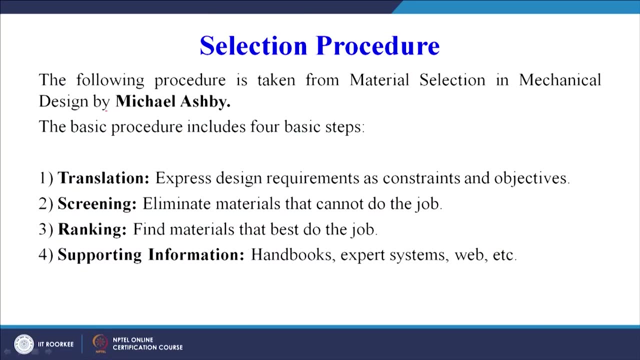 the material index allows ranking of a set of engineering materials in order of performance for a given application. So we can rank the materials based on the MI value. So the following procedure is taken from material selection in mechanical design. This is the source from where Michael Ashby, from where this discussion has been taken. 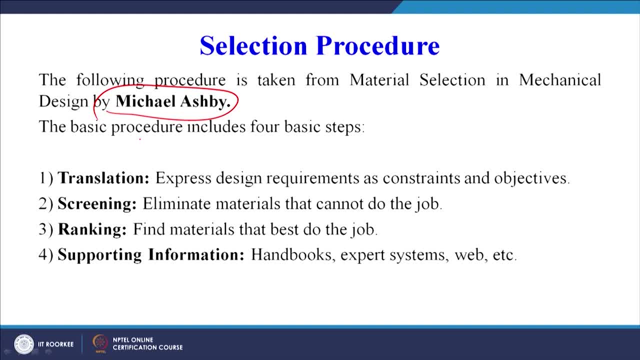 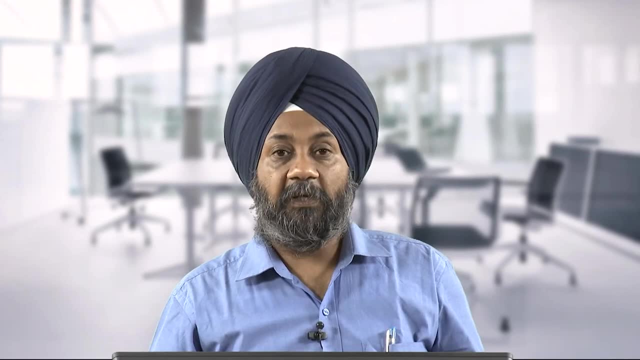 The basic procedure includes the 4 basic steps. First one is translation: express the design requirements as constraints and objectives. We will take an example. things will become more clear. So first one is translation. So first we have to design requirements. we have to write them in terms of constraints. 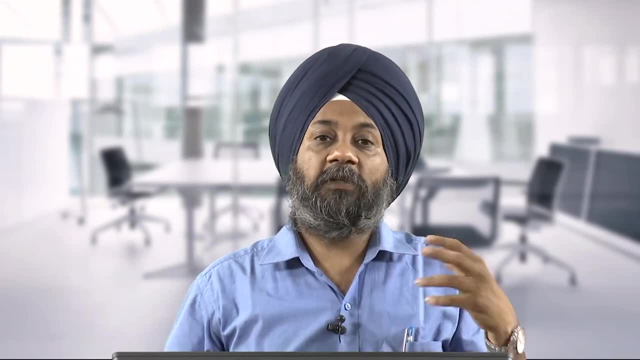 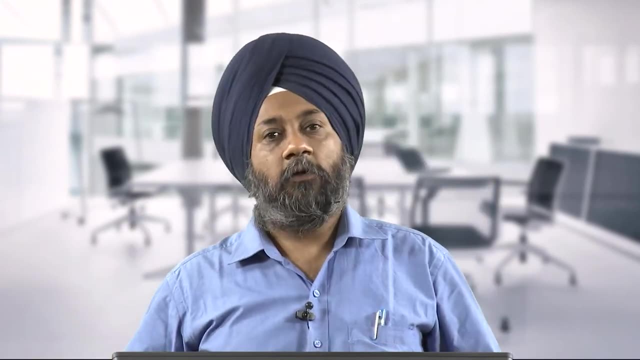 So this is the constraint of the design. So the one of the constraints can be that the height of this dies is fixed. You cannot change the height of the dies. It is the average height for all the speakers who are going to use this dies. 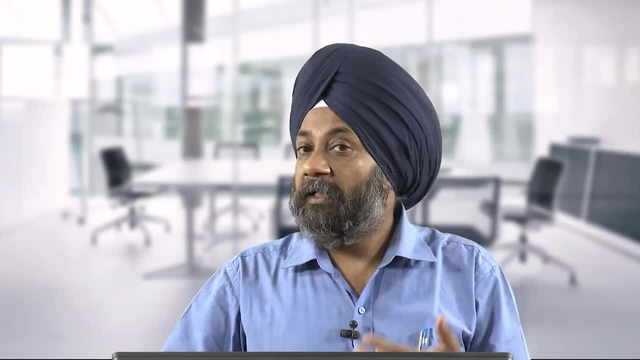 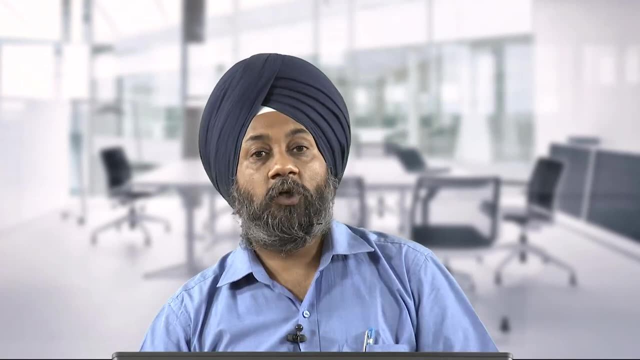 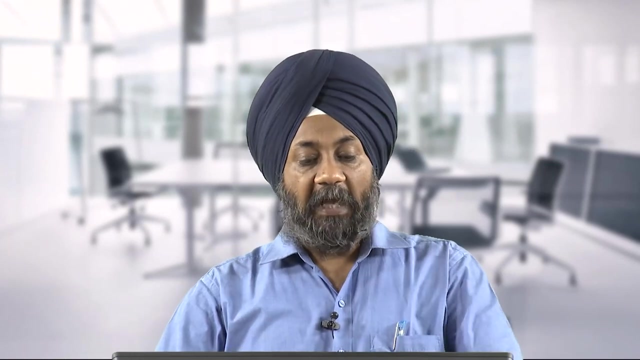 So the height becomes a constraint. So this is one design constraint which is already fixed. So express the design requirements as constraints, and then we have to list the objectives, that why this dies has to be designed. what is the objective for the dies? Screening, eliminate materials that cannot do the job. 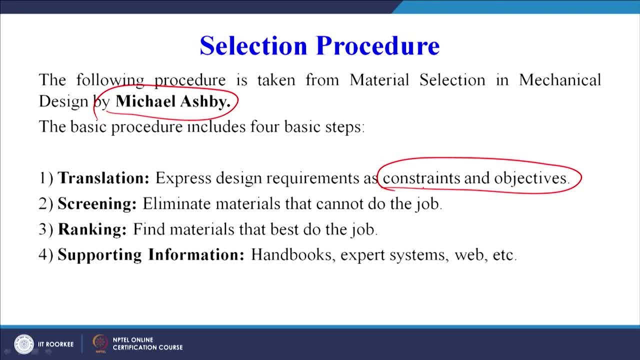 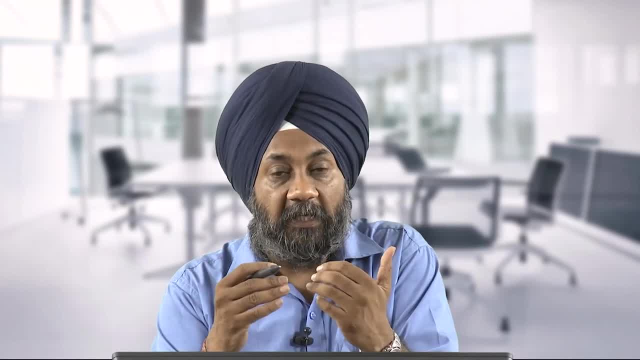 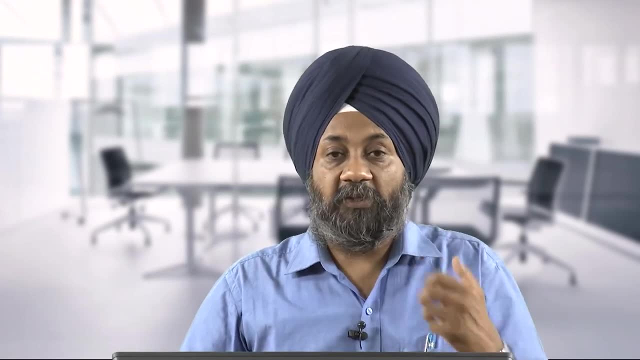 So then we start screening out the materials. For example, we have a constraint that the material that we are going to use, or the product that is being designed, has to sustain a temperature of 2000 degree centigrade. So this is a design requirement, which is a constraint: 2000 degree centigrade. 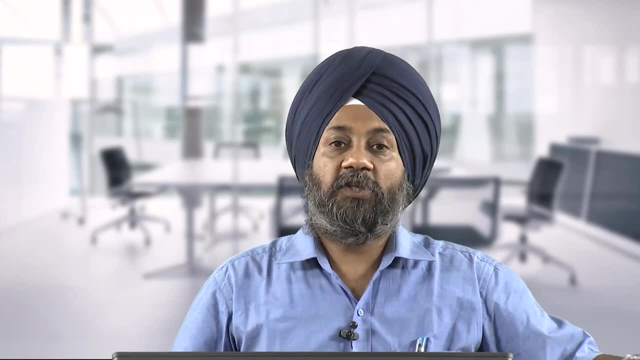 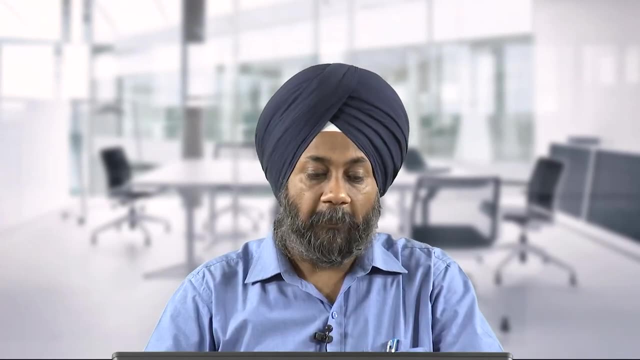 Then we can very easily screen out some materials which cannot sustain such a high temperature- 2000 degree centigrade. So some materials already gone. So that is the process of screening, Then ranking. suppose now we are left with 4 materials which can sustain the temperature. 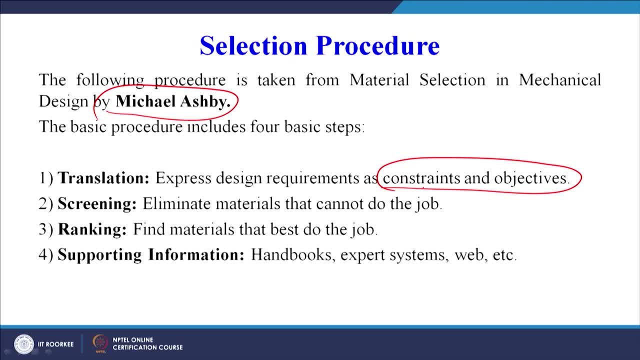 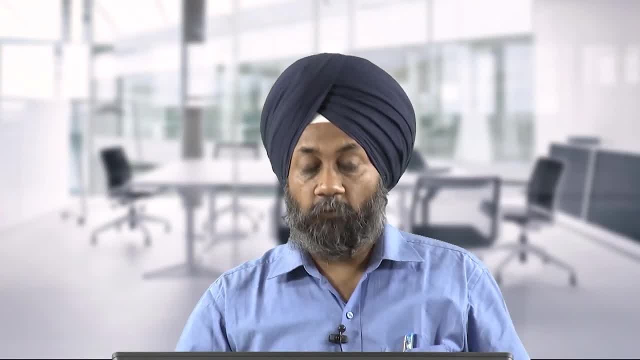 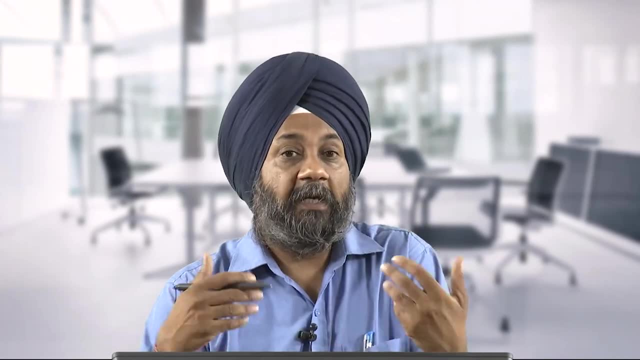 above 2000 degree centigrade. So then we will rank the materials based on certain other criteria. Then we will look for the supporting information from the handbooks or from the experts. there may be certain expert systems or the softwares available which may guide us regarding the 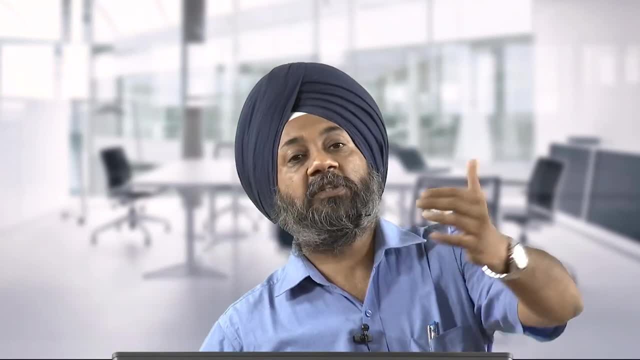 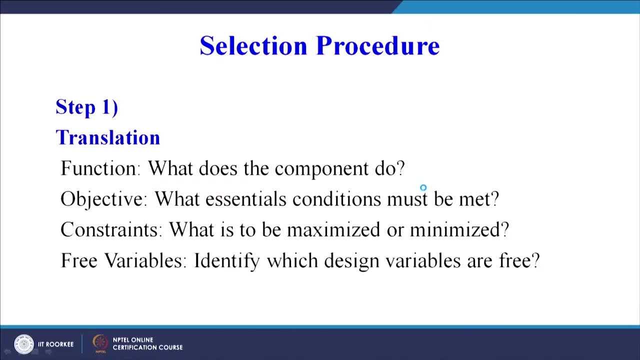 materials which are left. Some of the materials are already screened out based on the constraints and the objectives of the product design. Now the translation. let us quickly go through this process. translation first: we have to focus on function: what does the component do? Objective: what essential conditions must be met? 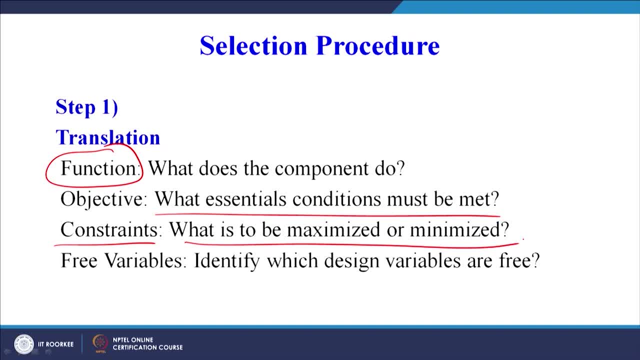 Constraints, what is to be maximized or minimized? As I have already told, the maximum temperature may be one of the constraint. Free variables identify which design variables are free. So for this design of this die. so the height, suppose, is fixed, but the cross sectional area. 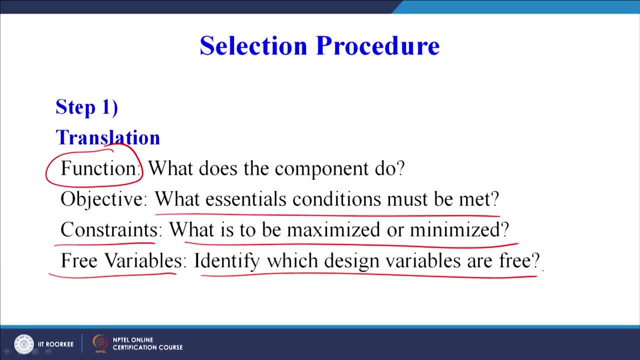 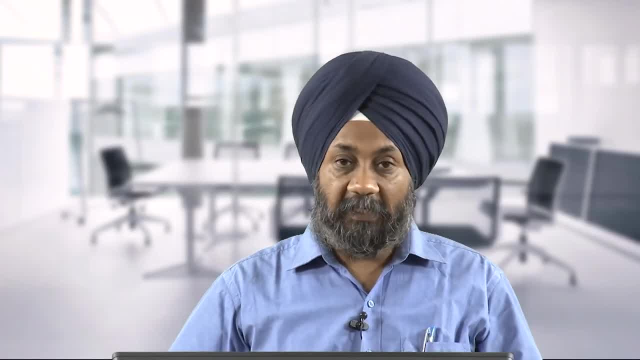 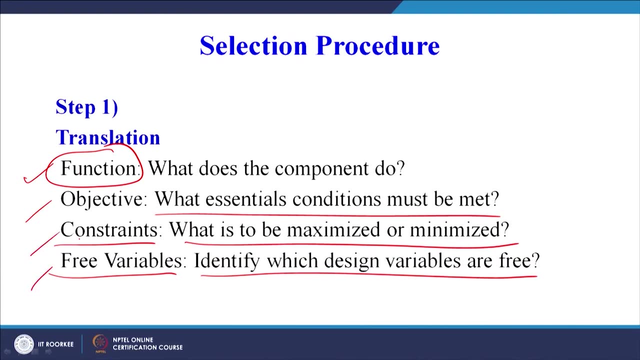 of this stand may be one of the free variable. I can choose the cross sectional area of the stand, So that may be a free variable in the design of this dies. So what is first is the translation of our design into function of design, Objectives, constraints and free variables. 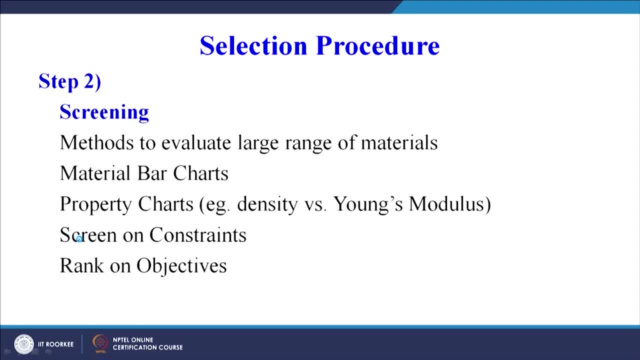 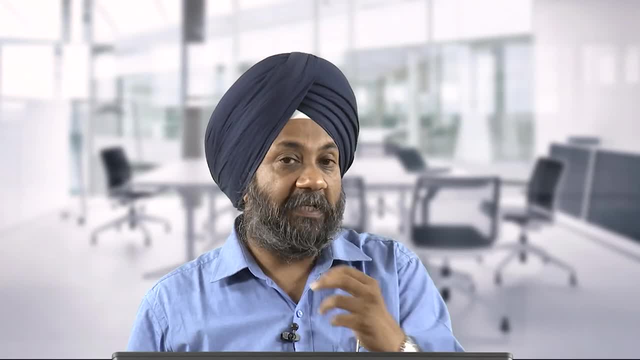 Then we do the screening. we need to develop methods to evaluate large range of materials. We can use the material bar charts and see which are the materials which are satisfying our requirements- Property charts, as we have seen in one of our previous session, towards the end of the 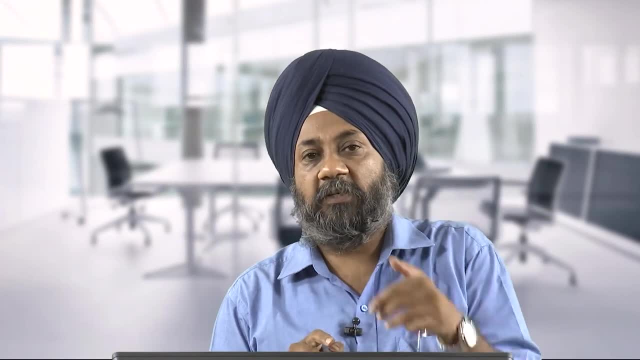 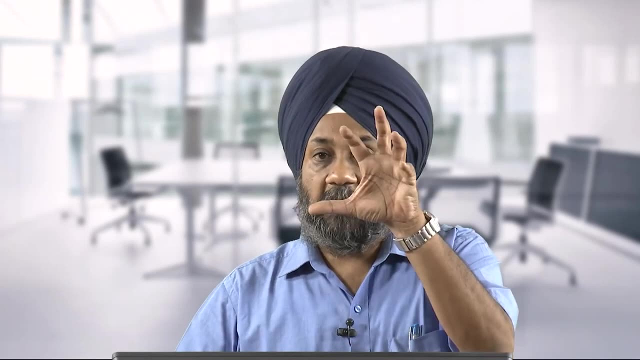 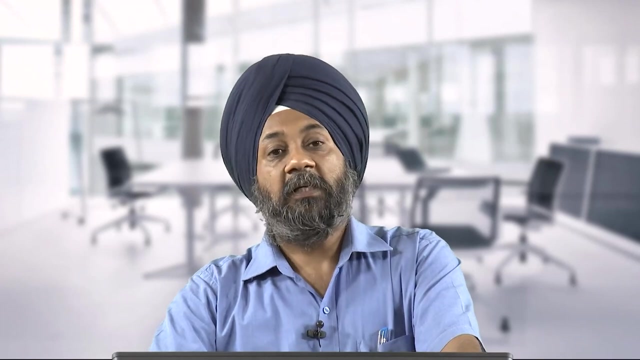 lecture I have shown a property chart which was showing that in soil strength, flexural strength, compressive strength, modulus, certain physical properties in terms of melting point, etc. So those type of charts are available. we can refer to those charts and screen out some of the materials which are not satisfying our constraints or not satisfying our objectives. 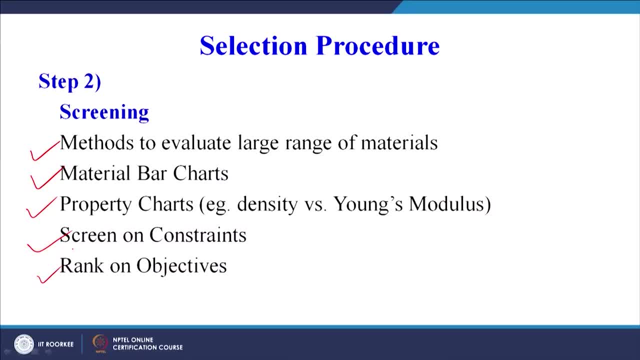 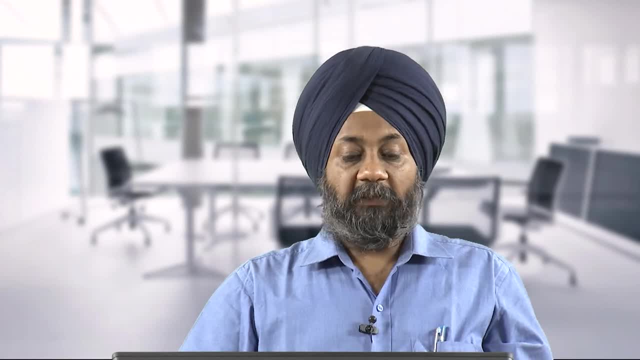 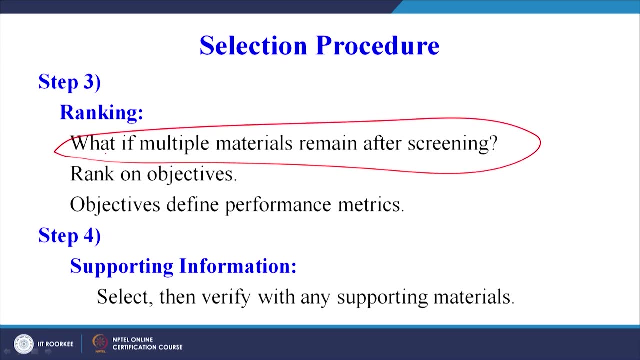 Then screen on the constraints and then rank on the objectives. So based on the objectives, we can rank the materials into the first rank, second rank, third rank, Then the ranking. so if, what if? multiple materials remain after screening very, very important. Now 3 materials are there. 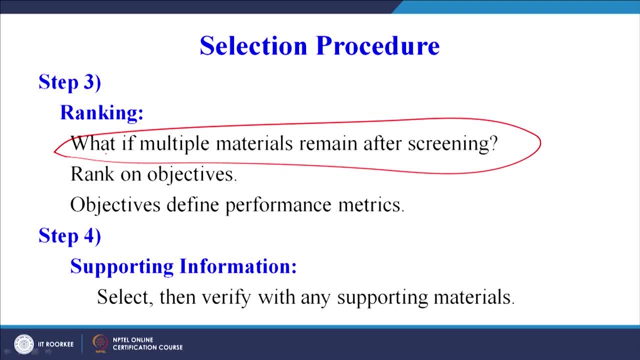 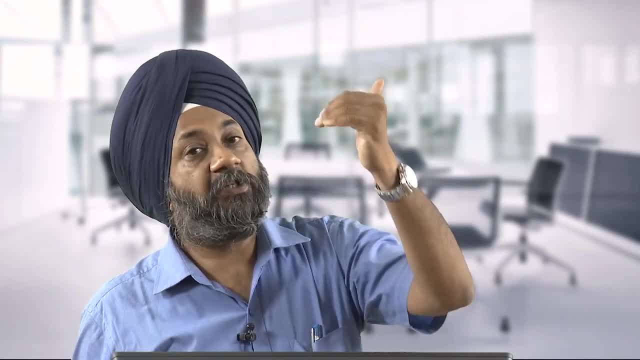 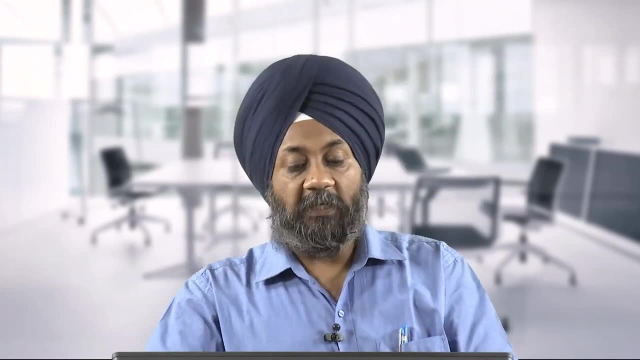 Which are left after screening. then we can rank on the objectives that, depending upon the objectives of the product, we can rank these materials that this is the material which is satisfying the objectives more closely as compared to the other materials. So objectives will define the performance matrix. 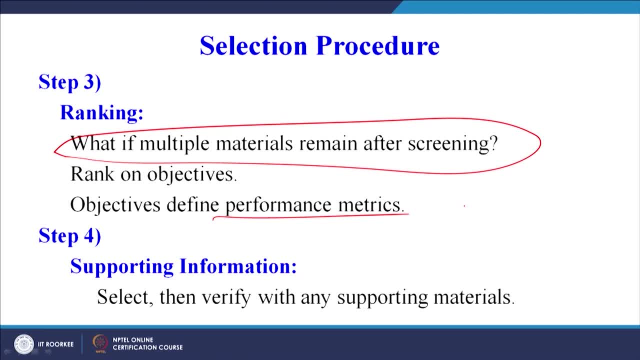 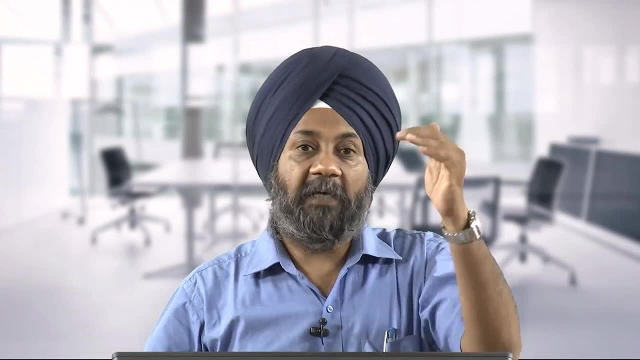 So there will be certain performance matrix for the product, which can be in terms of: for example, we are designing a new engine, So the efficiency of the engine Can be one of the performance matrix. and, depending upon the 3 materials that are left after the screening of the other materials, we will rank them that which material is going. 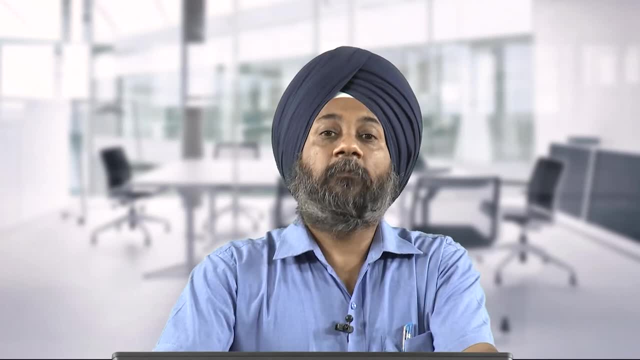 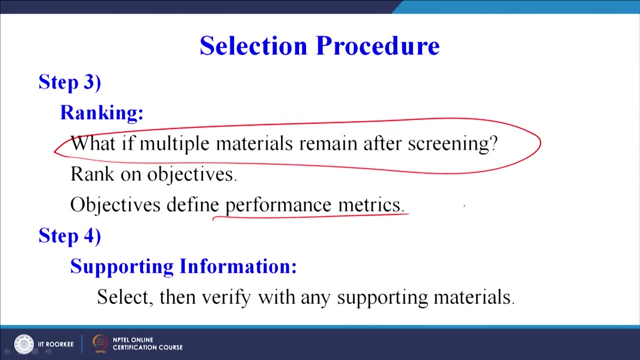 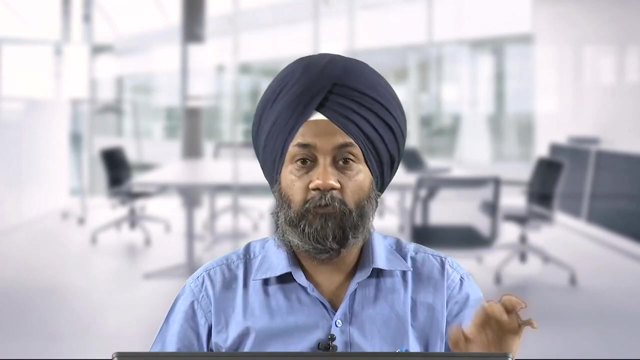 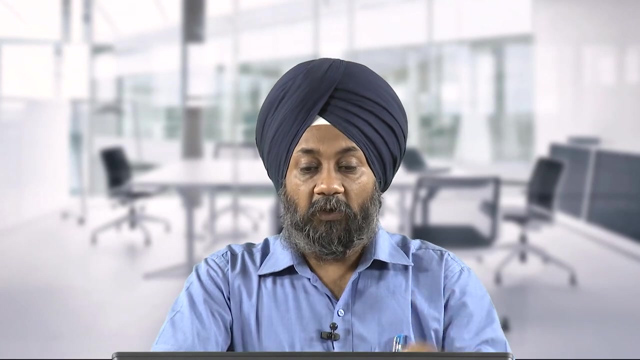 to affect the performance matrix in a more positive manner. Then, supporting information we will try to derive from the experts, from the books, from the handbooks, from discussion with the experts or the knowledgeable people in that specific engineering domain, So they will help us to take a decision regarding the choice of the material. 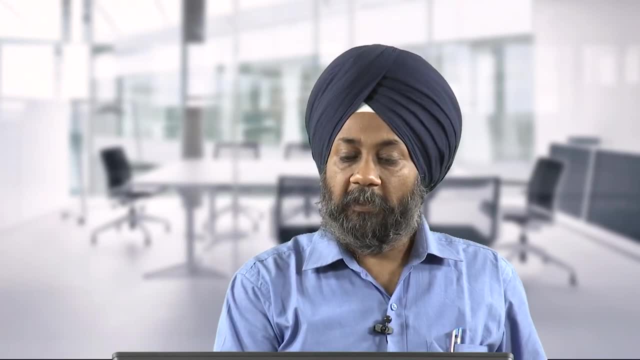 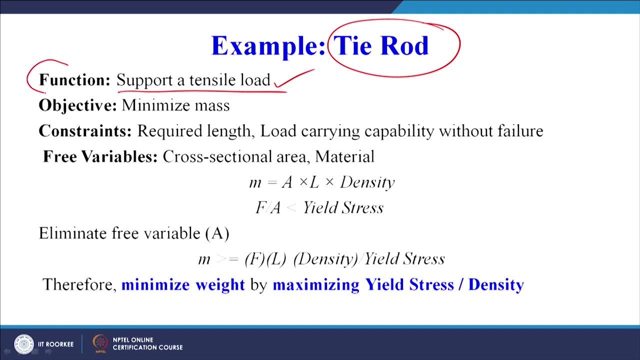 Now let us take an example of a tie rod. we have to design a tie rod, So the function is to support a tensile load. we must know the function. What is the objective of our material selection? we have to minimize the mass. What are the constraints? the constraint is: the required length is already fixed. 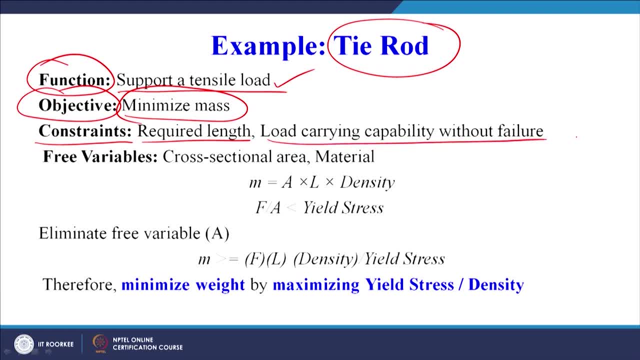 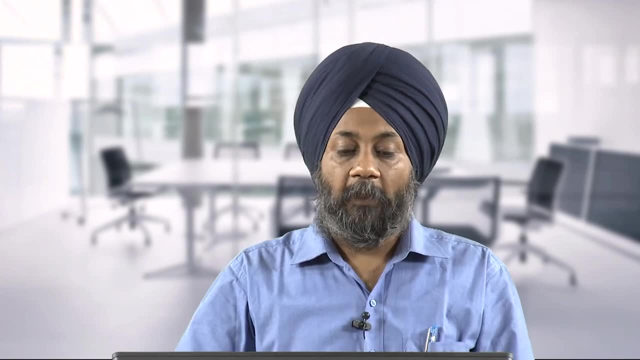 So L is already fixed. So load carrying capability without failure, that is also a constraint. So we have to support a tensile load, So it must not fail under that tensile load. that is also a constraint. the length is also a constraint. objective is to minimize the mass of this tensile, sorry, mass of this tie. 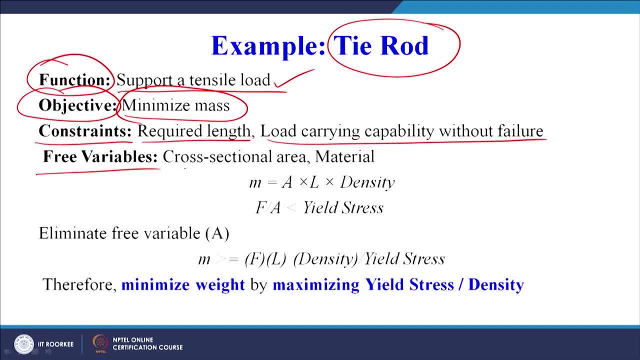 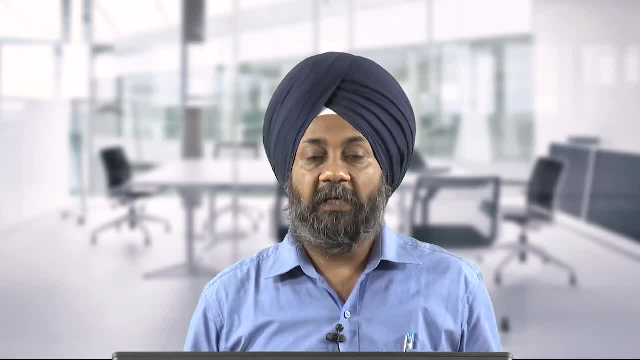 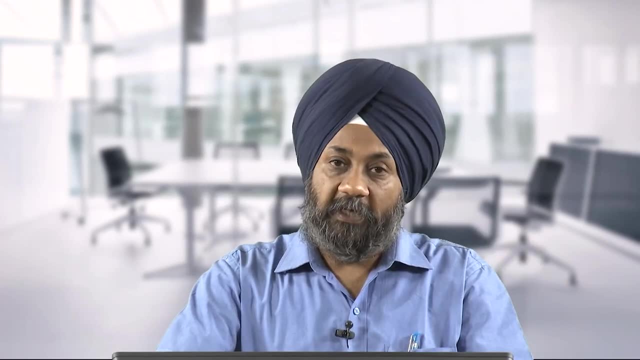 rod. So the free variable in this case is, as I have taken the example of this dies, design of the dies. suppose the height is a constraint here. the cross sectional area of the stand can be a free variable. Okay, Thank you, So that we can design as per our requirement or to satisfy the objective. 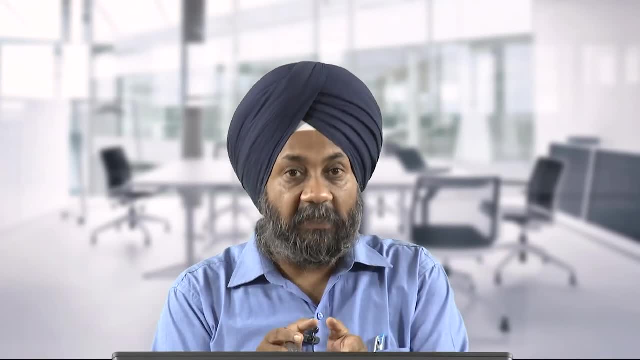 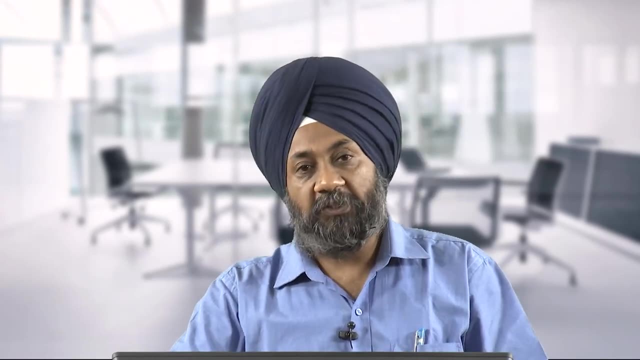 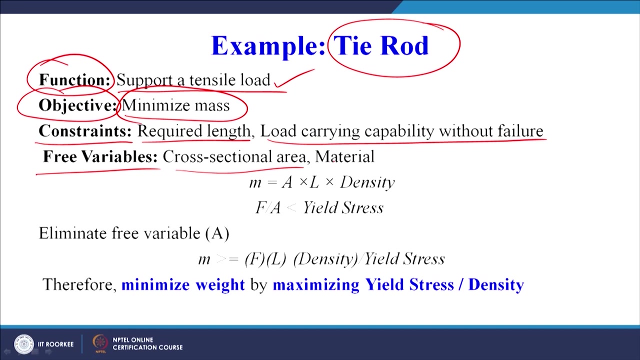 So the objective in this case will be different. wherever in our example that we have taken of a tie rod, the objective is very, very clear. that is, we have to minimize the mass of this tie rod. So the cross sectional area of the material is given by A, So we will see that the mass 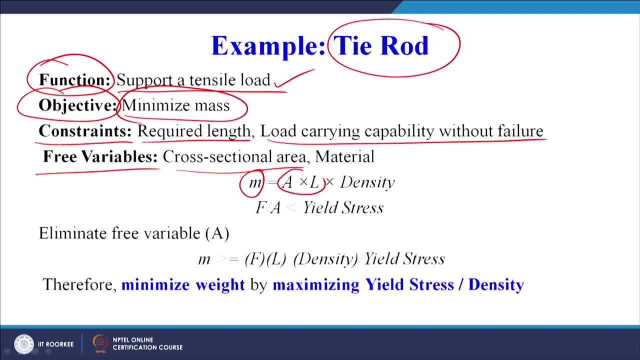 is given by the volume A x L. Okay, L is the cross sectional area, L is the length, so volume x, density, and F by A is the force per unit area that is being given by the yield stress. So we have to eliminate this free variable A. we have to design or we have to select a. 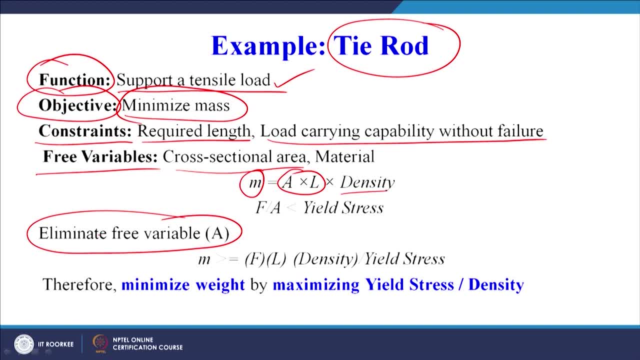 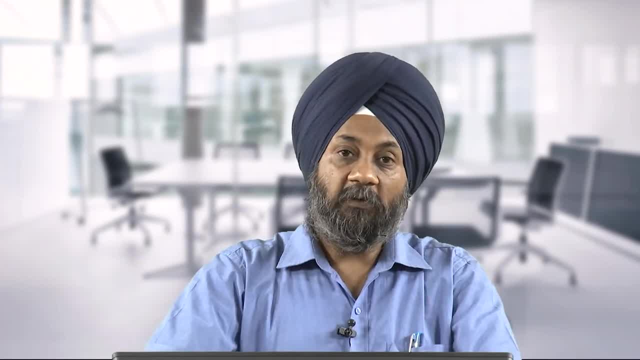 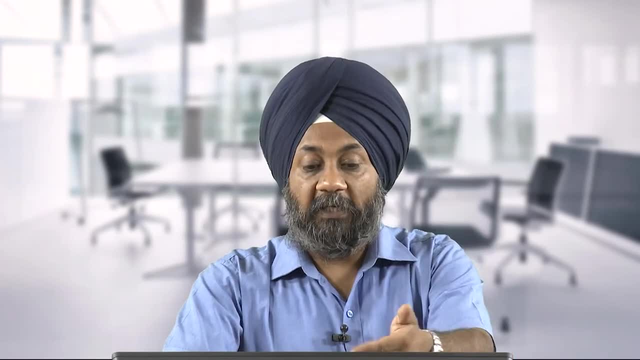 material for the cross sectional area. we have to decide the cross sectional area. length is fixed. We have to minimize the mass of this tie rod. that is our objective, so we can see that what can be the cross sectional area? So the cross sectional area which minimizes our mass without affecting our load carrying. 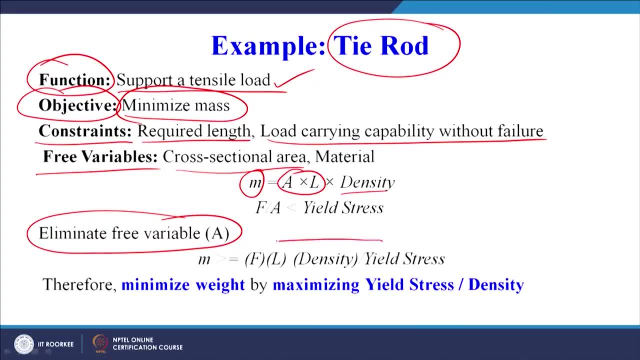 capacity without failure. So this equation will help us to fix or select our material. So here we see. density by yield stress is a parameter which can help us to decide a material. So therefore, if we have to minimize the weight, we can do it by maximizing the ratio of yield. 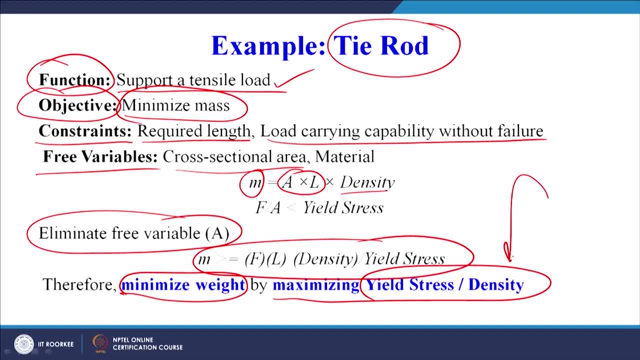 stress to density. So we have to focus now on this equation of yield stress. not the equation, but the ratio, the yield stress to density. Now suppose we have 4 different materials available with us. we will see the yield stress for the material and the density of the material and wherever we get this maximum ratio of yield. 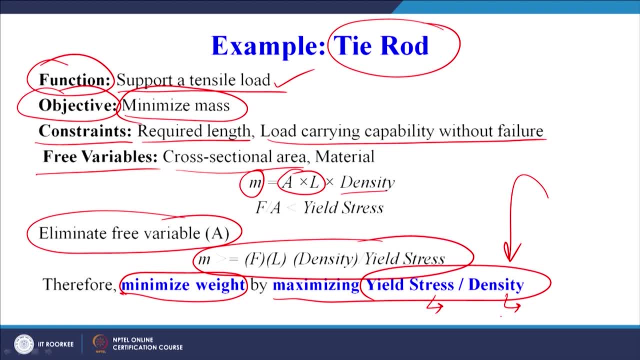 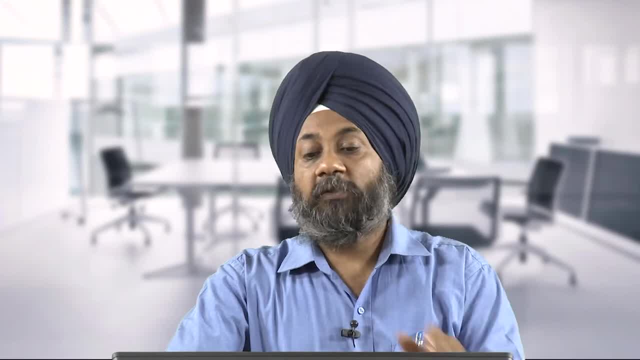 stress to density, or for the material for which we get the maximum ratio for yield: stress to density. that material we will select for our application. Okay, That is the tie rod in this case. So the 4 things are very important. what is the function, what is the objective, with which? 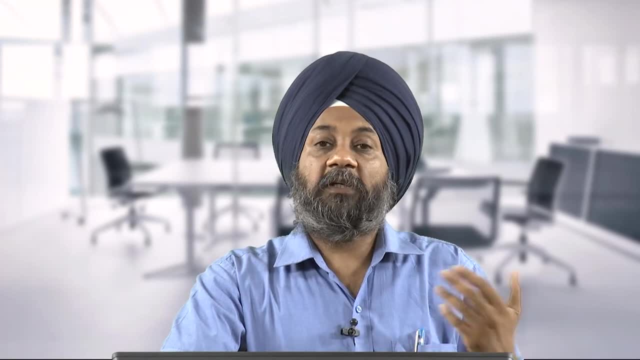 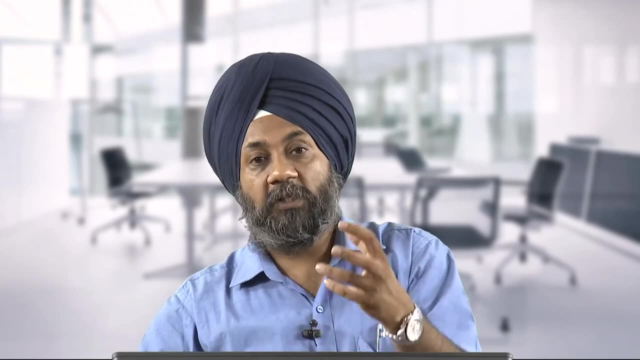 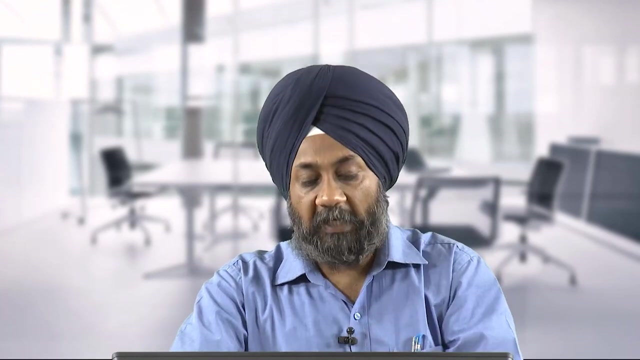 we want to select the material, what are the constraints and what are the free variables that have to be taken into account? Once that is ready, then simply we can try to fix up the material properties or the material index, which will help us to select the or rank the engineering material for that particular. 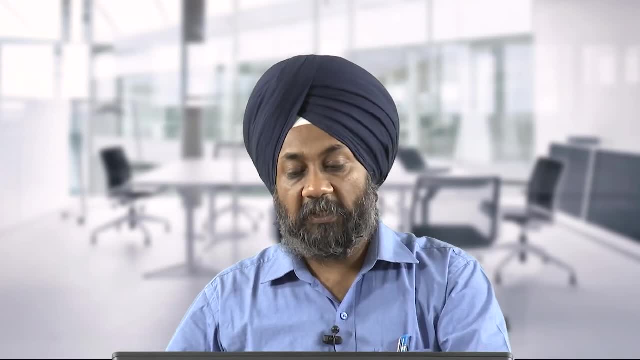 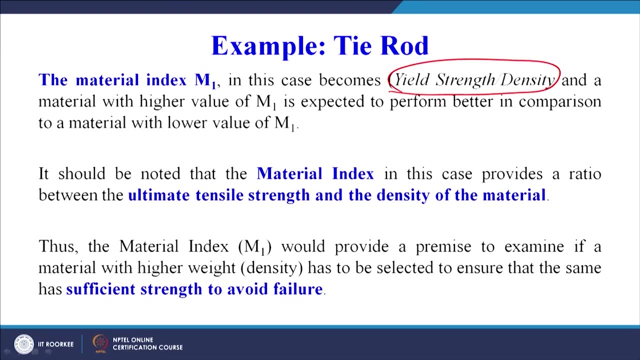 application. The material index m1 in this case becomes So the material index is yield stress by density, and a material with higher value of m1 is expected to perform better in comparison to a material with lower value of m1. that we need to maximize. 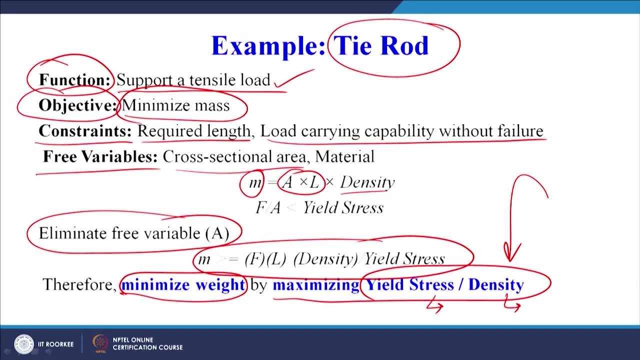 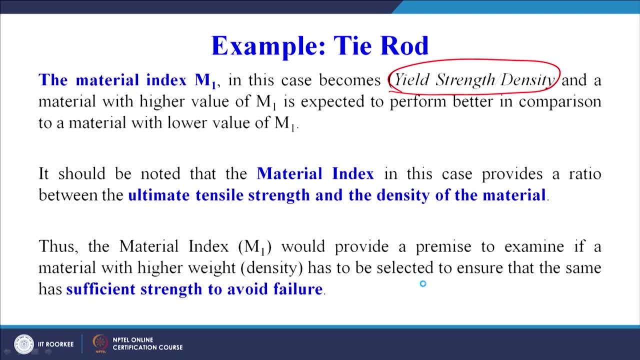 as we have seen in our previous slide, also yield stress by density. So the yield strength by density is. stress by density is an important material index which will help us to rank the various materials which are left after the scale, Okay, Which are left after the screening process. 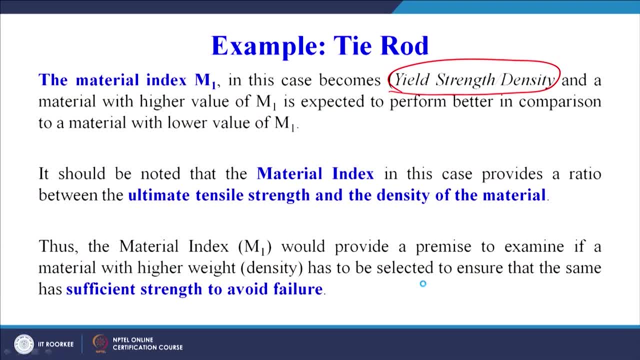 So it should be noted that a material index in this case provides a ratio between the ultimate and size strength and the density of the material. Thus, the material index would provide a premise to examine if a material with higher weight has to be selected to ensure that the same has sufficient strength to avoid failure. 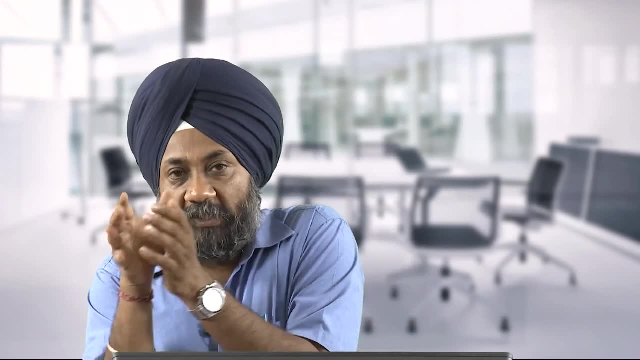 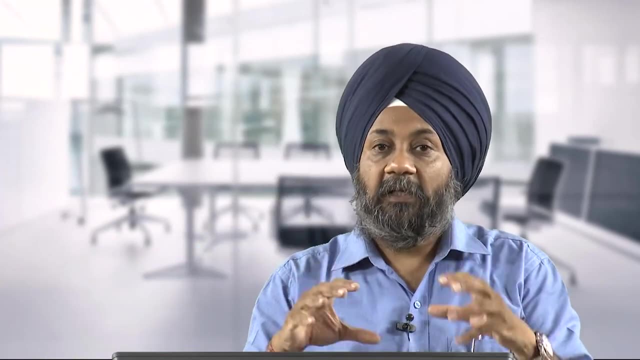 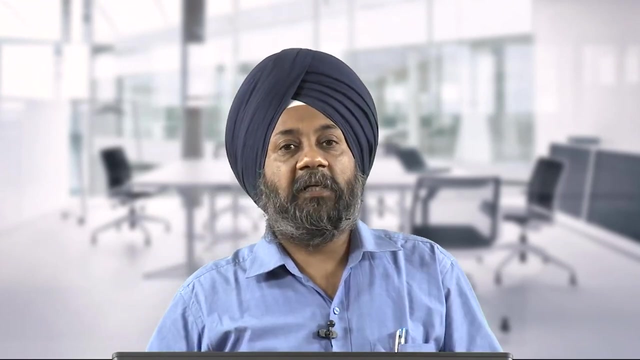 So here we will see that if the weight is more, whether it has the strength or a correlation between the density and the resistance to failure, Okay, The weight to failure under the tensile load becomes a important parameter, or a important guiding parameter for selecting a material with an overall objective of minimizing the 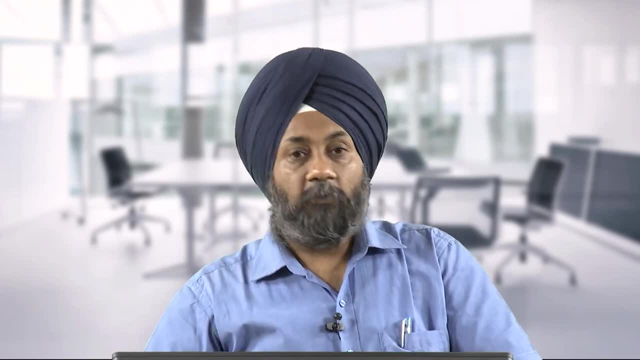 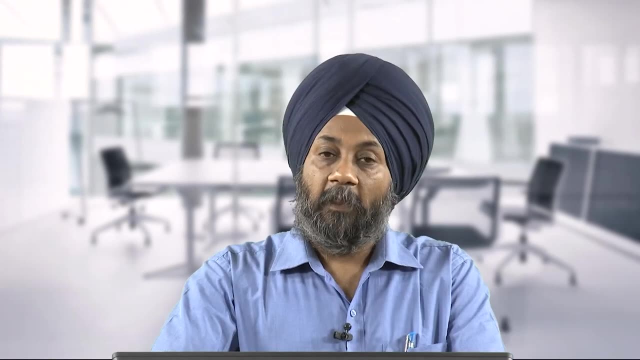 mass of the tie rod. So with this we come to the end for today's session. In our last session in this particular week, that is, week number 2, we will focus on the important engineering materials And we will try to see that. What are the?